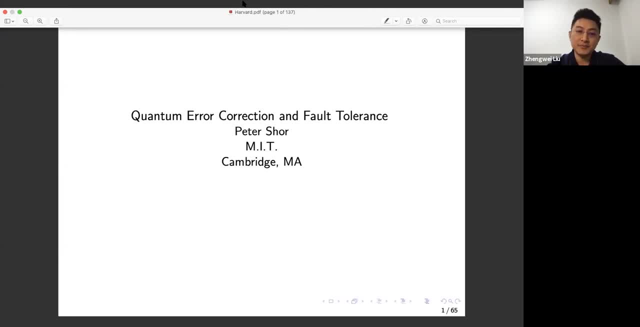 than the best known algorithm running on classical computing, And he constructed the first quantum error correcting codes showing the possibility of fault-tolerant quantum computation. Peter was awarded many international prizes, including Navelina Prize, Goddard Prize, Dirac Prize. 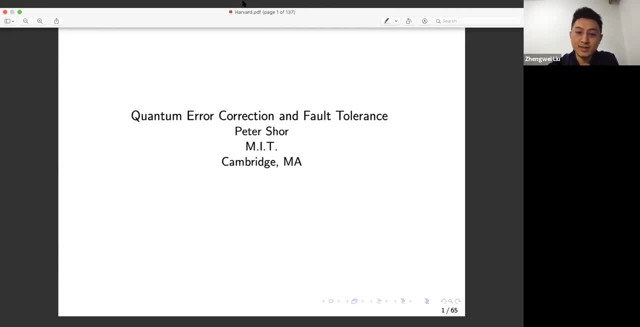 and several others. Well, today it's really great that we have Peter here to give us a talk on quantum error correcting and fault-tolerance. So, Peter, please, Okay, thank you very much for the introduction And I should say that I'm not going to say very. 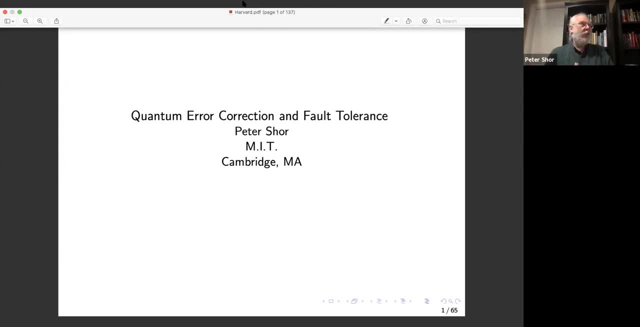 much about history in this talk, although I'll say a little bit. But coming up there is this 46th conference, which is the 40th anniversary of the MIT Endicott House Conference, where I guess Feynman gave his keynote address on quantum computation, And it was a conference. 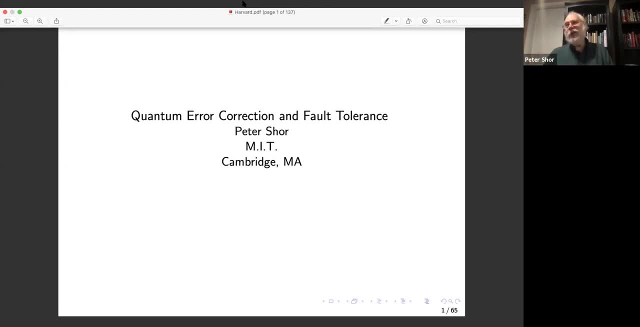 on physics and computation And there is going to be a 40th anniversary conference And I'm giving a keynote address there which is all about history. So if you want to know about the history of the subject, you can listen to that. 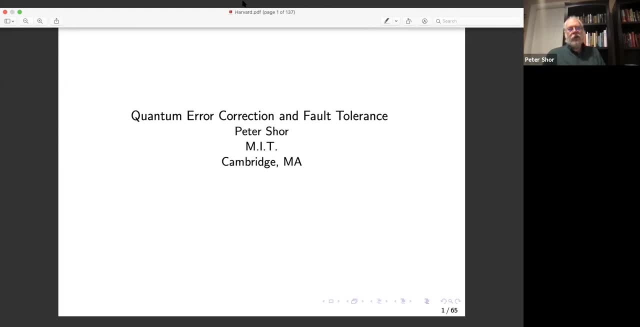 Okay, So I'm going to be talking about quantum error correction and fault-tolerance. Okay, Something is There, we go. So when I first discovered the quantum factoring algorithm, there was one reaction, And I guess Rolf Landauer, who was a physicist at BM. 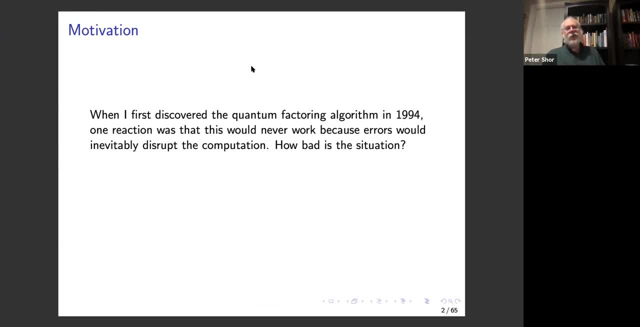 is probably the strongest proponent of this reaction, And the reaction was: this is never going to work because errors are going to inevitably disrupt the computation. So why did he think this? And how bad is the situation? Well, if you want to do 10 to the 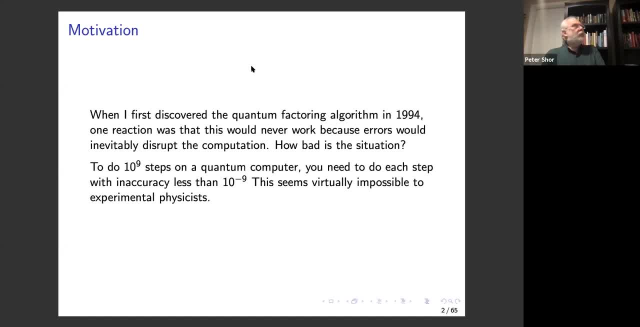 ninth steps on a quantum computer and you don't do any kind of error correction. you need to do each step with inaccuracy less than 10 to the minus ninth. Now, 10 to the ninth steps is not that long for you know if you want to factor a large number And doing it. 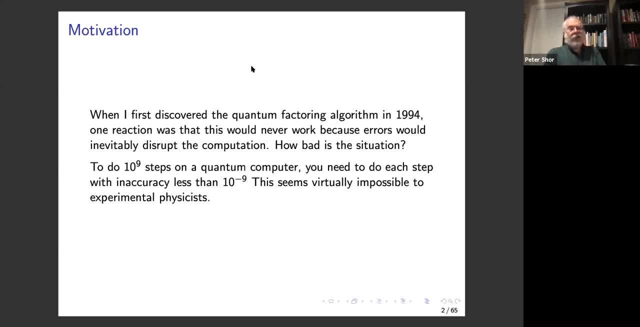 each step is less than 10 to the minus ninth, And if you want to factor a large number step with inaccuracy- less than 10 to the minus 9th is basically absolutely impossible. At least experimental physicists now think it's absolutely impossible. So you can ask: is there some way of? 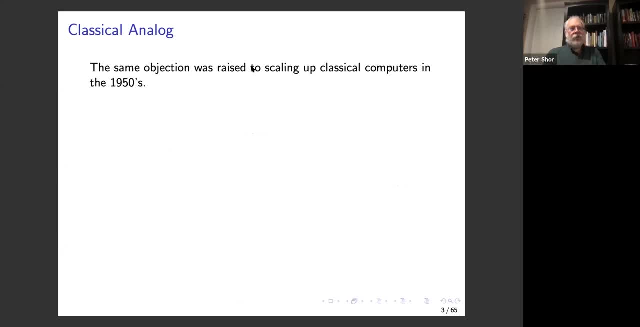 doing quantum error correction. Well, if you look back in history, the same objection was raised to scaling up classical computers in the 1950s And people said that vacuum tubes will never be accurate enough to do long computations. Vacuum tubes are always breaking and failing and 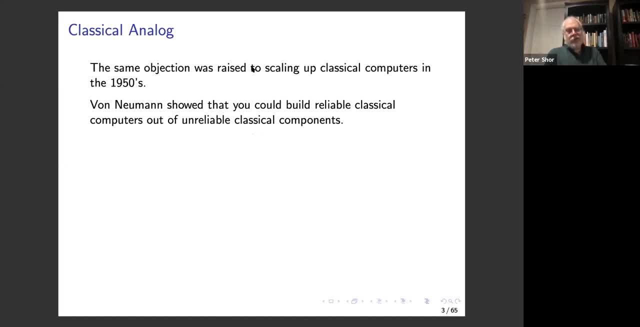 giving the wrong answer. So von Neumann, in response to this, showed that you could build reliable classical computers out of unreliable classical components. And then he speculated that the brain did something of the kind. So we can look back and ask: well, can you use these? 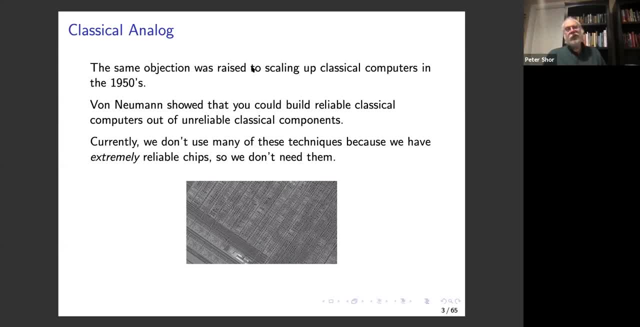 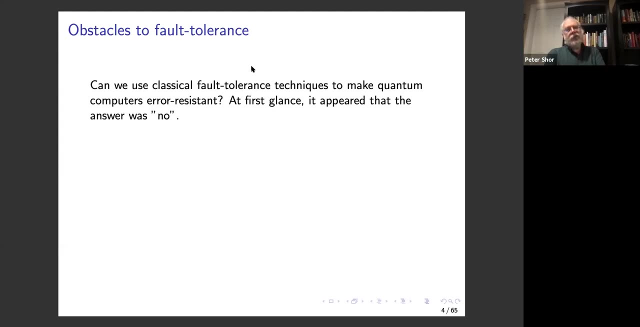 techniques For quantum computation. So currently we don't actually use many of these techniques because we have extremely reliable computer chips, So we don't need them. But we could if we had to. So at first glance it looked like the answer to whether you could use classical fault-tolerant. 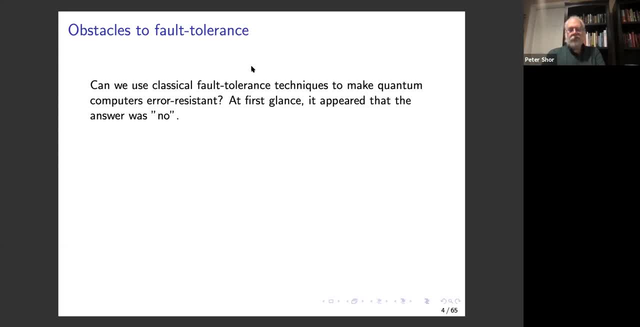 techniques for quantum computers was no, Why not? Well, there's this thing called the no-cloning theorem, which says you cannot duplicate an unknown quantum state. There's this thing called the Heisenberg Uncertain Principle, which, well, one aspect of it says that. 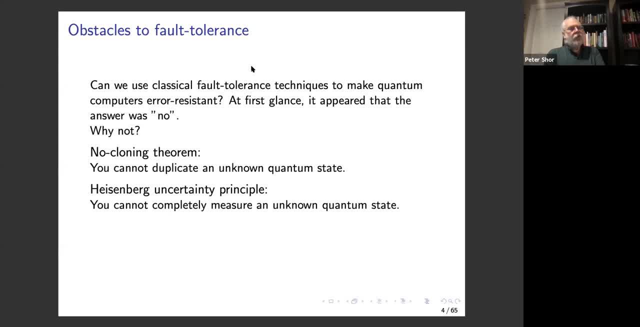 you cannot completely measure an unknown quantum state. So if you have a quantum state, I mean so that's a definite state with lots of accuracy. If you have a one-qubit quantum state, you can only get one bit out of it, even though it takes three real numbers to specify it. So that's the Heisenberg. 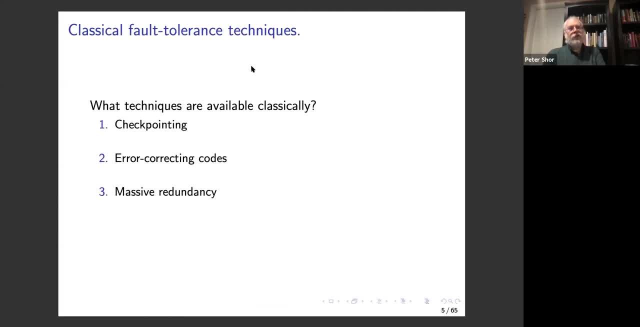 Uncertain Principle. So let's look at the classical fault-tolerant techniques, So the ones that are really useful and not just minor patches, are checkpointing, error-correcting codes and massive redundancy. So checkpointing is: you start your quantum computer or start your classical computer and every so often you write. 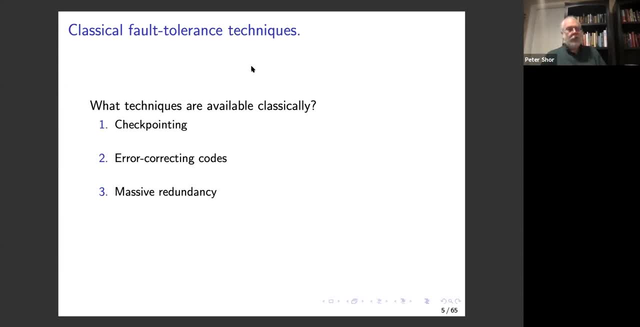 down the state of the classical computer And then if the computation goes off the rails after the most recent checkpoint. Now can you do that? No, Because taking the state of the quantum computer and writing it down is cloning, So that's impossible. Now, error-correcting codes. So 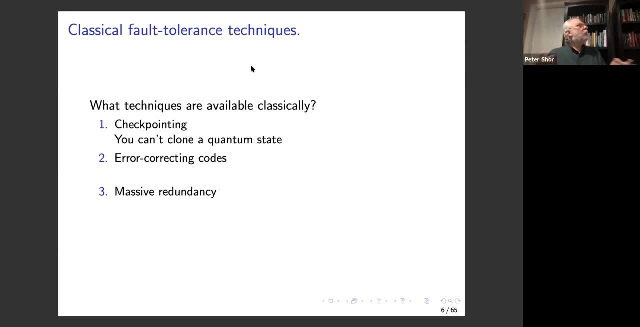 error-correcting codes. you have, say, k bits, and then you add some number of parity-checked bits, which are, you know, Boolean combinations, In fact exclusive r's of the previous bits, and the whole thing is your error-correcting code. And now, if a few bits of your 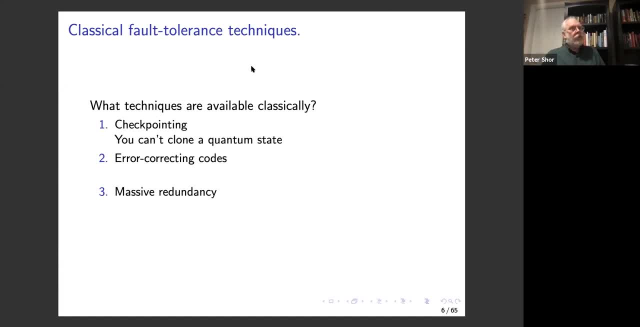 error-correcting code are wrong, you can correct them by looking at the parity-checked bits. And so that was a beautiful, classical idea. Can you do it in quantum computing? Well, at first sight it looks like it's cloning, because you're taking this bit and making parity-checked bits out of it. 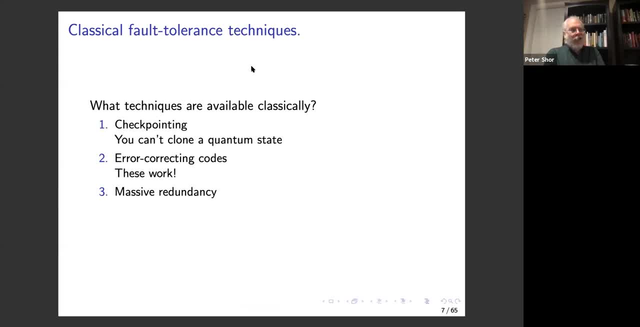 But no, it's not cloning. These actually work, And I'll explain why. The third thing is massive redundancy. You make many, many copies of every bit in your computer and you continually compare them against each other, And this is a thing that really works. 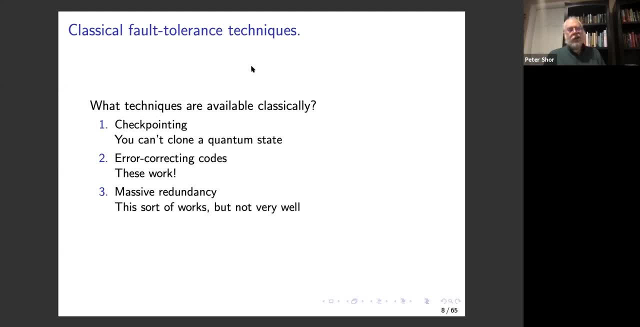 classically And it sort of works, but really not very well at all on a quantum computer. So error-correcting codes are what we have to use. So can people see this little cursor? Oh well, I will assume you can. 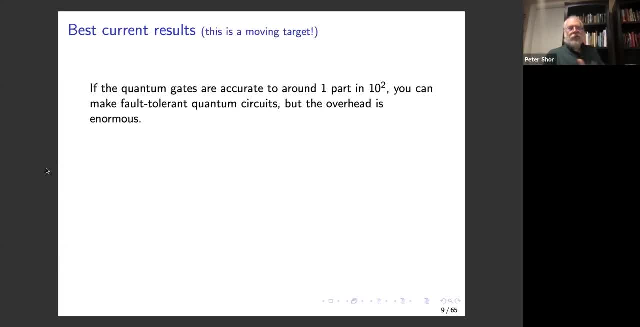 Anyway. so if the quantum computer? so the best current result is if the quantum computers are around accurate quantum gates are accurate to around 1 part in 10 squared 1 in 100, you can make fault-tolerant quantum circuits. But the overhead, although it's polynomial, is absolutely. 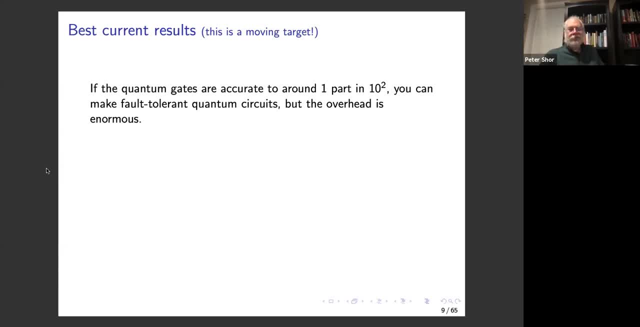 phenomenal. You would never actually want to do this. If your gates are accurate to 1 part and 10 to the fourth, you actually get much better overhead. It's still pretty big, but it's probably workable. I mean you might, instead of having 1,000 bits, quantum bits need 100,000. 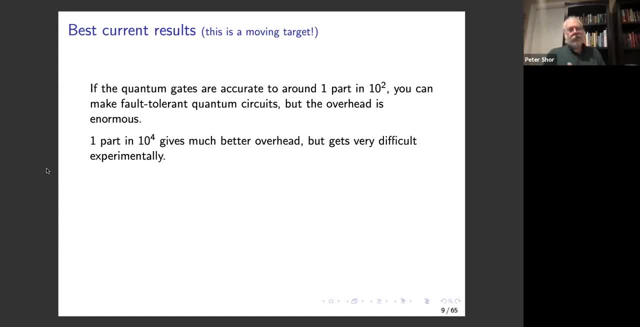 physical quantum bits to implement 1,000 logical bits. But this gets very difficult. I mean it's very difficult to get 1 part in 10 to the fourth gates experimentally. Right now they can do this if you just have two cubits and you're doing a gate between them. 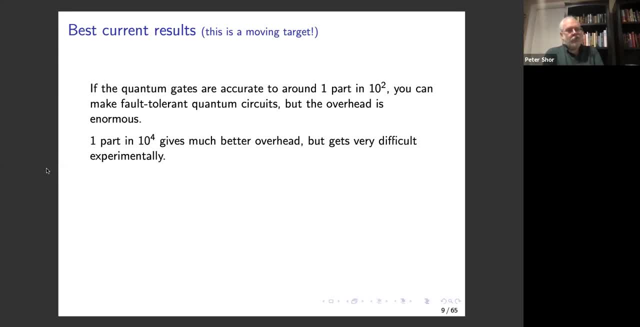 But suppose you have 100 cubits and you're doing a gate between them. I mean, we're going to have 100 cubit chips in the very near future but they're not going to be anywhere near 1 part in 10 to the fourth accuracy. And 100 cubits isn't anywhere near enough to do these fault-tolerant. 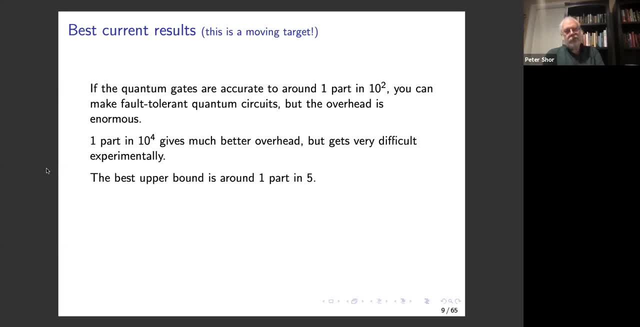 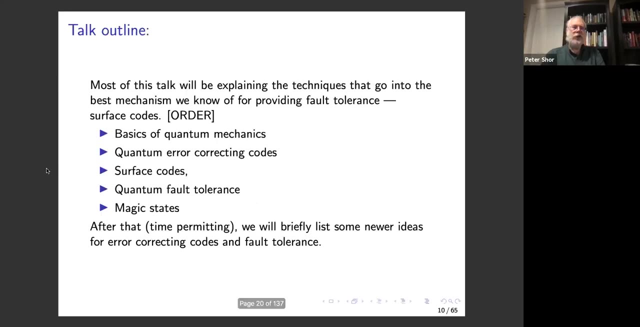 techniques anyway, And the best upper bound is 1 part in 5 or so And I should say one open-cubic question maybe is the right threshold. it's a very fuzzy, open question because the actual threshold depends very much on the architecture of your machine. so most of this talk will be 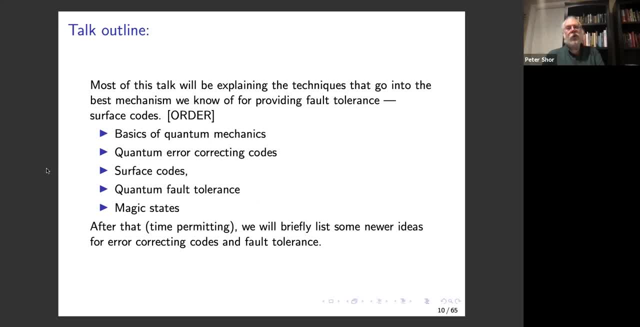 explaining the techniques that go into the best mechanism we know of for providing fault tolerance, which is, um the surface codes. and this order was to remind me to put these techniques in the right order. i had in my talk and i didn't do that. so, um, first we're going to do the basics of 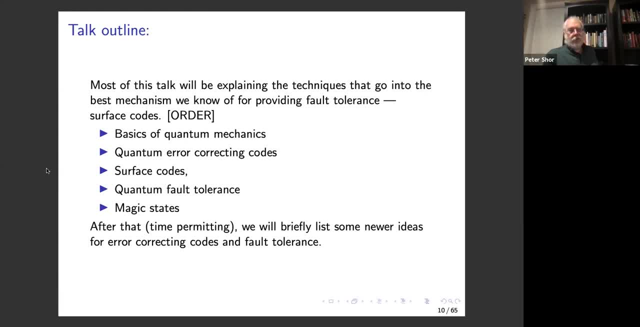 quantum error correcting codes, then we're doing quantum error, then we're doing surface codes- and yeah, this is the right order- quantum fault tolerance and then magic states, and after that, if we have any time left, i have two slides on some completely different ideas that might be useful for doing quantum error correction and computers. 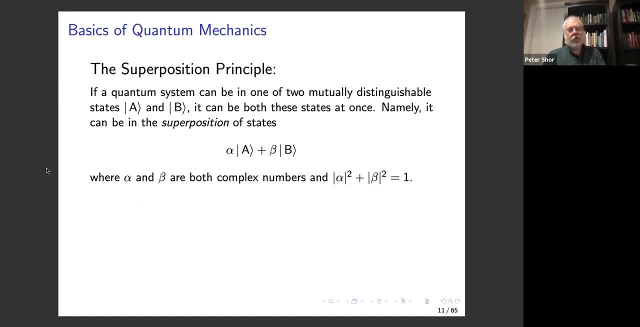 okay, so first let's go over the basics of quantum mechanics. so the superpositions principle, as physicists stated, is suppose a quantum computer system can be in one of two mutually distinguishable states, a and b, then it can be in both these states at once. so namely it can be in the superposition of states alpha a plus beta b. 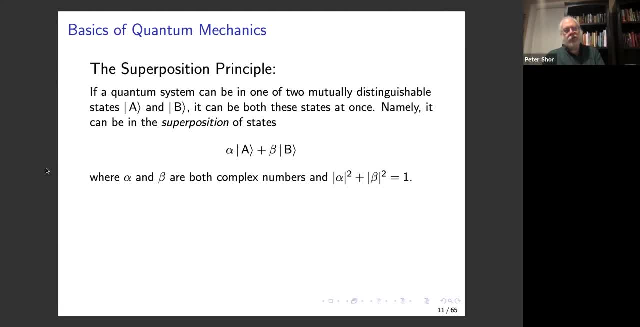 where alpha beta are both complex numbers and the sum of their squares of their magnitudes is one. okay, and you know this is. you know, schrodinger took the superposition principle and took it to, i guess ad absurdum, by um saying: well, suppose a is a live cat and b is a dead cat. 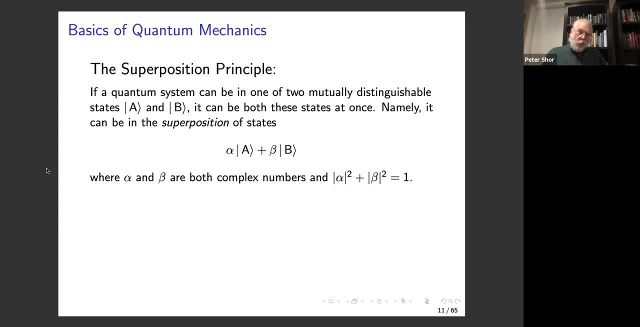 how can a system be in a safe position of um alpha times live cat plus beta times dead cat? and you know, you can argue philosophy, i mean, if you're a philosopher you can argue about whether such a superposition um can exist or not. or does it really meaningful to say a cat isn't a supervision? 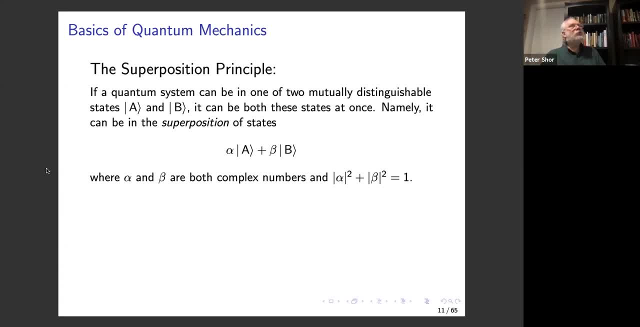 of live and dead. but you know, cats are much bigger than your qubits in a quantum computer, and so we will assume this holds for quantum computers and, as far as anybody knows, this is true of everything in the universe. so if you look at this system, remember we said these two. 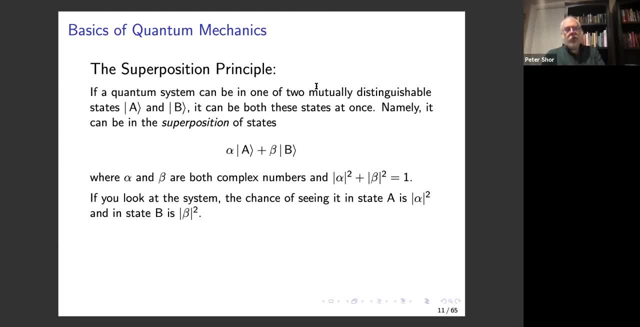 systems, state states, for mutual is distinguishable. so you use whatever experiment you have for distinguishing these two states. then the chance of seeing it in state a is absolute value of alpha squared and stance of seeing it in state b is absolute value of beta squared. so this is the 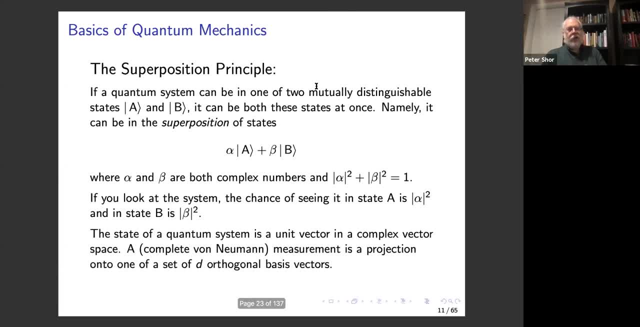 physics explanation of the superposition principle. the math explanation of the superposition principle as a state of the system is a unit vector in a complex vector space, or actually you can also say it's a vector and a projective vector space. it's the same. a complex projective vector space, it's the same thing, and a measurement. well, 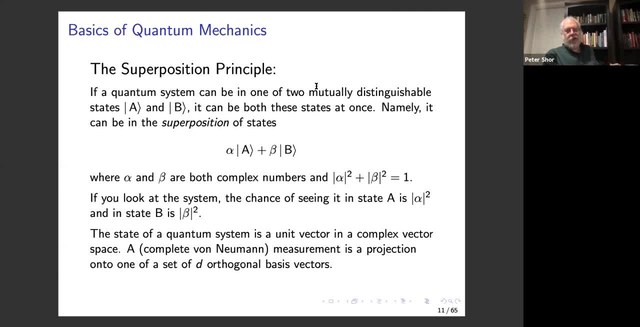 a complete von neumann measurement is a projection onto one of the set of d orthogonal basis vectors, and so two states are distinguished if they're orthogonal vectors. where orthogonal means you have a and you have b. they're distinguishable if um complex conjugate of a times dot product b is zero. 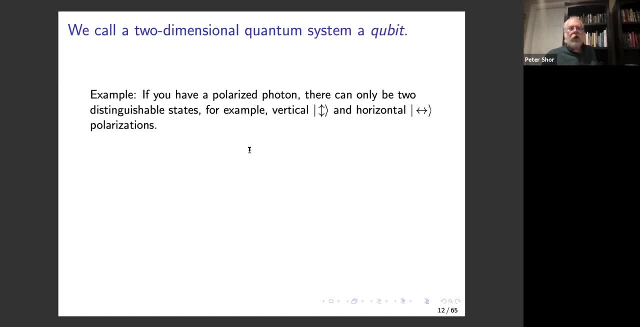 okay, so we're going to call a two-dimensional quantum state space, a qubit, and the example is: if you have a polarized photons, then there are only two distinguishable states and we have to choose a basis for that, and we can choose the basis vertical polarization and 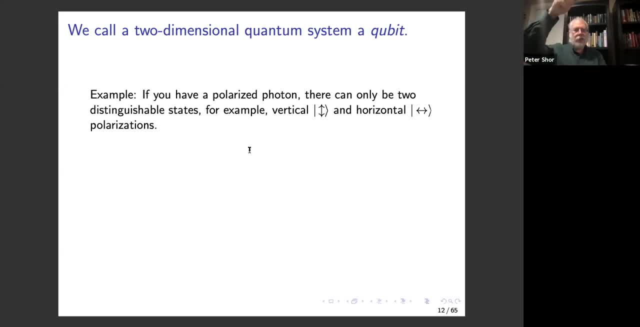 horizontal polarization. of course, we could rotate our polarizing filter at 45 degrees and choose right diagonal and left diagonal and any two. um any state of a polarization of a photon can be expressed in this basis, for example in this form: we know that the value of the 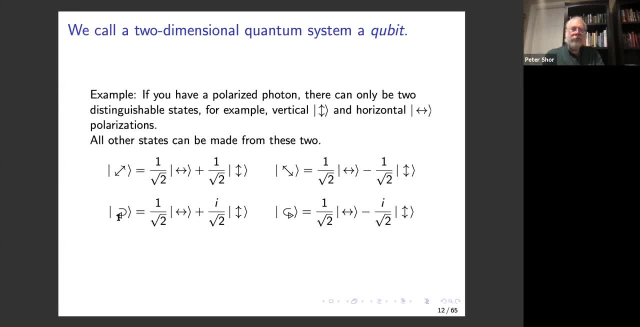 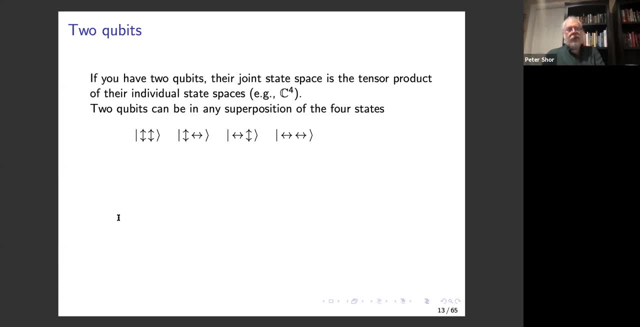 the 1 over the 5 is the totalBe mark 12. 3dSean's hol inversion Van bunch inch his going to the original state spaces and this means there is that will be the can be in any superposition of the four states. 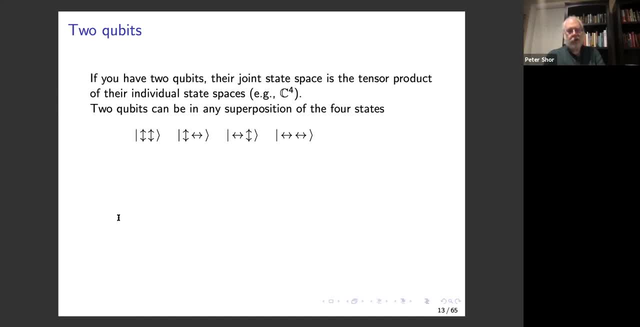 vertical, vertical, vertical horizontal, horizontal, vertical, horizontal, horizontal. And this includes completely non-intuitive states such as an EPR pair of photons where neither qubit alone has a definite state. So for an EPR pair. 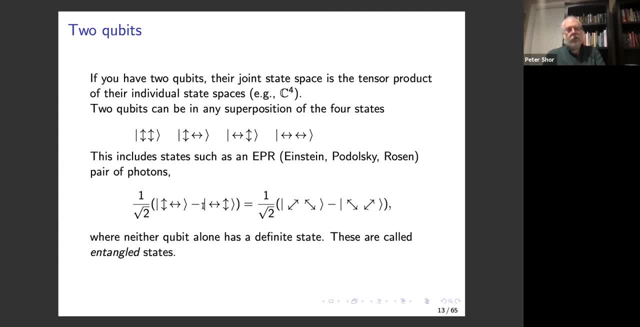 it's the superposition of vertical horizontal minus horizontal vertical, And if you write this in any basis, the two qubits will always be in opposite states, in orthogonal states. So these are called entangled states and they're one of the places. 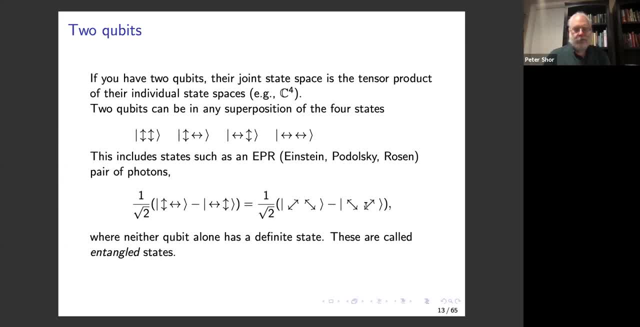 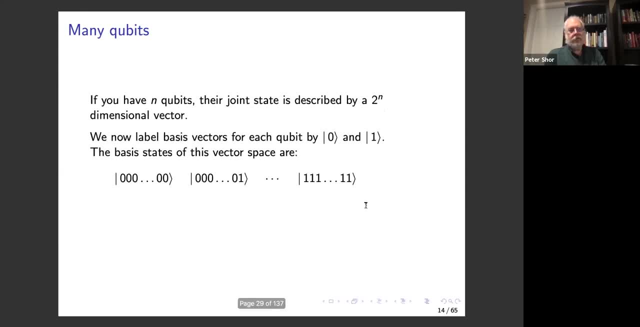 where quantum computation gets its power. So if you have n qubits, their joint state space is described by a two to the nth n-dimensional vector. And from now on we're not gonna be using horizontal and vertical, but zero and one. 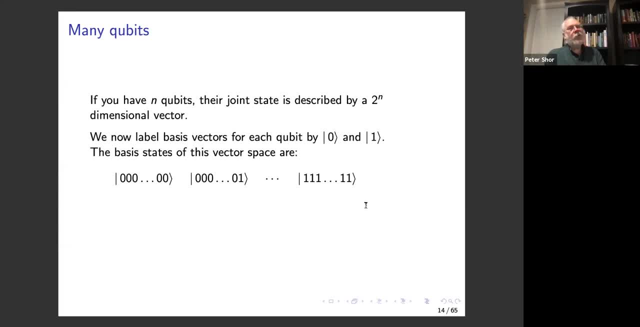 which you know if you're a computer scientist, it's much more comfortable to use zero and one. So the basis states of this vectors are n-bit binary strings, And the high dimensional reality of the space is another place where quantum computing obtains its power. 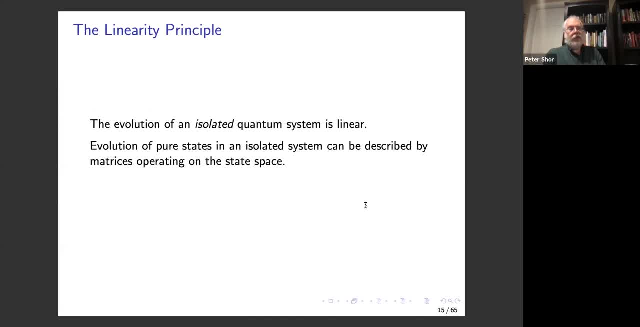 So the linearity principle says the evolution of an isolated quantum system is linear. The measurement operator is not linear. And again, you can have endless philosophical arguments over what exactly this means and physicists have, but let's not worry about that in this talk. 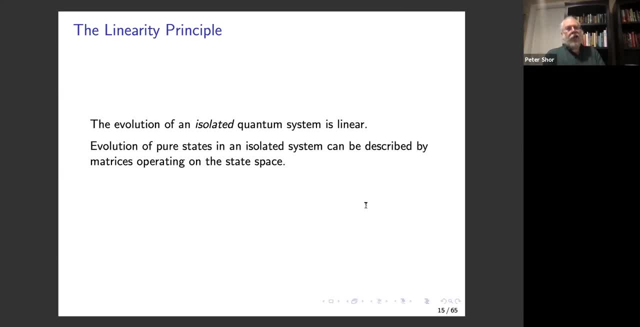 So the evolution of pure states in an isolated system is: we have a linear operator on a vector space. It's just a matrix And to preserve probability the matrices must be unitary, which means their common circuit transpose has to be the same as the original matrix. 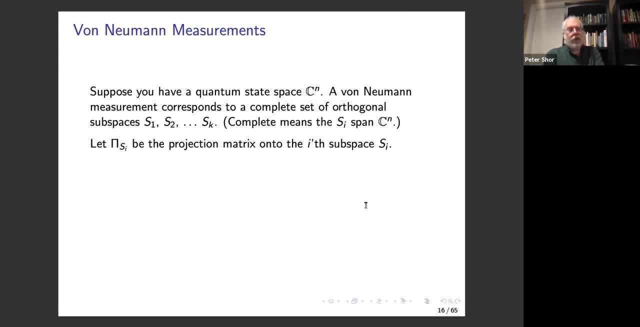 So that's now we want you to say what a von Neumann measurement is. So suppose you have a quantum state, space c to the n. A von Neumann measurement corresponds to a complete set of orthogonal subspaces. So complete means that all of these orthogonal subspaces. 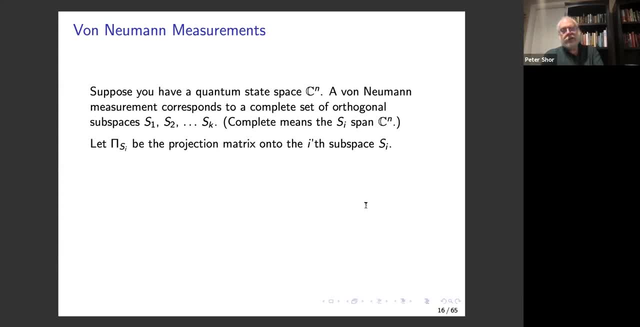 are a complete set of orthogonal subspaces. So complete means that all of these orthogonal subspaces and c sub n And that means that the sums of their dimensions has to be n. So if we let pi, sub s, sub i be the projection matrix, 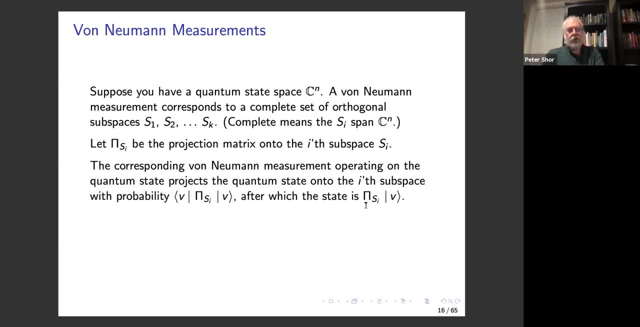 onto the i-th subspace. the corresponding von Neumann measurement projects the quantum state onto the i-th subspace. So you get i as the classical output of the measurement with probability v, pi, sub s, i, v, And this v is the projection matrix. 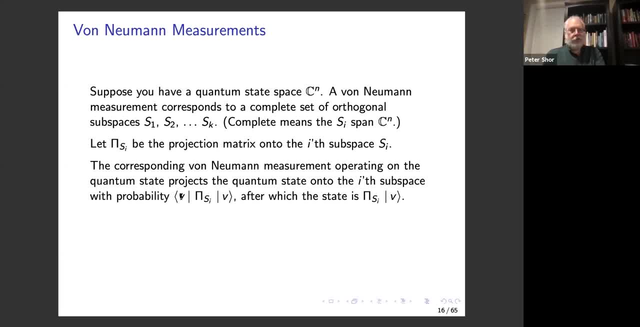 This is the original vector And this is the left thing is called a bra, which means you put them, and this right thing is called a ket. You put them together and you get a bra ket or a bracket, which is, I guess, Dirac's wordplay. 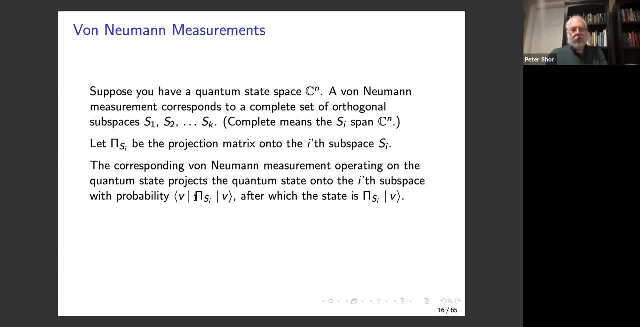 And so it's the conjugate transpose projection matrix v, which is just a scalar And that's a probability, And after you make the measurement, the state, the quantum state, is the state projected onto the i-th subspace, And there, indeed, is a more general class of measurements. 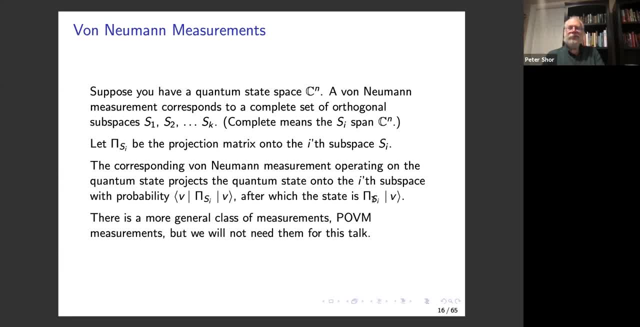 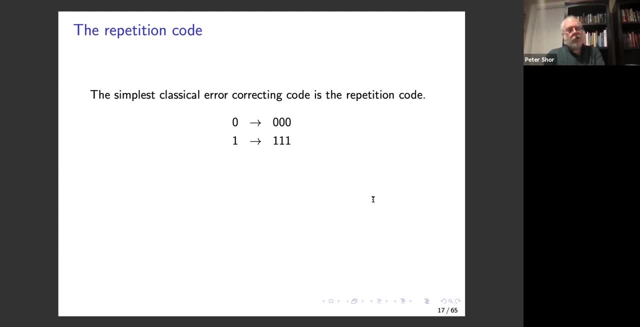 but we're not going to need them for this talk, so I won't define them. Okay, So now I think we know enough to talk about quantum error correcting codes, So let's go back and look at classical error correcting codes, The simplest classical error correcting code. 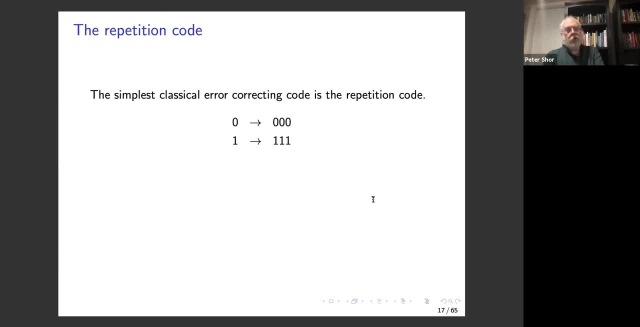 and it's the only one known before around 1950 or so- is the repetition code. So you have a zero, So maybe this a bit. zero means attack at dawn, So it's a message and you send it to your general. 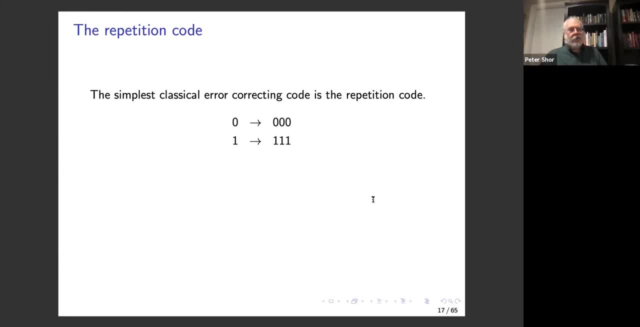 Now you want to make sure that your general gets this message. so instead of sending one horseman with a message, you send four horsemen with a message, and you know one of them is going to get through with high probability. So that's the idea behind the classical error correcting code. 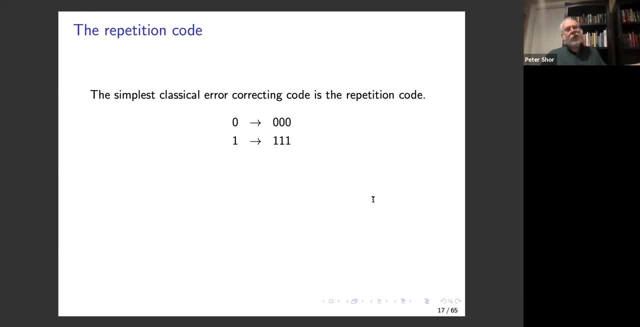 We just replace each bit with many copies of it, And three is the smallest number that will work And that's the one we'll use in this example, because it's really easy to think about And you can see that you can decode it just by taking the majority. 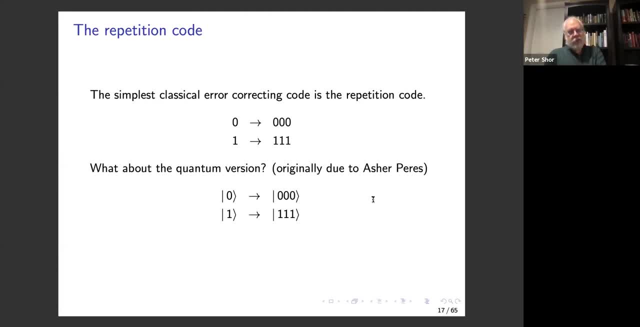 And if one bit is corrupted, you still get the original message. Well, what about the quantum version? Well, where you can take the zero state to zero, zero, zero. three copies of the zero state and one, two, three copies of the one state. 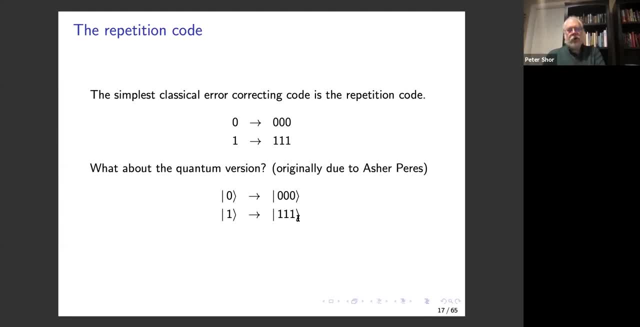 And that is a three qubit quantum error correcting code. How well does it work? Well, we'll explain that in the next few slides. So suppose you have a bit flip. So what a bit flip is is the sigma X Pauli matrix. 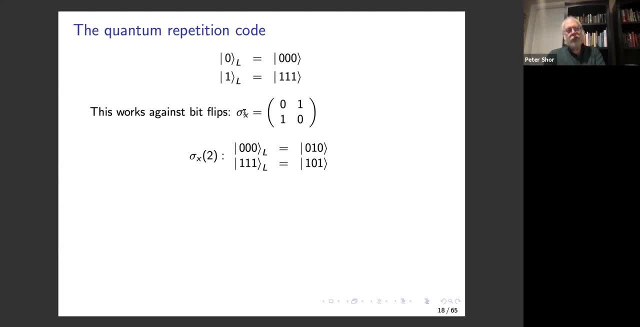 There are three Pauli matrices: sigma X, sigma Y, sigma Z, and I'll introduce them all eventually in this talk. But right now the sigma X is a bit flip And if you apply a sigma X to the second bit takes zero, zero, zero L. 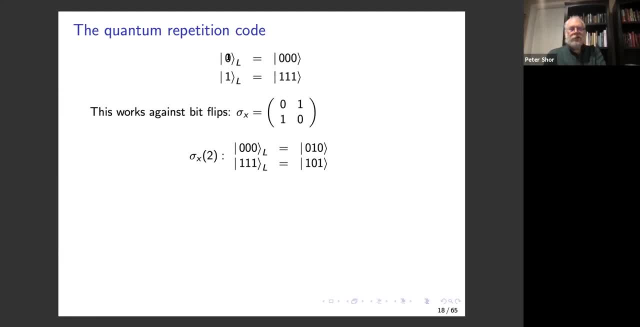 Okay, this L should not be there, I'm sorry. Zero L is a logical zero and it's represented by three zeros, And a one L is a logic L represented by three ones, And this should just be zero, zero, zero. 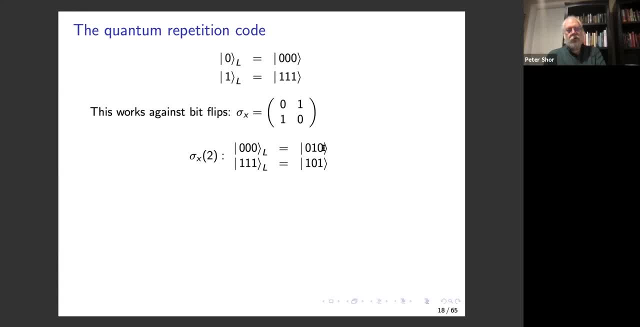 So it takes zero zero, zero to zero one zero- It flips the second bit. and one one one to one zero one- It flips the second bit. So now we ask which bit is different. So asking which bit is different is a measurement. 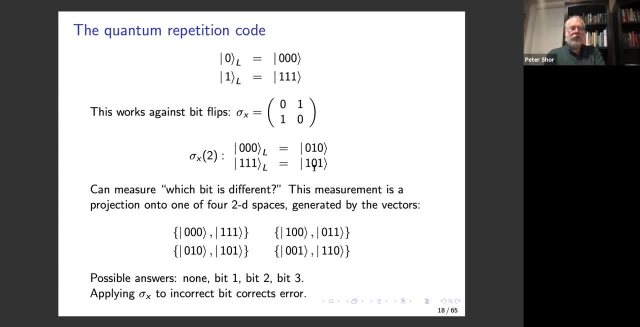 that projects it onto one of four two dimensional subspaces, And you know, this dimensional subspace is zero, one zero and one zero one. So this is a set of vectors for which the second bit is different And the possible answers to which bit are different. 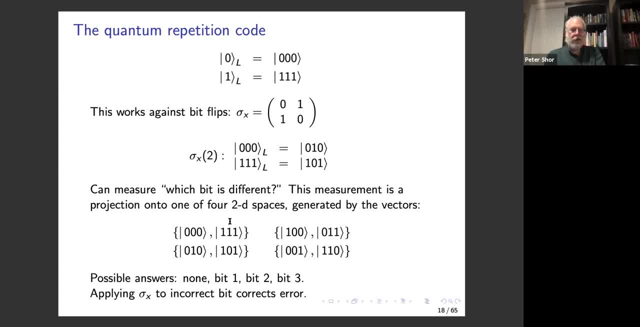 are none bit one, bit two and bit three, And that corresponds to the fact that there are four subspaces here And now, once we've found the incorrect bit, we can apply a Pauli matrix or a bit flip to this incorrect. 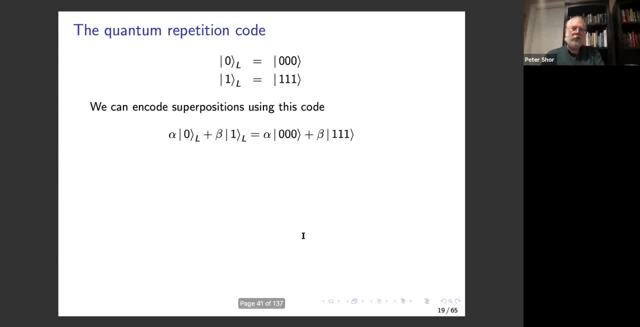 bit and correct the error. So that works. And in fact if you encode superpositions using this code, so logical zero plus superimposed with a logical one goes to zero, zero, zero plus one, one, one one. 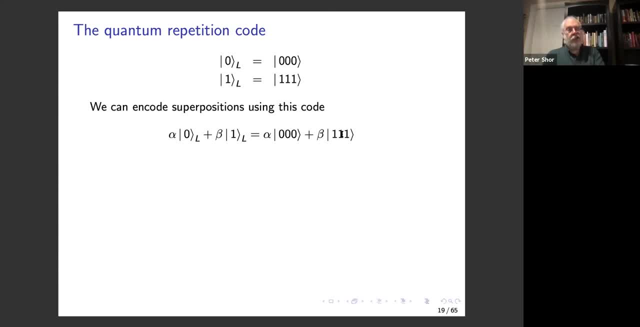 Now, if you look at this, you will see that we're not cloning, because if we're cloning the state alpha zero plus beta one, we would get three copy, three qubits, each of which was in the state alpha zero plus beta one. 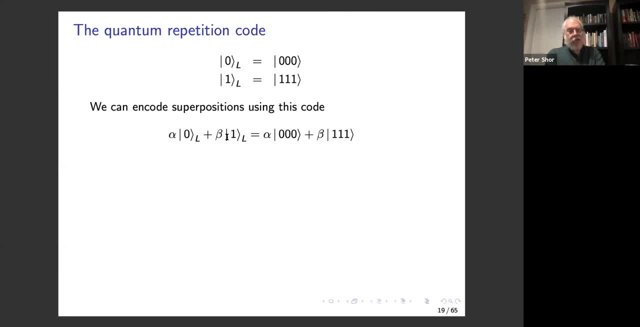 And in fact we get a superposition of zero, zero, zero and one, one one. So encoding in this code is not cloning, which means we can do it. It doesn't violate the no cloning theorem. So suppose we have a bit error in the second bit. 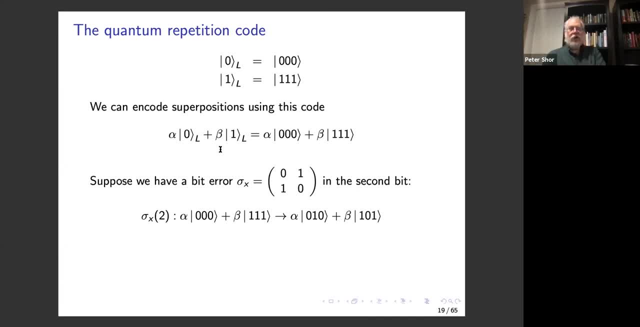 We can correct it And we still stay in the superposition because we project the whole. we project this whole state on to the superposition And when the result is measured, the result is, bit two is flipped and the measurement gives the same answer. 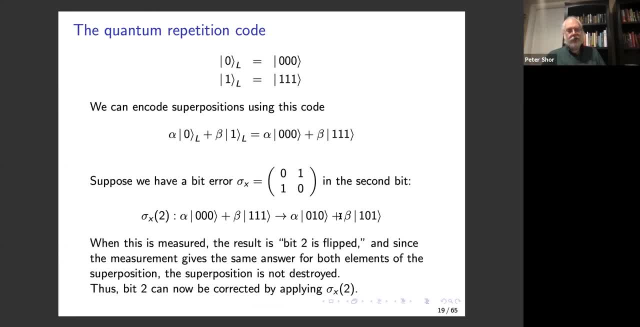 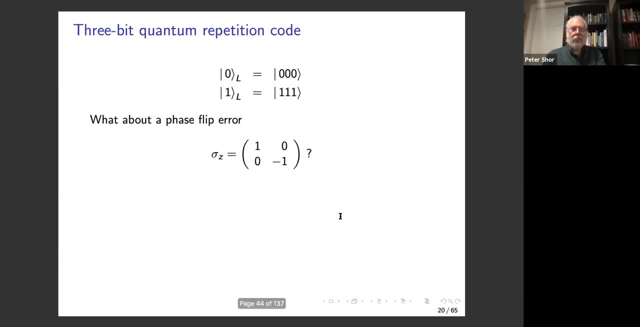 for both elements of the superposition. So the superposition is not destroyed. And now we can correct the error by applying sigma X to the second bit. So what happens if you have a phase flip error In quantum computing? you need to keep phases correct. 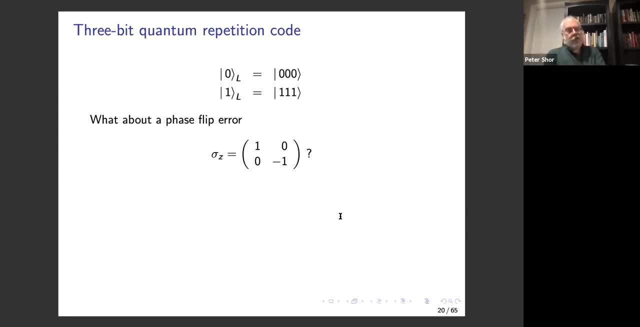 So you need the relative phase between two states to be right. So if you have a phase flip error, it can destroy your quantum computation just as much as a bit flip error could. So what about a phase flip error? Well, here's what a phase flip error does. 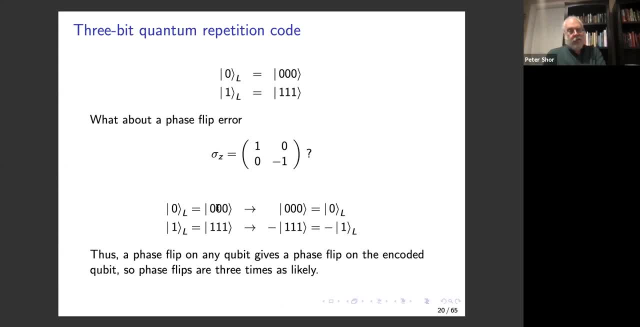 If you apply a phase flip error to well any of these bits, it takes a zero. It takes a zero to a zero and a one to a minus one. So it takes an encoded zero, a logical zero to a logical zero and a logical one to minus logical one. 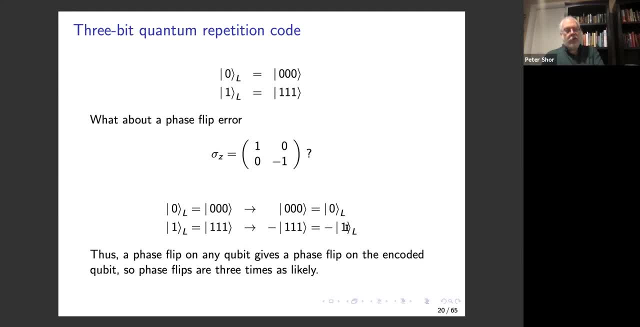 So a phase flip on any qubit gives a phase flip on the encoded qubit. So our code, you know if you have some rate of phase flips on individual qubits, say P and P, small phase flips are three times as likely in this code. 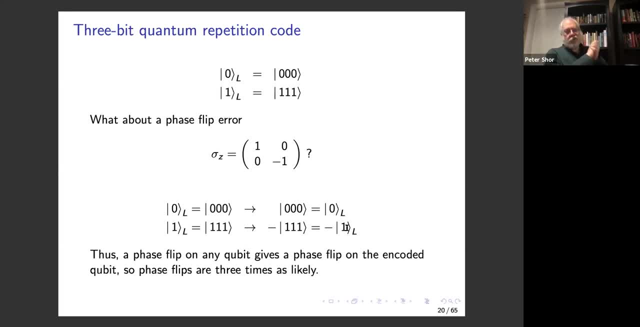 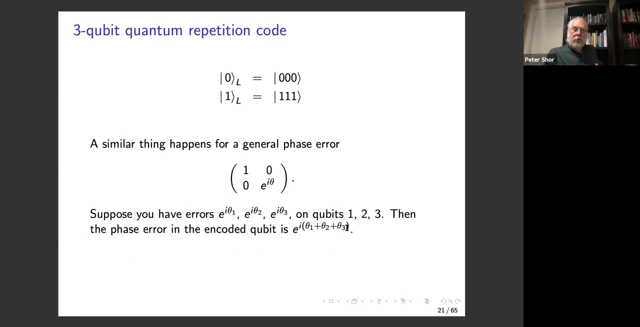 So we're correcting one type of error, but we're, you know, making another type of error much worse. So at first it looks like we haven't done anything. Now what I noticed was: oh wait, no, that's the next slide I'm talking about. 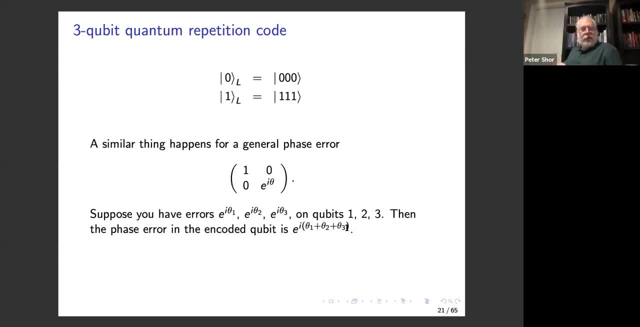 So a similar thing happens for a general phase error. And if you have errors, either the I theta one, either the I theta two, one, two, three, four, five, six, either the I theta three on qubits one, two, three. 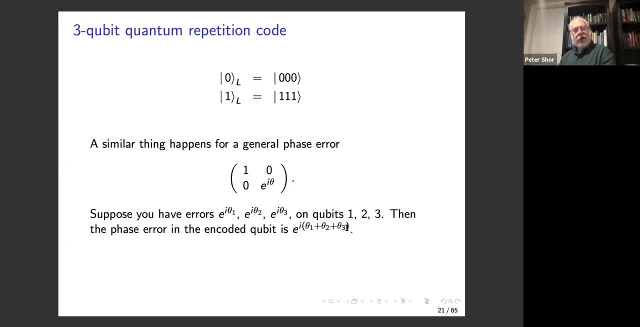 these are phase errors, Then the phase error in the encoded qubit is the phase error corresponding to the phase, the sum of these three phases, And that means phase errors behave like errors in analog computation, And errors in analog computation are generally known to be uncorrectable. 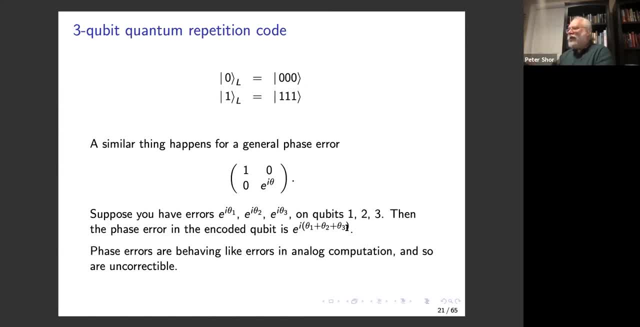 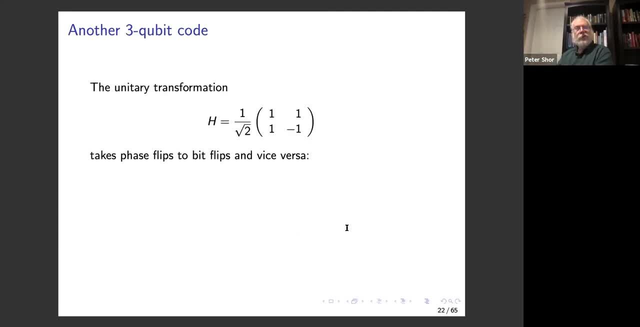 So our nice analog of the repetition, the repetition code, hasn't helped. Well, there's another code that we can look at. What you can see fairly easily is a unitary transformation, which is called a Hadamard gate. takes bit flips to phase flips and vice versa. 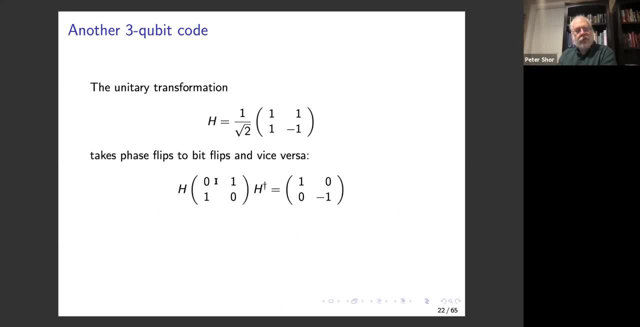 And you can see this by just saying that Hadamard times bit flip, times conjugate. you know the conjugate transpose of the phase flips, The conjugate transpose of the Hadamard matrix, which is actually the Hadamard matrix, is a phase flip. 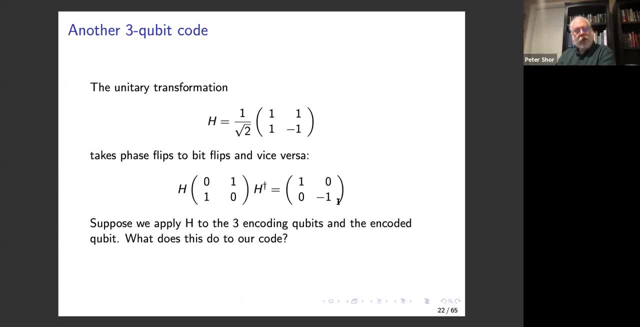 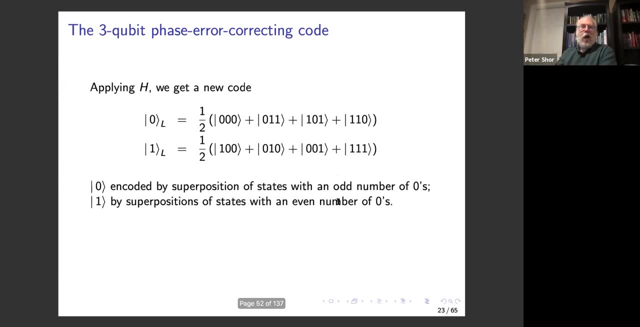 And so suppose we apply the Hadamard transform to original code. what do we get? We get a new code, And I'm skipping all the computations for how you apply the Hadamard transform, but it's absolutely very straightforward. So zero is encoded by a superposition of states. 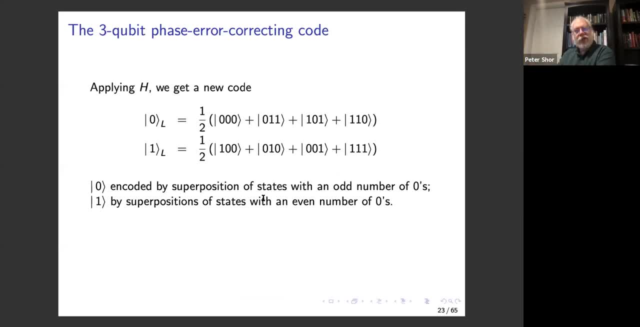 with an odd number of zeros And one by the superposition of states with an even number of zeros. So now we can see a bit flip on. any qubit exchanges zero and one, which means it takes a state within a superposition of odd number of zeros. 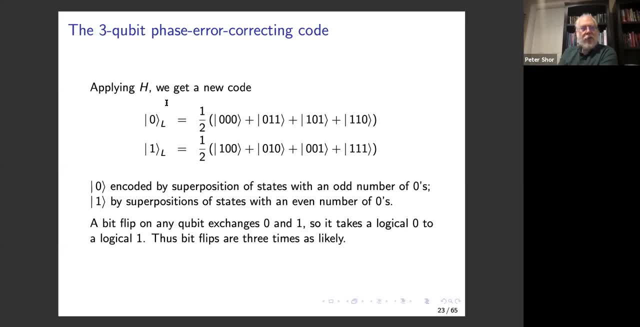 to a superposition of an even number of zeros and vice versa, And that means it takes a logical zero to a logical one. So a bit flip on any qubit takes induces a bit flip on a logical qubit, So bit flips are three times as likely. 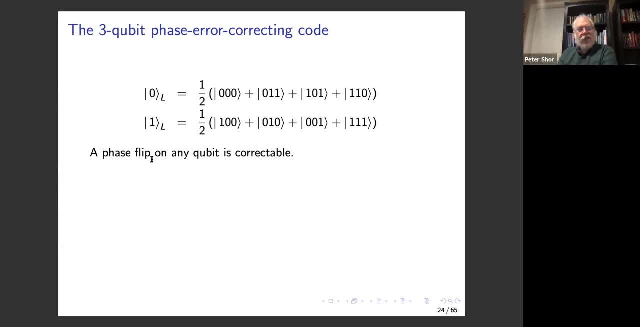 But a phase flip on any qubit is correctable And that's because it takes a state to an orthogonal state And that means that there is a Von Neumann measurement which will tell you which state had a phase which qubit has. 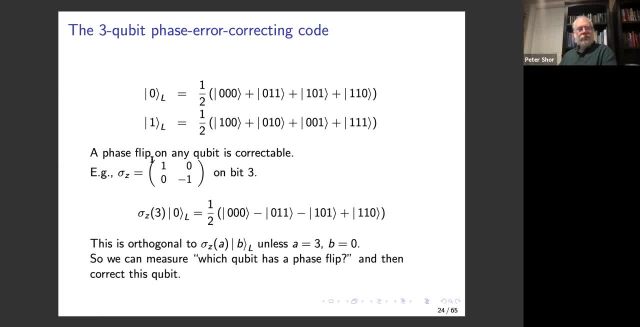 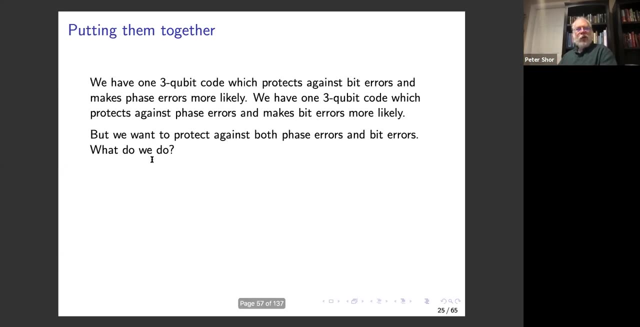 a phase flip, And then you can Undo it. So now we have one code that corrects phase flips but makes bit flips worse, One code that corrects bit flips and makes phase flip worse. What do we do? Well, we put these two codes together. 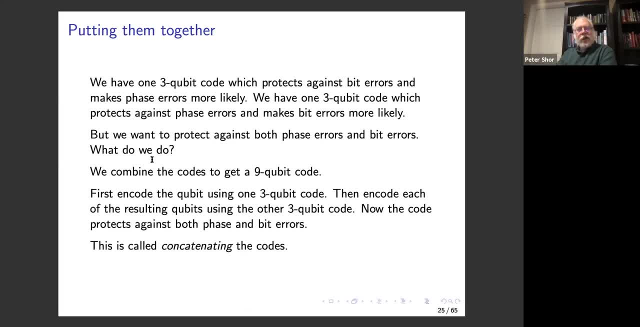 So technically what we do is we can concatenate the two codes. We first encode the qubits using our three bit phase correcting code And then we encode each of the resulting three bits with our qubit bit error correcting code And it turns out the resulting code. 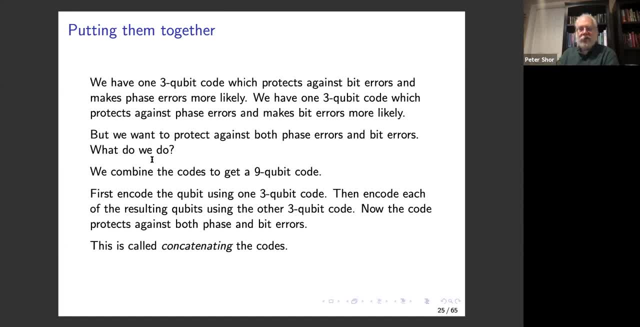 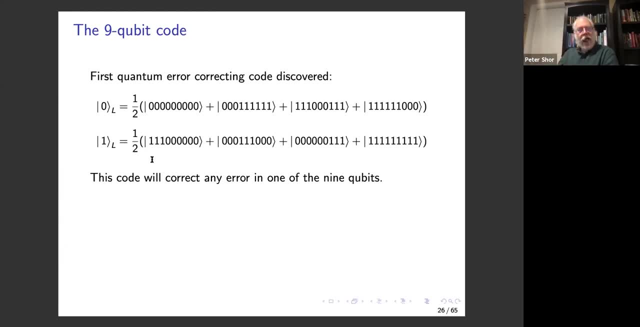 predicts against both the phase errors and bit errors, So this is called kinetic, concatenating the three codes. So this was the first real quantum error correcting code discovered, And this is what we're going to do. This is what it looks like and this code. 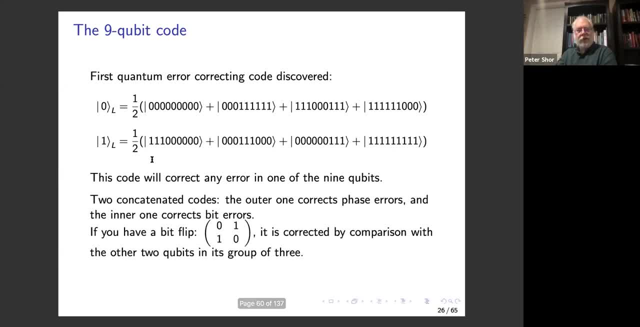 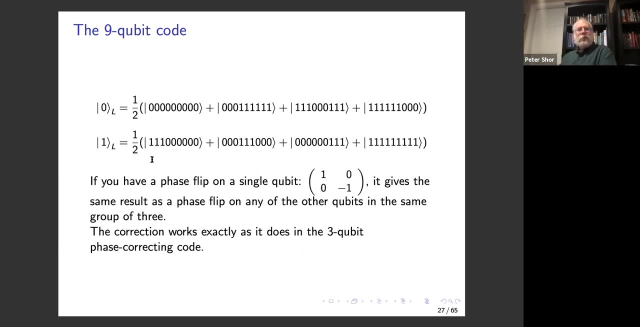 will correct any error in one of the nine qubits, And the outer code corrects the phase errors and the inner one corrects the bit errors. So if you have a bit flip, it's corrected, by comparison with the other two qubits in this group of three. 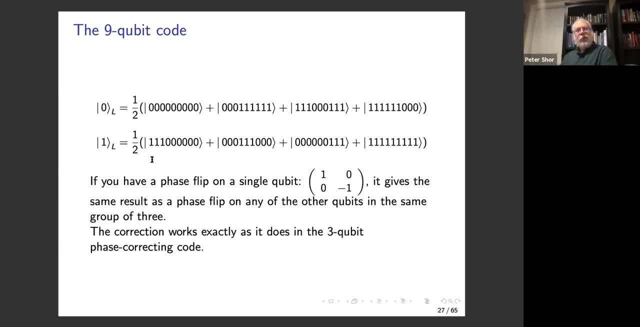 And if you have a phase flip on a single qubit, it has the same result as a phase flip on any of the other qubits in the group of three. And what this means is you can use the correction process exactly as you did in the three qubit phase error correcting. 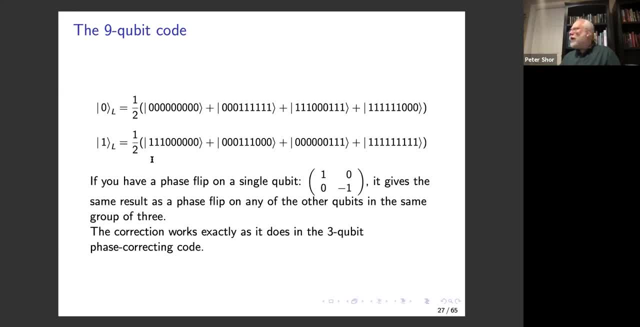 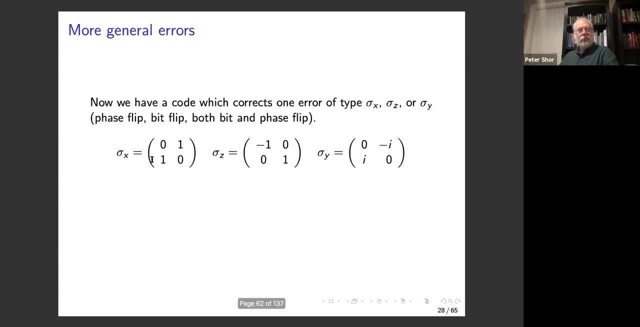 code And you can correct a phase error in any single qubit as well as a bit error in any single qubit. And that means that because you can correct both a bit error and a phase error, You can correct this third Pauli matrix, sigma y. 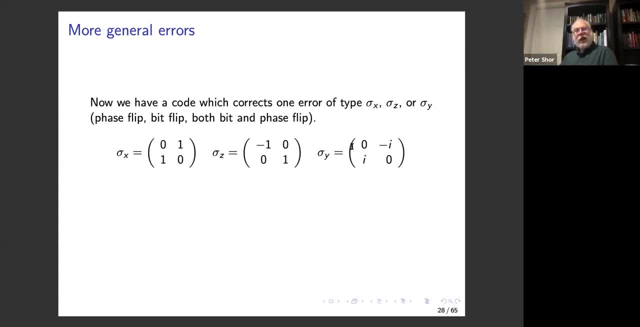 which is this is its definition And it corresponds to both a phase error and a bit error. So sigma y is just sigma x times sigma z with an extra i factor, And you put the i factor in to make the three matrices behave symmetrically. 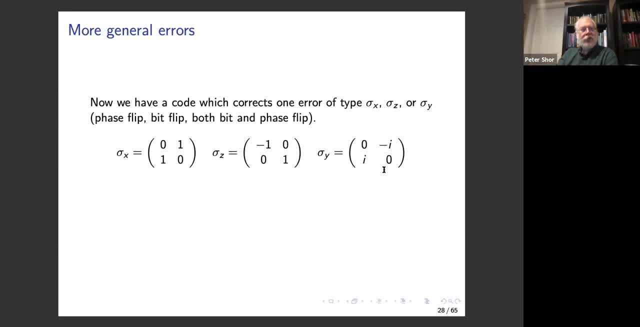 So this is the standard physics definition of the three Pauli matrices. But there are There are many, many more quantum errors. you can apply to qubits And you can ask: can these be corrected? So you can take an arbitrary unitary matrix. 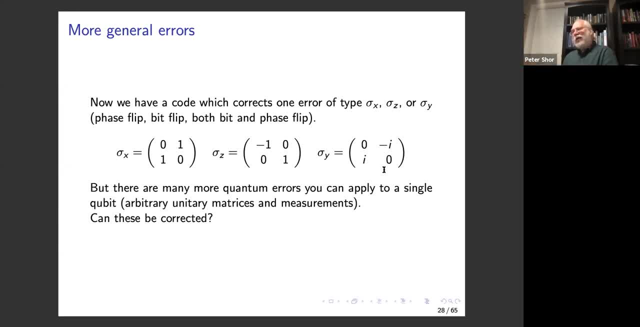 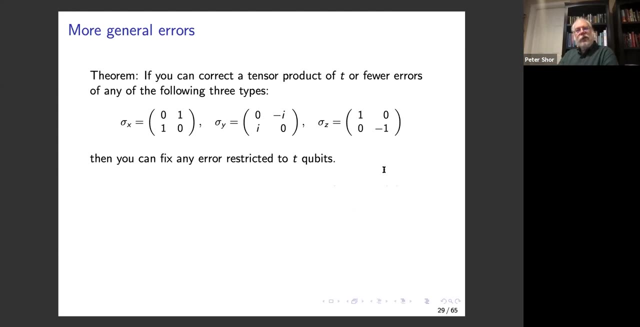 and apply it to a single qubit, And that's a valid quantum operation. You can take a measurement and apply it to a single qubit- another valid quantum operation. So you can ask: can you correct these? So the theorem is: if you can correct a tensor product of t? 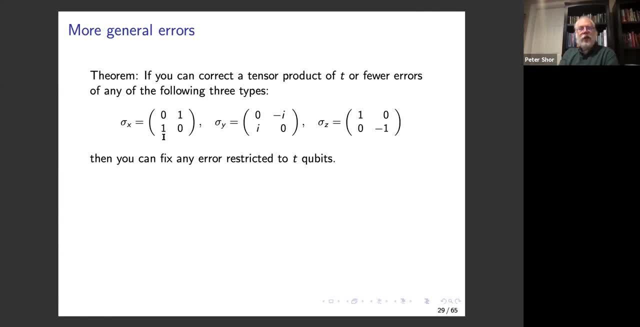 there are fewer of the following three types. So you have t errors And you can correct t errors of a single Pauli matrix And technically that's t Pauli matrices or a Pauli matrix on t of the qubits tensored with an identity matrix on the rest of the qubits. 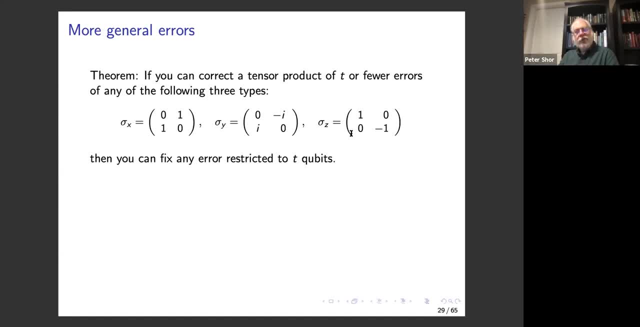 Then you can fix any error. We see It's restricted to t qubits And I am not going to give a proof of this, but I'll give a proof sketch And the proof sketch is basically the identity matrix and sigma x, sigma y and sigma z form for a basis. 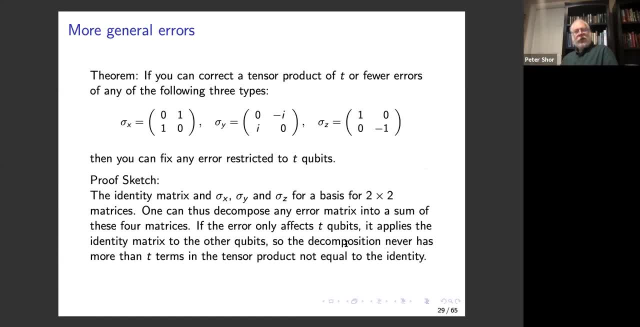 for 2 by 2 matrices, And thus if you have a single qubit error, you can decompose this error into an identity matrix component And three Pauli matrix components, And then when you measure the error, it will project the error onto one of these three things. 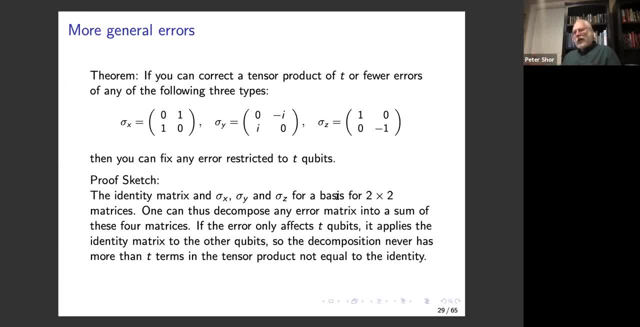 And well, the state collapses if you use the language of physicists to actually have the error that you measured, in which case you can correct the error that you measured And, in fact, you can decompose any error on t qubits too. 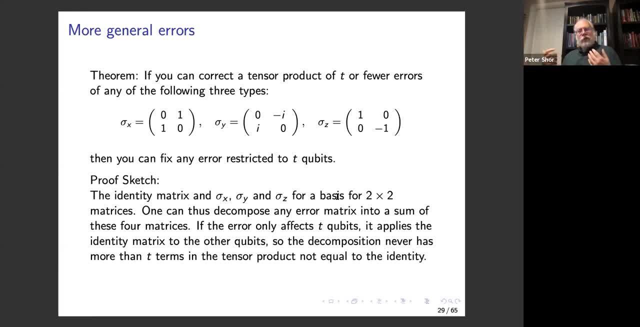 So you can do some of tensor products of t of the Pauli matrices with the identity on those qubits. So if you have an error that only affects t qubits and you can correct any Pauli-type errors on t qubits, then you can correct any error on t qubits. 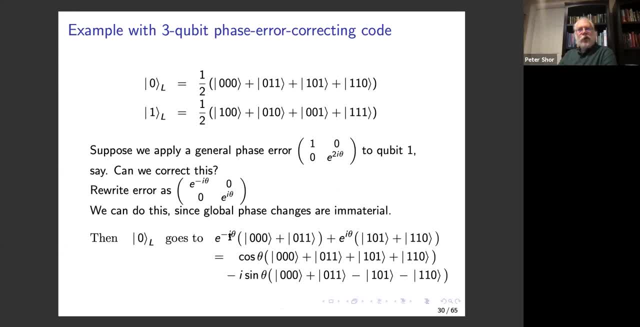 And we will do an example of this for the phase error correcting code, just because This is the biggest code you can actually. I mean, this is a simple example, but you can see what's actually going on, So you have. so here is the phase error correcting code. 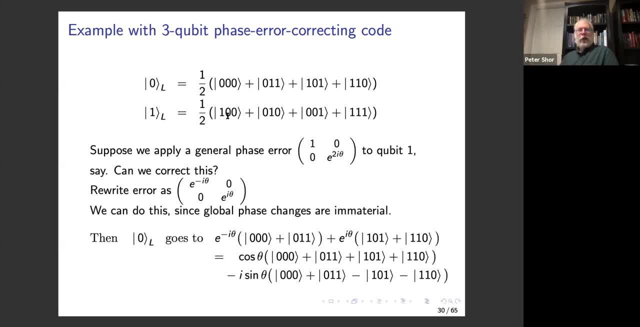 This is an encoded 0 and an encoded 1.. And what happens if you apply a general phase error to some qubit? Can we correct this? Well, we can rewrite the error as e to the minus i theta and e to the i theta in the diagonal. 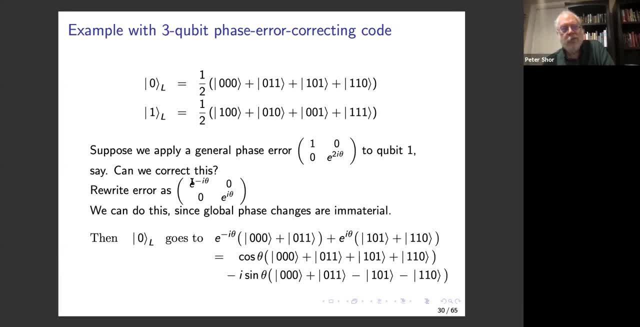 because multiplying a quantum state by an arbitrary unit complex phase doesn't change the quantum state. So we rewrite the error as this and then apply it And let's see. OK, I have my, I have the chat, So suppose we apply it to qubit 1.. 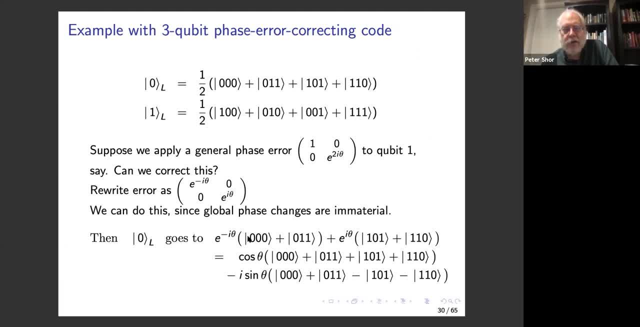 Then we get an e to the minus i theta for all of these basis states which have a 0 in the first qubit and e to the i theta on the states which have a 1 in the first qubit, And now you can rewrite this as cos theta applied to well. 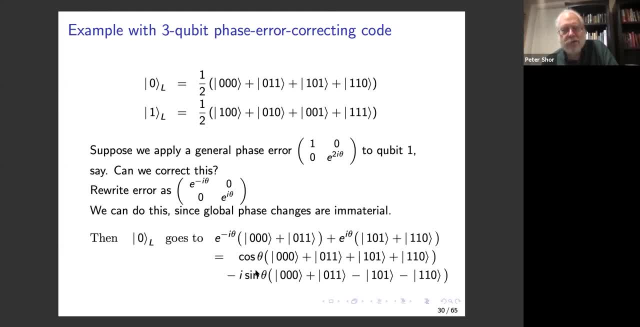 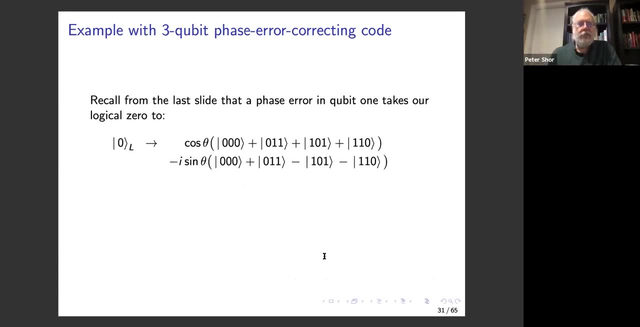 applied to this, which turns out to be our logical 0, and minus i sine theta. applied to this, which turns out to be the logical 0, with a phase flip on the first qubit. And this when we measure which bit has a phase flip. 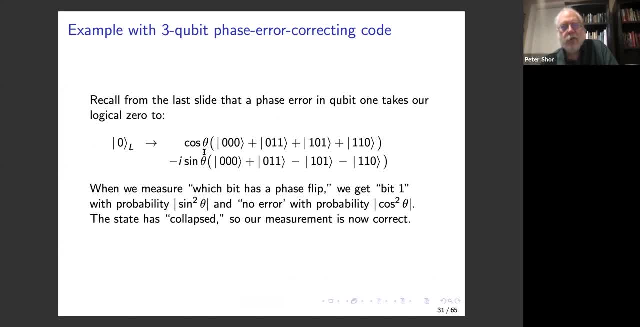 we get bit 1 with probability sine squared and no error with probability cosine squared, And so the state has now collapsed, Our measurement is now correct and we can fix the error, And that's exactly the same thing that happens with general errors with the theorem I gave two slides ago. 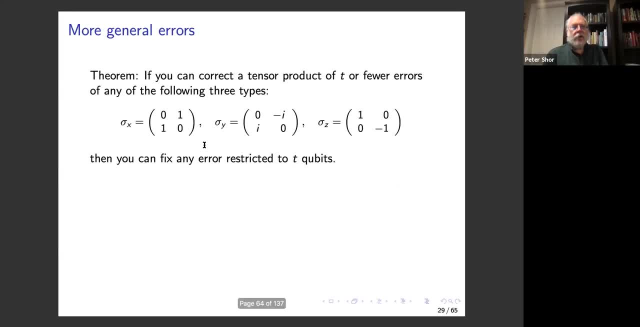 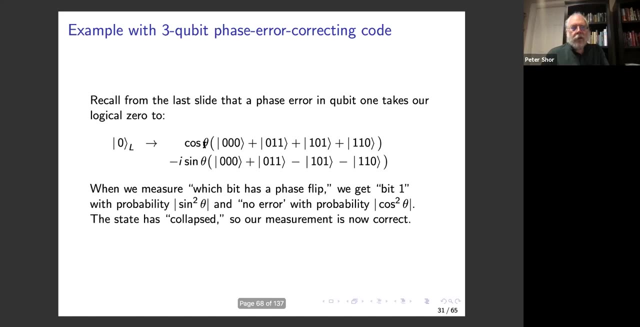 Let's see if we can find that If you can correct a tensor product of t or few errors, then you can correct any error restricted to t qubits. That is correct. That follows the exact same proof as our example. OK, So now we know our quantum error-correcting code. 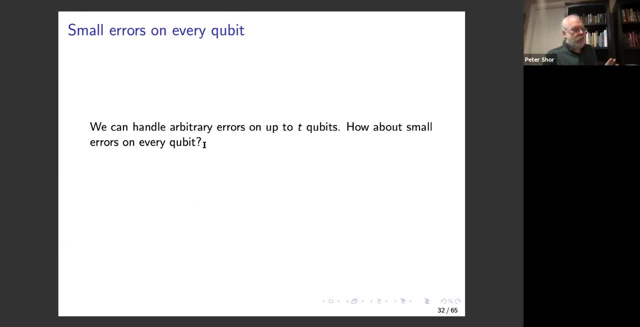 can handle arbitrary errors on up to t qubits. What happens if we have a small error on every single qubit? OK, so I am not going to go into details about this, But essentially what we do is we expand the errors in the Taylor series. 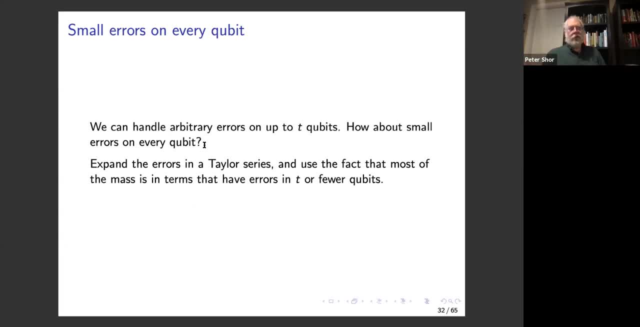 And so we take all of these arbitrary errors, We rewrite them as so. let's assume these errors are independent. We have independent errors on every qubit. We write each of these independent error as a sum of the identity and the three Pauli matrices. 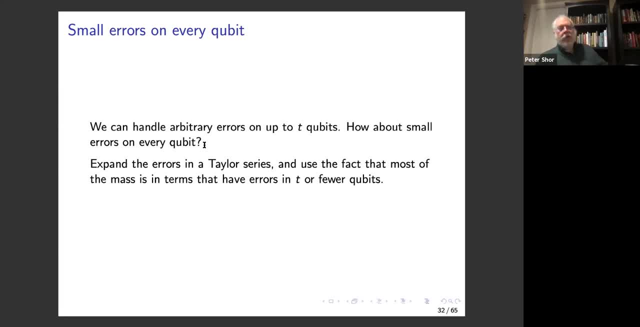 and then just expand, Expand the whole thing out, And the fact that these errors are small means that most of the mass is in terms that have errors on t or fewer qubits. So it will correct all of these terms And then there's a small chance that the error original error. 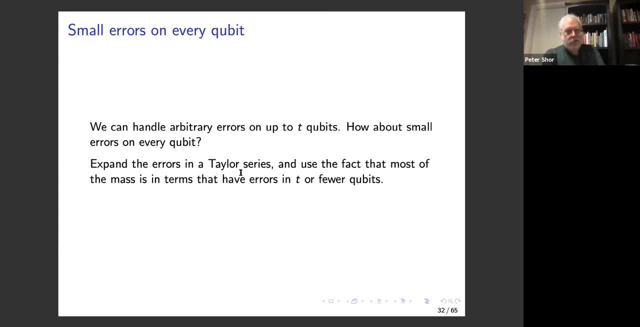 actually had more than t qubits, affected more than t qubits And we can't correct those errors. But That's a very small probability And the same thing is on a class. same thing holds on a classical error correcting code. 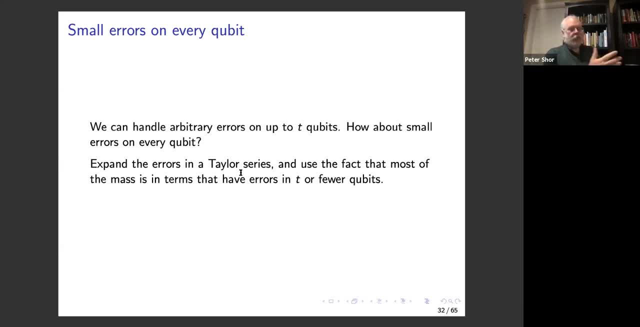 I mean, suppose you have a code that corrects up to 10% errors and you have a 0.05 error rate- 5%- There's a small probability that you're that more than 10% of your bits will have an error. 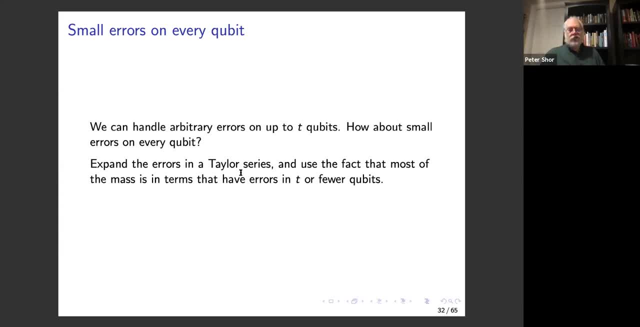 and then your code will fail. But if you chose- You know enough qubits and 10 and you know 10% and 5% different enough, then the chance that the code fails to correct the error is very, very is exponentially small. 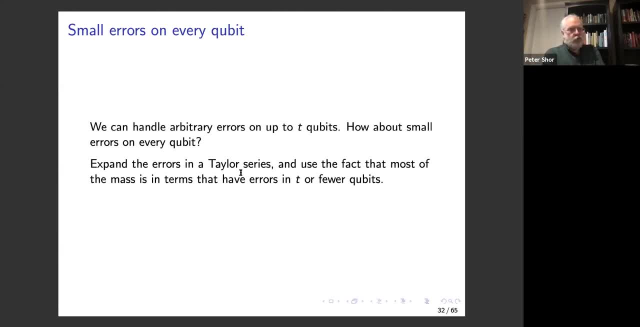 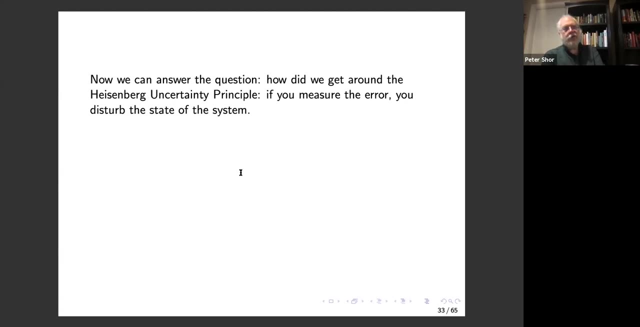 And the same is true here. If you choose your code right, the chance that it fails to correct the errors will be exponentially small. Okay, So now we can go back and answer the question: How did we get around the Heisenberg uncertainty principle? 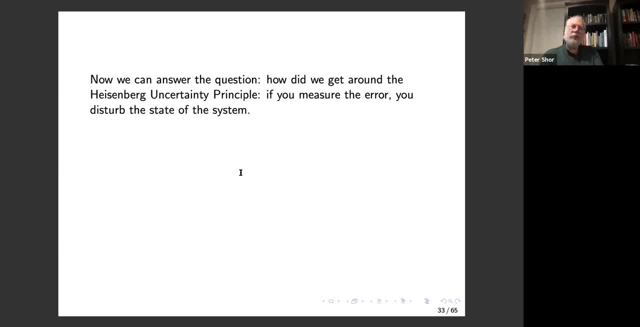 Which says: if you measure the error, you disturb the state of the system. Well, what we did was we constructed codes where we can measure the error, Assuming it falls into some set of likely errors, without measuring the encoded quantum state, And then we can correct the error without disturbing the original quantum state. 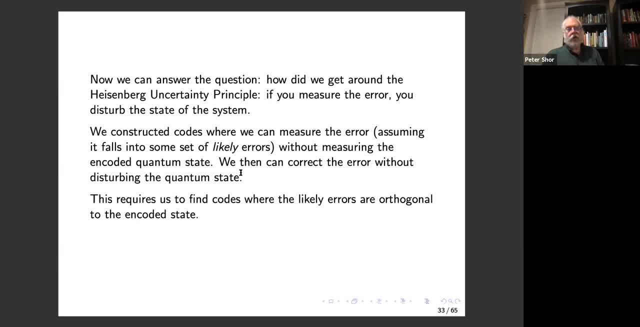 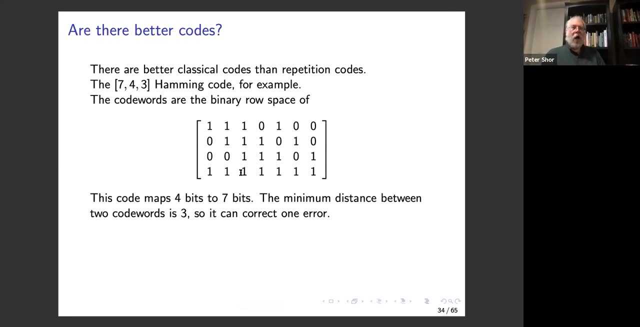 So what this does is? this requires us to find codes where the likely errors are orthogonal to the encoded state. Okay, So that was how to correct errors with the analog of repetition codes. But if you look back at classical coding theory in 1948, Shannon 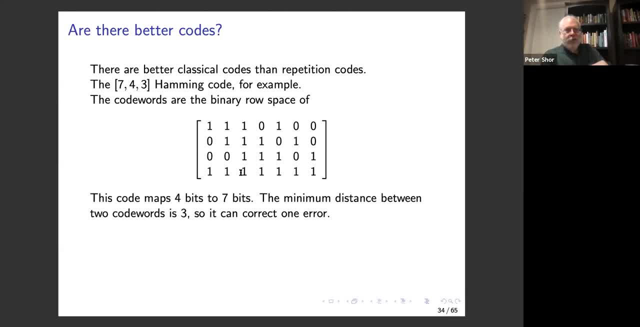 you know, proved that channels have capacities, And you know that proof meant that there were much must. there must exist much better codes than the repetition code, And not long after that, people discovered these, And the first code they discovered was the Hamming code. 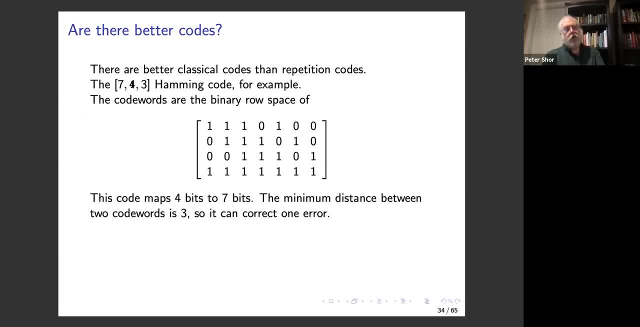 So the 743 Hamming codes means that it encodes four bits into seven bits And it has a distance of three, which means it can correct one error. Okay, So this the code words of the Hamming code are the binary row space of this matrix, which means you just add up all the 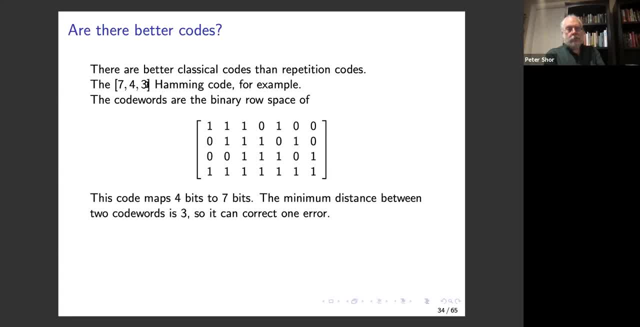 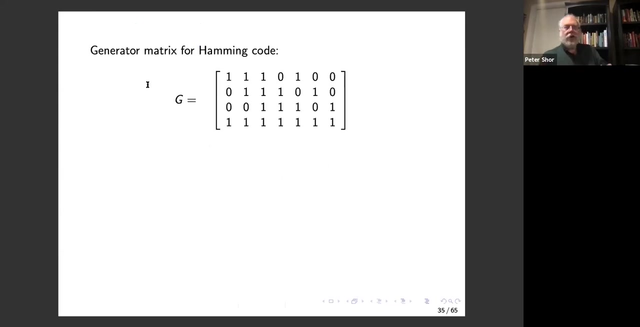 you add up all the numbers, all the bits And you get this. So the quantum analog of the 3-bit repetition code is a 9-cubic code. So you can ask: can you make better Hamming codes? Well, here is the generator matrix for the 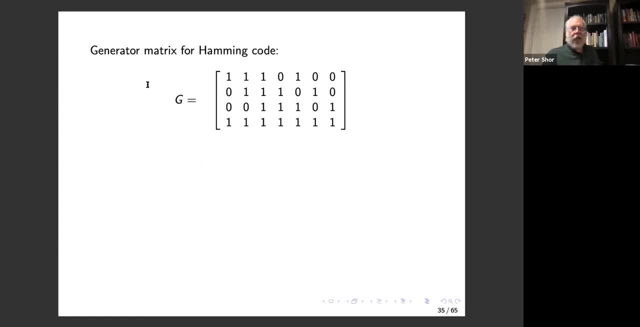 Hamming code And there's something called a parity check matrix, And the parity check matrix is just a matrix whose rows are all orthogonal to the rows here. So, for example, if we take this row 1, 1, 0, 1, or 0, 0, 1, 1, 0, 1, and look at its inner product, with this row it overlaps on two. 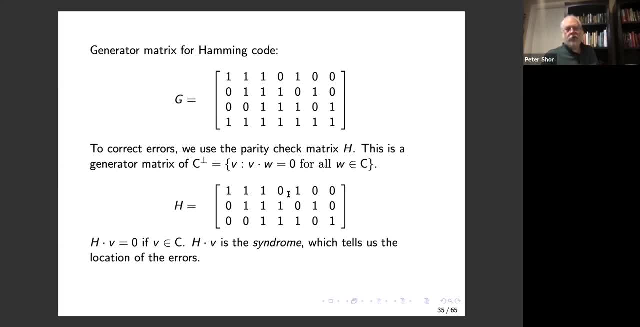 bits. So the inner product of these two rows is 1 plus 1, or 0. So this is a basis for the orthogonal space to this space And, because it's binary, the orthogonal space and the original space contain some of the same. 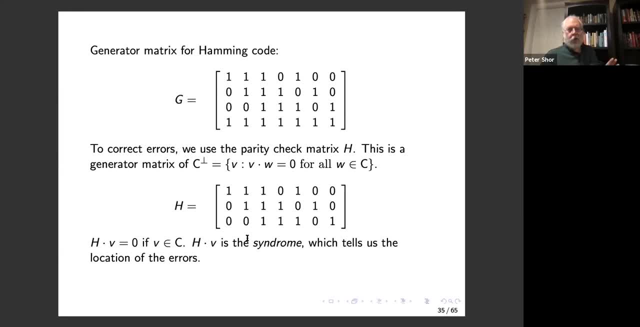 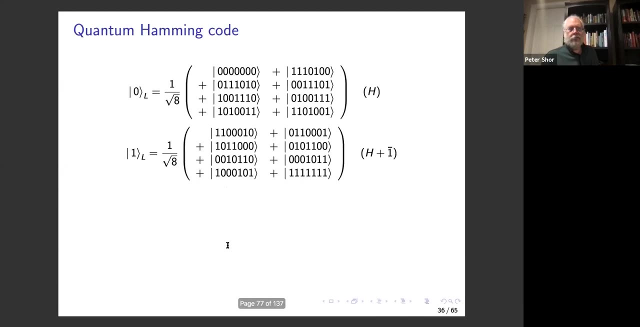 vectors. So how do we correct errors? Well, what we do is we take: H dot V equals 0 if V isn't C, and H dot V is a syndrome which tells us the location of the errors. So quantum Hamming code. 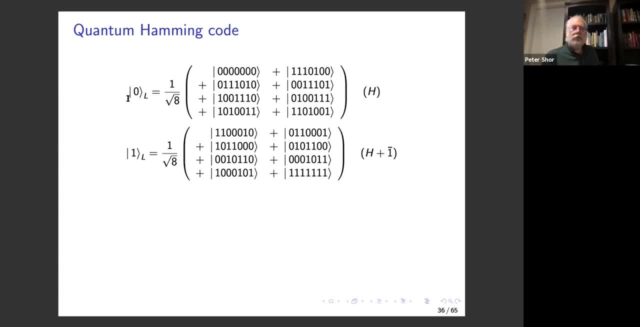 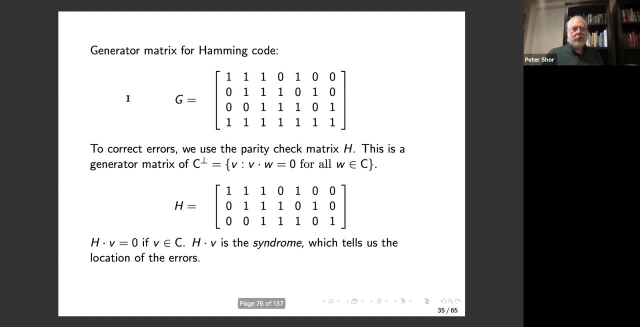 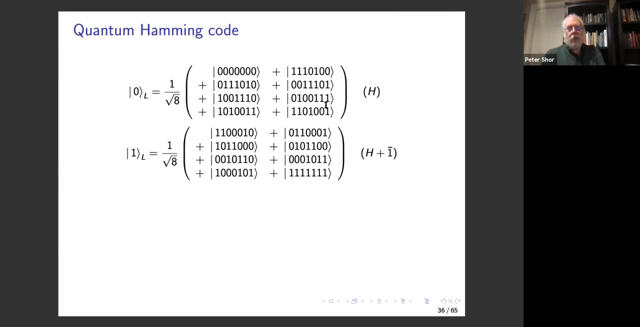 Well, the quantum Hamming code, which I basically found by playing around with this Hamming code, as you take the superposition of all of these vectors in the parity check matrix, in the dual of the Hamming code, and then take the rest of the vectors, the girls and the 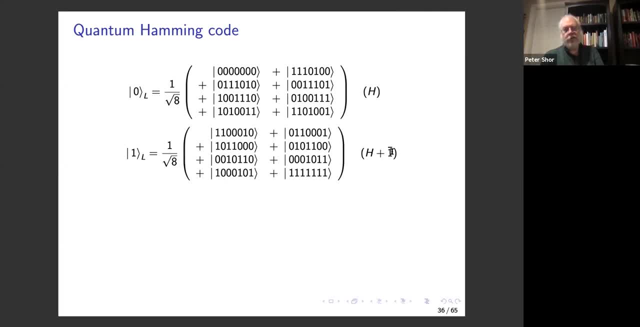 in the Hamming code, which are just these ones plus the all ones vector. So if you start with 0, 1 0 0, 1 1 1 and add the all ones vector to it, you get 1 0 1 1 0 0 0, which is one of the 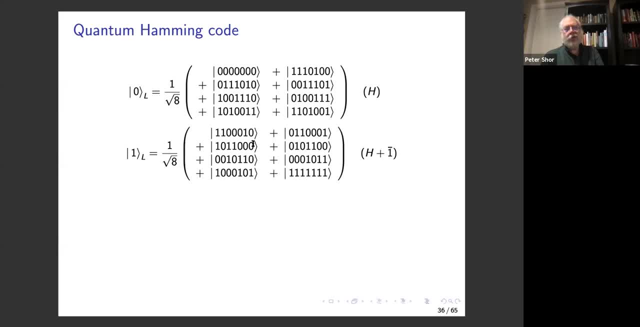 things in this superposition. So this will correct one error using seven qubits rather than nine qubits. So the bit flip errors are all correctable, basically because all of these elements in the superpositions are in the Hamming code And bit flip errors are just, you know, behave exactly. 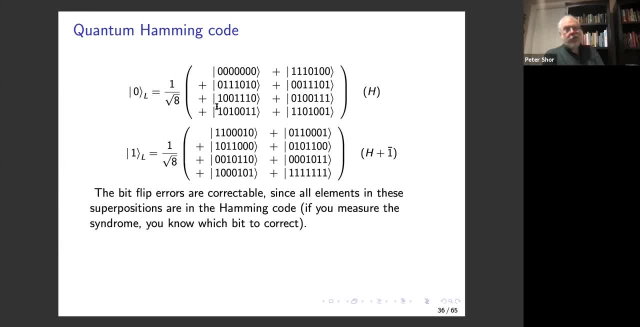 the same as classical single bit errors. So, because the Hamming code can correct all those errors, And if you measure the syndrome, you know which to correct. then the Hamming code can correct a bit flip error. Well, what about phase flip errors? Well, recall we had this transformation that took bit flips to. 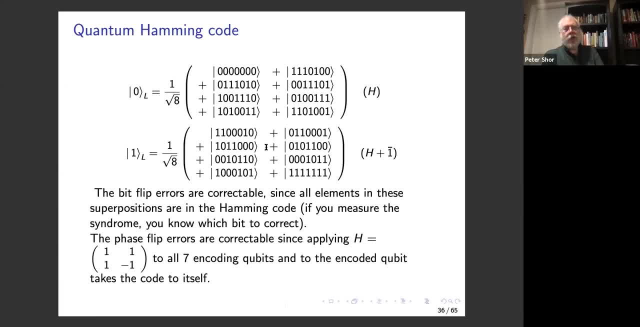 phase flips and phase flips to bit flips. What happens if you apply it to this code? Well, you get the same code back. You get the Hamming code again. So now a phase flip error is correctable because you can just apply a Hadamard to every qubit and 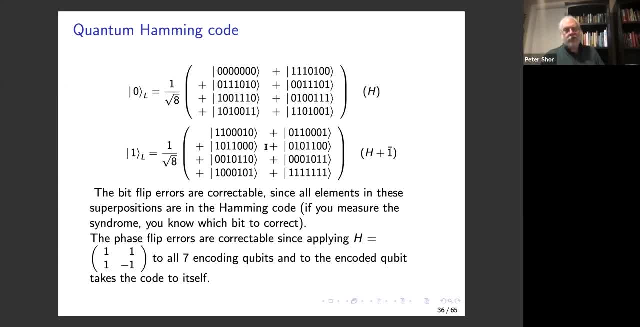 correct And the phase flip error turns into a bit flip error. And now the code is the same, So you can correct phase flip errors. So that's a remarkable property. So we have a code now that corrects bit flip errors and phase flip errors. So by our theorem it will correct any arbitrary. 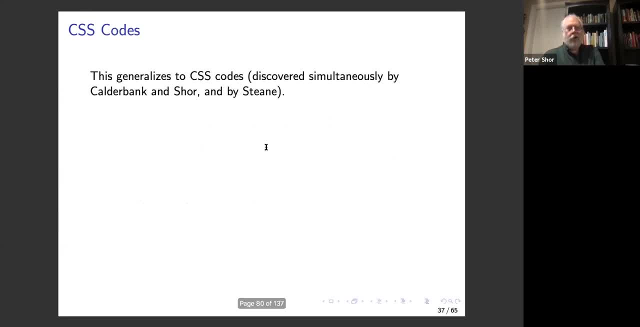 single qubit error. Okay, So now you can ask: well, what happens to this code? Can you generalize it? And the answer is yes, And it's not all that hard, I mean. so now I'm going to go into a little technical. 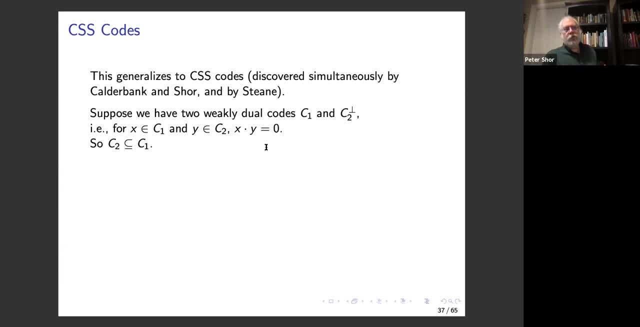 coding theory. So suppose you have two weekly dual code, C1 and C2, perpendicular. So these are two. So weekly duel just means that that the string is going to beäng worst than the根. int in like this: barhelp Sonic Hardware. 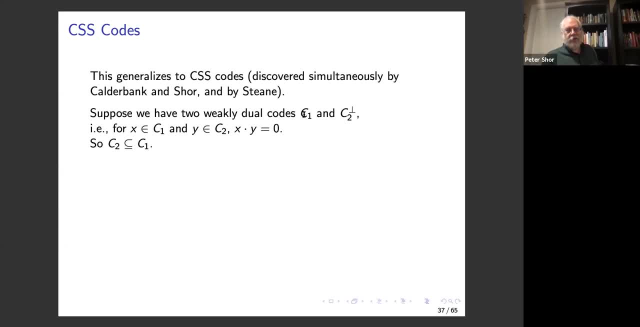 proc Sens int sen sc h. xx means that every code word in this code is orthogonal to every code word in this other code. So for X in C1 and Y in this should be C2 dual X dot Y equals zero. 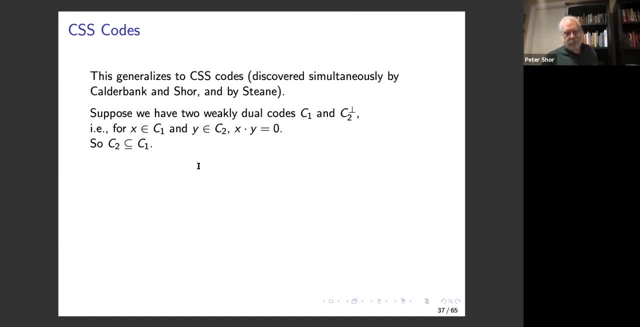 and that means that C2 is contained in C1.. Okay, so we have two weakly dual codes. What do we do? Well, what we can do is define code words corresponding to the co-sets of C2 and C1.. 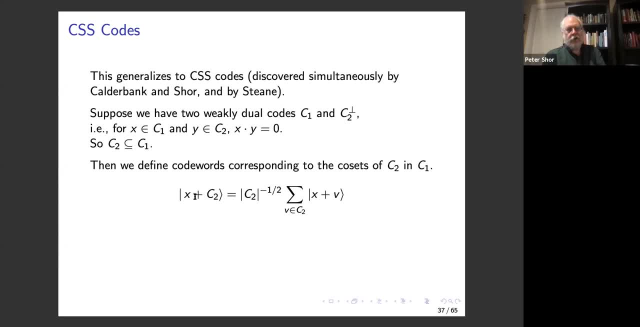 And the code word corresponding to the co-set given by X is just the superposition of all words and that are all code words in that co-set. And what happens is that when we take the dual of this, we get the same code back only. 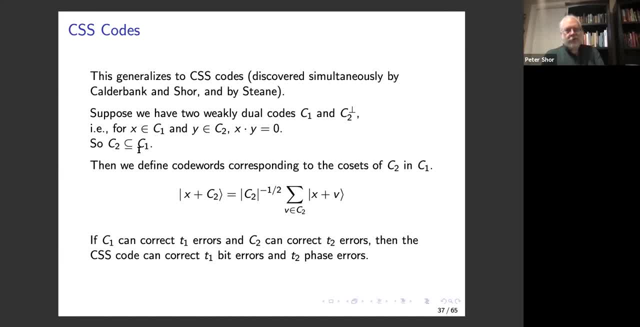 instead of C1 and C2, we have C2 dual and C1 dual, And so if our code C1 can correct T1 errors and our code C2 can correct T2 errors, then the resulting CSS code can correct T1 bit errors. 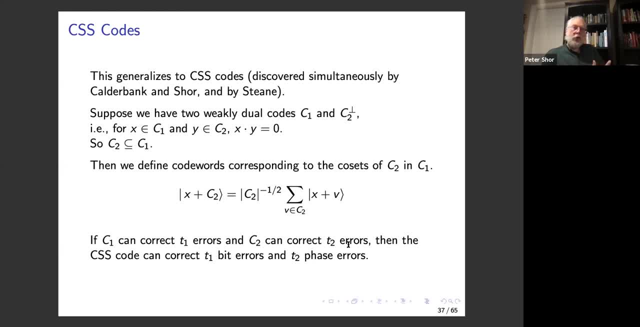 and T2 phase errors. So now we've turned, or we turned, the problem of discovering quantum CSS codes into the problem of discovering weakly dual classical codes which have, or which the weakly dual codes are, good error correcting codes. And actually there's this huge classical literature on codes. 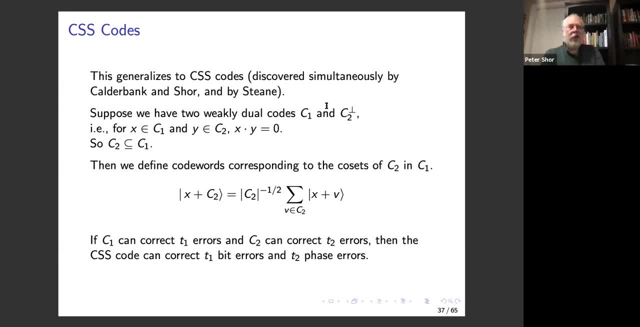 and we can just look at it and find a whole bunch of good CSS codes. And you can also use techniques on classical coding theory to prove theorems about how good CSS codes are, and you can prove so. basically, I mean. 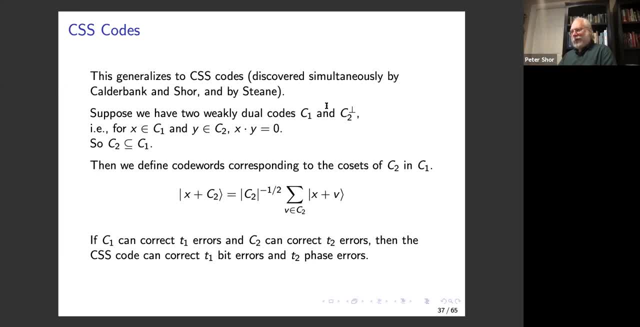 there are all sorts of good theorems on you know. there are all sorts of theorems on what's the minimum distance of a code. I guess this is the you know it's about. it's about the minimum distance of a code. 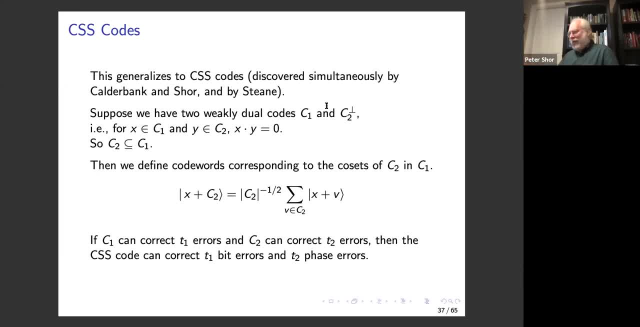 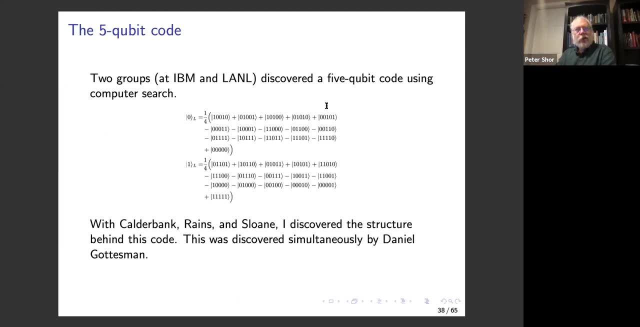 I guess this is the. you know, it's a, it's the Hamming bound, and you can prove. and you can prove, these bounds work for these codes. So are there better codes? Okay, well, so two groups at IBM. 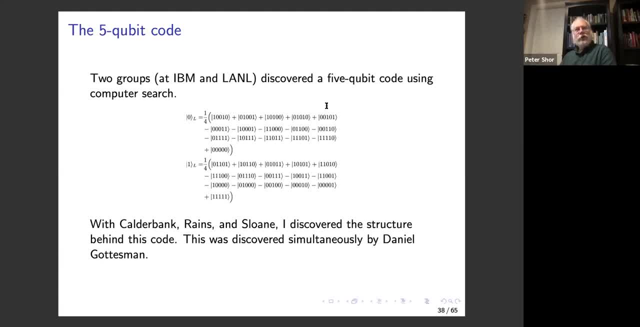 after the paper on CSS codes came out. they basically put finding codes on a super, on a computer search, and discovered five qubit codes And they look different And but in fact by playing around that with them, you could find that they were actually the same. 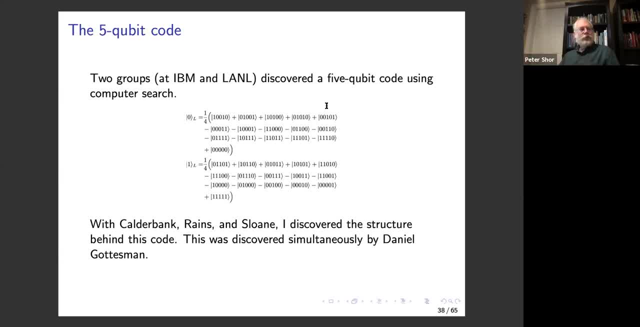 if you applied various transformations to the qubits and permuted the qubits- excuse me- et cetera. So they're both equivalent to this code, which I've written down so you can see some of its symmetries. So we wanted to figure out. 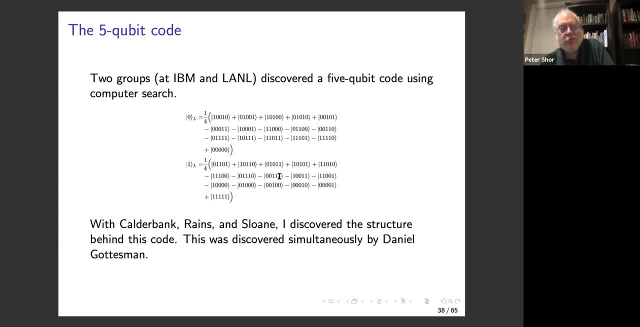 you know, this is obviously has a lot of interesting structure in it. So we wanted to figure out the structure. So I said the first thing to do was to find the symmetry group of this code. And I asked Neil Sloan how you would find symmetry groups of a code. 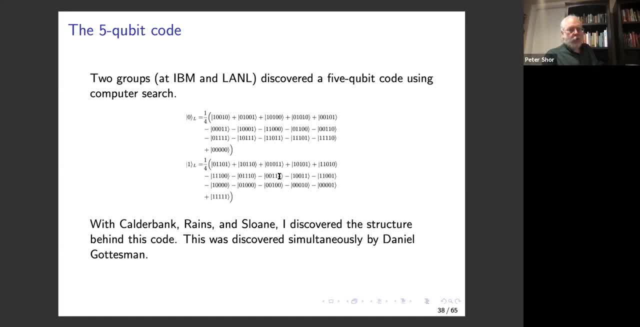 So he told me you should use this computer program, magma, And he gave an example of a magma program which down the symmetry group of a problem that he was looking at then. So I wrote up the program for finding the symmetry group of this code. 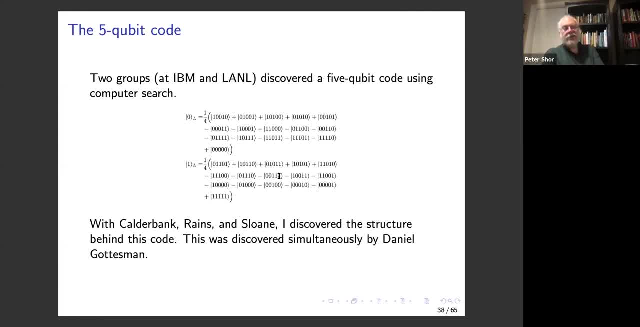 and it spit out 190 million and something. And you know this example program that Neil Sloan had given me looking for his problem gave the symmetry group had the exact same number. So we looked at this more closely and they were the exact same group. 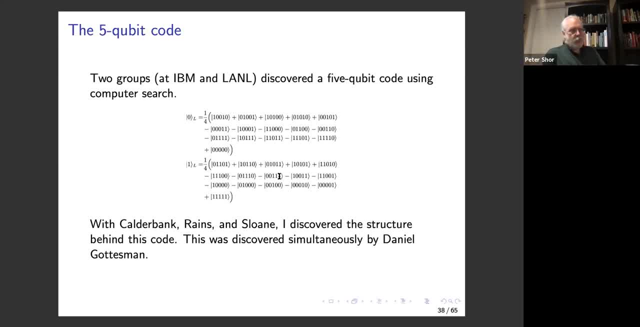 And in fact there was a very interesting relationship between the problem of one codes and the problem of packing Grassmannian spaces, which is what Neil Sloan had been looking at, And this interesting relation gave us the clue for finding all of these qubit. 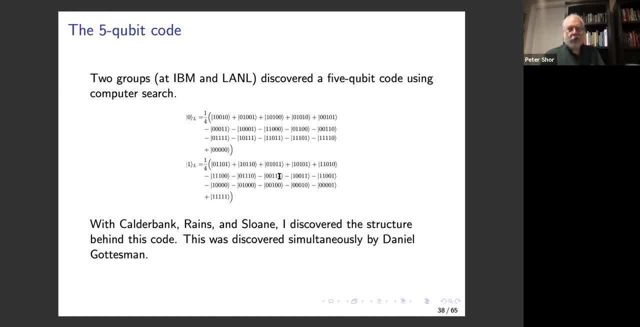 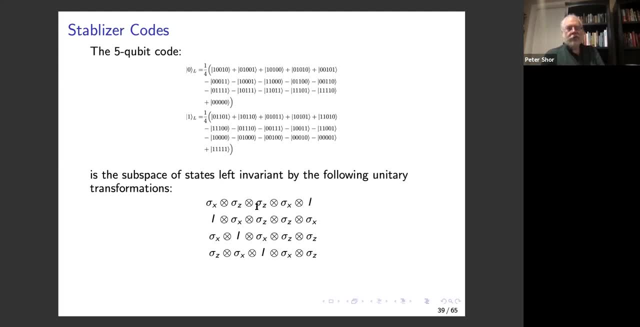 all of these, you know finding this general structure for these codes. So what was that? Well, it turns out that this five qubit code is just well. the five qubit code is really a subspace, And it's the subspace generated by the zero. 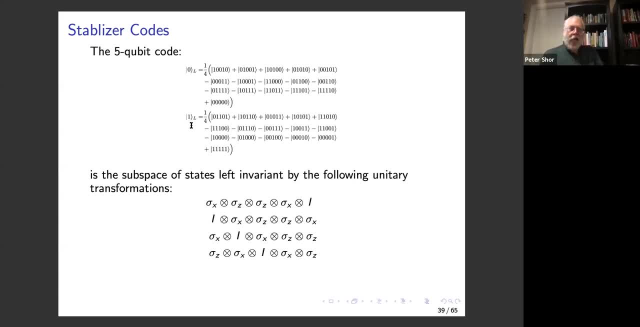 the encoded zero and the encoded one And a code really is a subspace because once you have the subspace, you can choose the- you know an arbitrary orthogonal basis to encode zero and one or however many bits you want You want to encode. 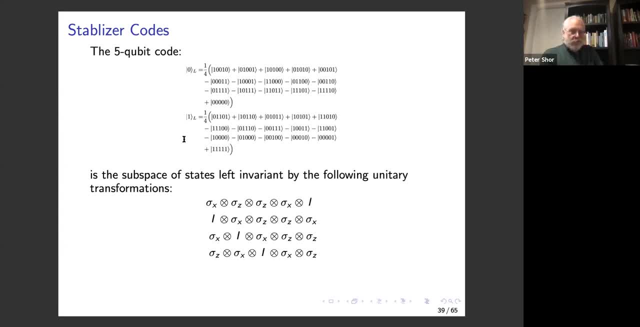 And of course some of these arbitrary bases are much nicer than others, but just from a purely code standpoint, they're all give the same code. So it's the subspace of states left invariant by the following four unitary transformations where you can see that they're tensor products. 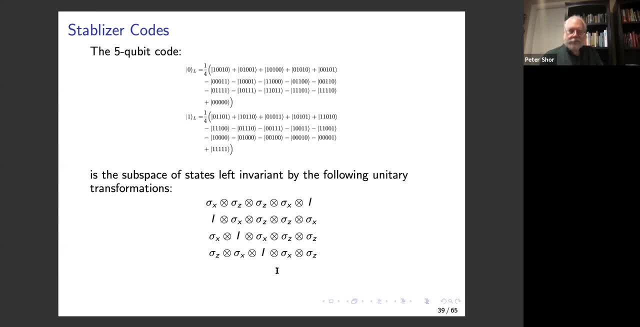 of Sigma Xs, Sigma Ys and Sigma Zs. So this is the general state. you take some tensor product of these three Pauli matrices, X, Y and Z, And you want all pairs of to be orthogonal, to be commuting. 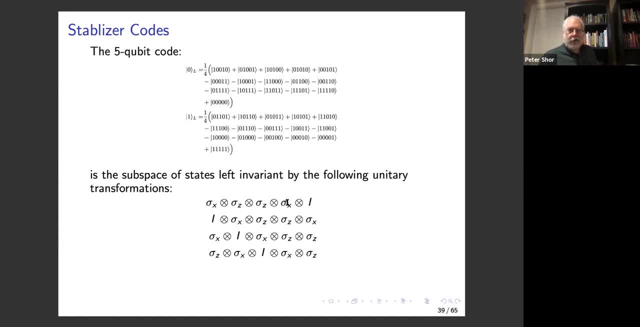 And these commute, because I don't think I told you it- but Sigma I and Sigma J anti-commute if I is not equal to J. So if you look at this and this, they differ. i mean, there's a sigma z and a sigma x here and a sigma x and a sigma z error. 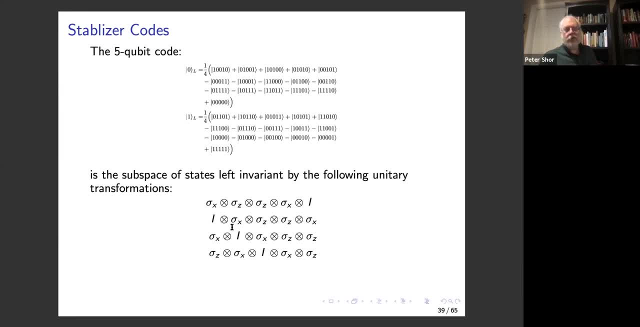 so this position anti-commutes and this position anti-commutes and you take the product. that means minus one times minus one equals one. these two things commute, and the same is true for any pair here. so that's how you get a general stabilizer code. you find a set of, you find a stabilizer set. 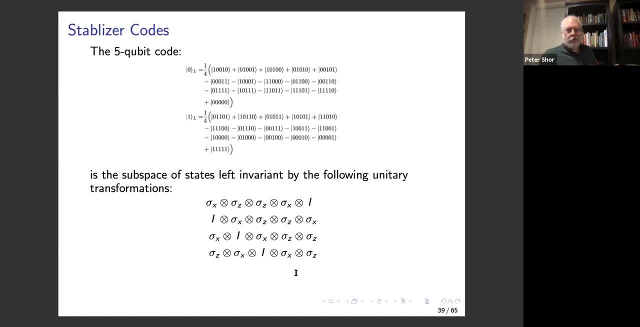 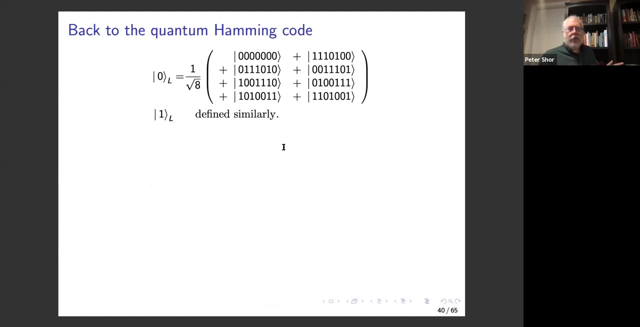 which is these things, and that they all commute, and then you find the simultaneous eigen space of those. okay, so we can ask: well, back to the hamming code, is that a stabilizer code? and the answer is yes, and in fact- um, i screwed up here- there should only be three of these, um. 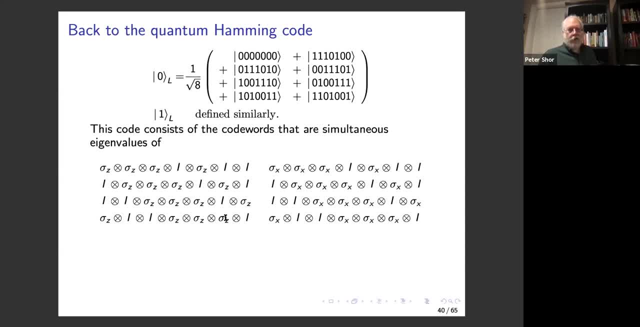 simultaneous code words and not four, because it turns out the fourth is a product of these three, some product of um two of i believe the fourth is a product of two of these three. so the code consists of code words that are simultaneous eigenvalues of these six um. 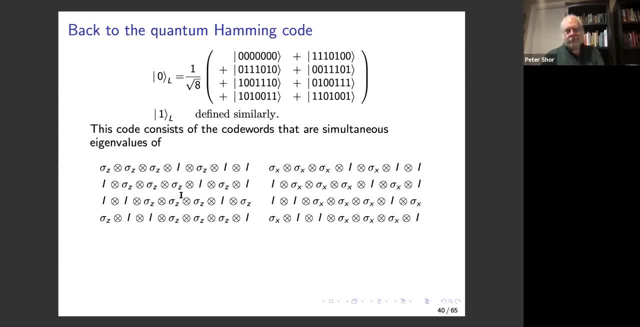 operators and you know you can go up and check that these leave all of this space invariant. for example, if you apply sigma x to the first, second, third and fourth, let's apply a sigma x to the first, second, third and fifth of this. that's one one one, zero one. so one one, one, zero one is a state here. 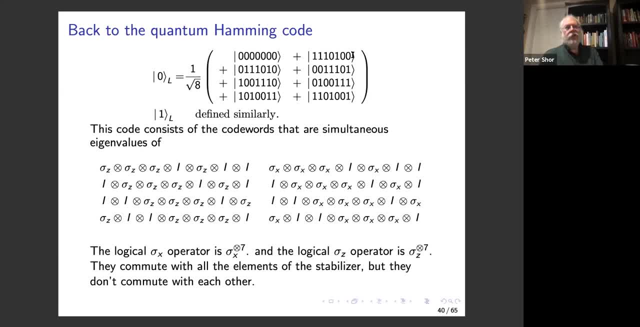 so it's easy to check that the state of the variable is the same as the state of the variable. okay, the this code is the: gives the subspace that's left invariant by this um. the stabilizer set so the logical, and for this code there's a logical sigma x, zero, and it's just the product. 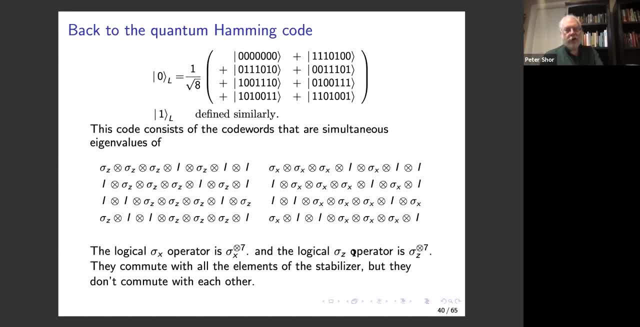 of all sigma x's and the logical sigma z operator is the product of all sigma z operators and they commute with all elements of the stabilizer, but they don't commute with each other, which means that one of them applies a sigma x to the um, one of them applies a sigma x. well, they're applied. two: 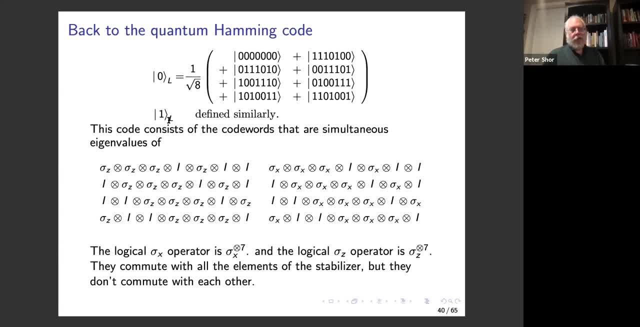 operators to the original two qubits and they're non-commuting operators. and it turns out that if you write the two, choose the proper um basis for this code word, for this code space, for this space of code words, you can make a sigma zero and a sigma. 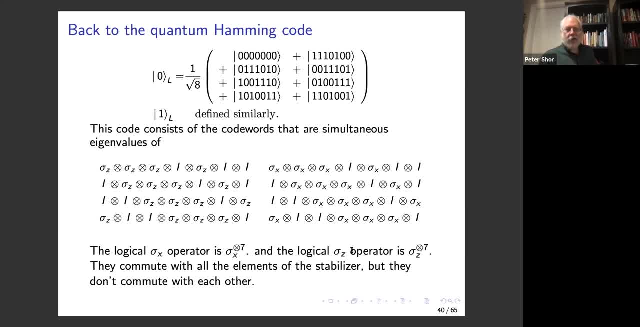 one and have the logical sigma x operator and a logical sigma y, z operator operate on these. and the proper way. so just having, uh, having things. if you look at things that commute with all elements of this system X stabilizer set, then you get the logical Sigma X operators. 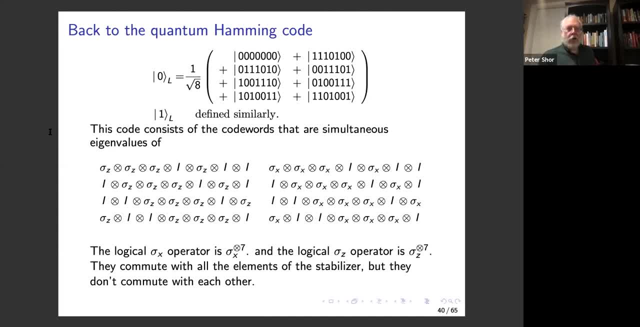 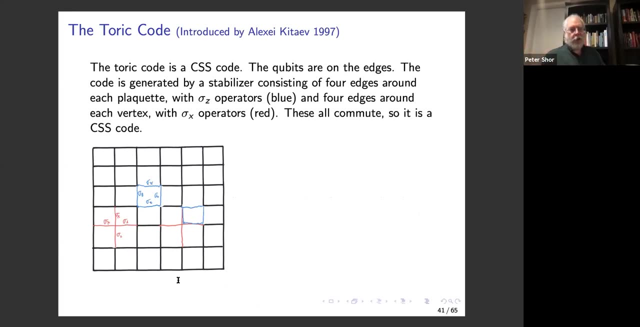 and the logical Sigma Z operators on the original, on the code words or the logical qubits. Okay, so now I want to go into the Tauric code. So I mean, my goal in this talk is to explain all the things that go, or at least a lot of the things. 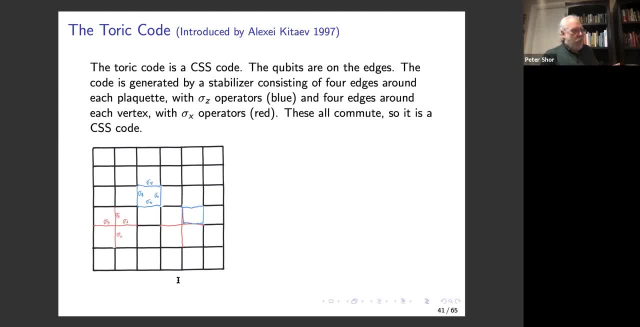 that go into the current best way we know of of doing fault tolerance on quantum computers, And that is using Tauric codes. or rather, we're using surface codes And the surface code is actually a variation of the Tauric code. 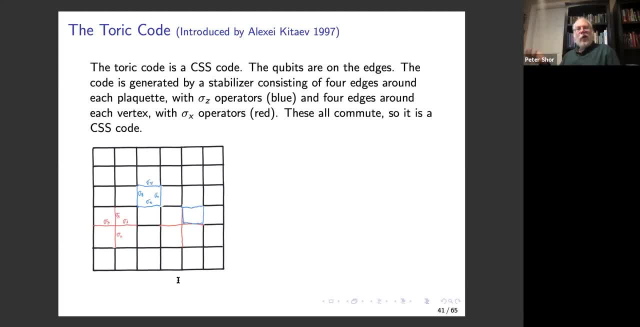 And the Tauric code is actually the first topological quantum code to be discovered. It was discovered in Alex Kuhn's in 1997, and he, you know he discovered more of this type of code later. but this well okay. 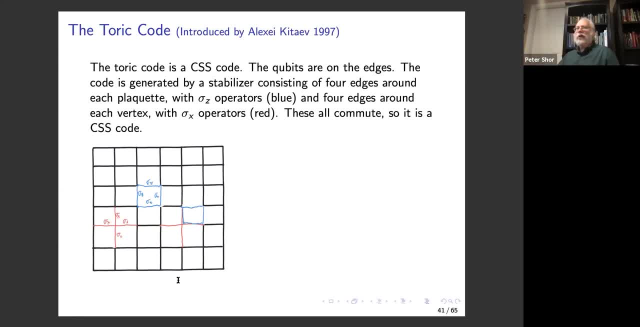 So surface code is not a Tauric code. It's a very simple variation of this Tauric code And I explained the difference. but the Tauric code is the easiest thing to work on, And so the Tauric code is a CSS code. 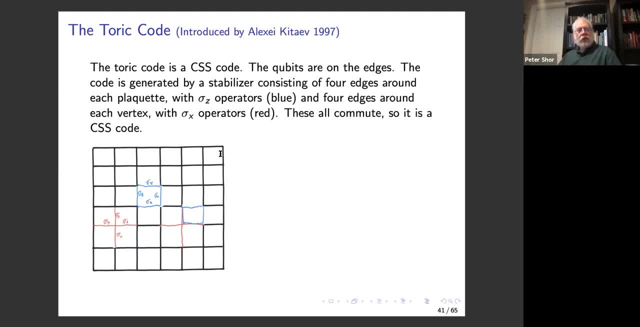 You have a Taurus here, which means we want to, let's identify the edges on the left and the right here, and on the top and the bottom. So the Tauric code is generated by a set of commuting stabilizers. And what are these commuting stabilizers? 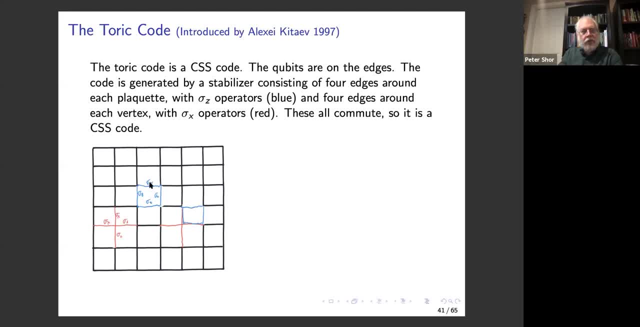 Well, one pair, one set of stabilizers is a Sigma Z, on all of the edges of these faces, of this tiling Which is called, which this is called a Placket, And the other set of stable stabilizers is the Sigma X. 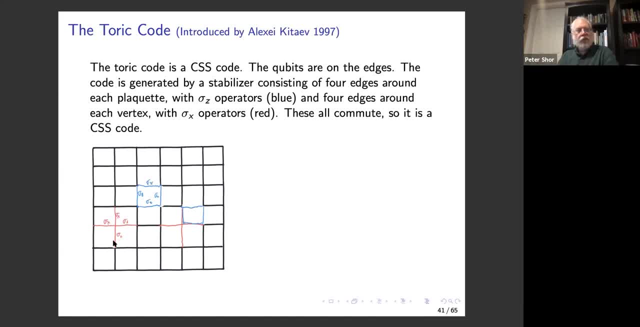 on the edges originating out of the vertex, And I'm going to draw Sigma Z operators in blue and Sigma X operators in red So you can tell them apart, Because my Zs look exactly like my Xs when I handwriting them. So you don't, you can't necessarily tell them apart that way. 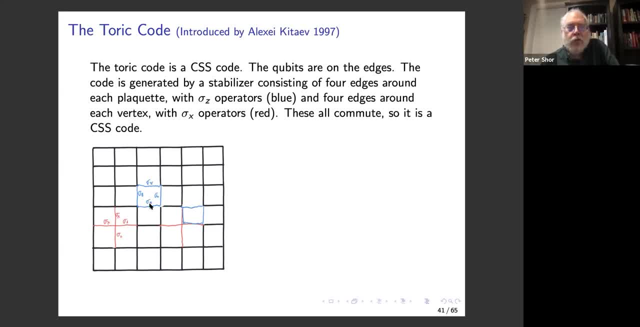 especially because these are so small, And so the Zs and the, so all of these operators commute. I mean they're, why do they commute? Well, if they're all Sigma Zs, they naturally all commute, because two Sigma Zs commute with each other. 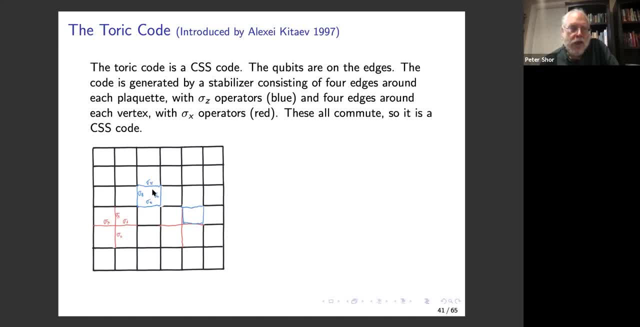 If they're, if the two- I thought Placket operators, they're all commuting- Placket operator and a Vertex operator are on disjoint set of edges, Then they automatically commute. And the only other here just a second. Yeah, so I I guess we moved my table last night. 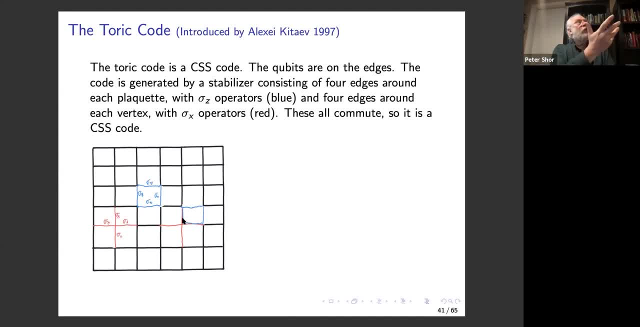 and right now. so these, these? yeah, So my lights are on timer. The basement lights are the timer. Okay, We've moved these tables So I'm behind a pillar from the timer. So now the lights seem to go off if I wait for too long. 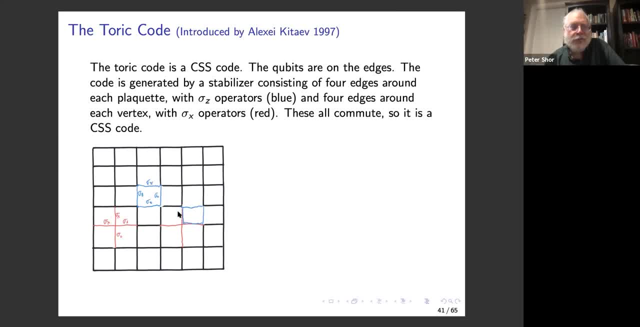 So I'm going to be doing this every so often in the talk to keep the lights on. Sorry about that. Anyway, what were I saying? So the only case where the Vertex operator and a Placket operator are overlap is in this case where the Vertex operator Placket operator. 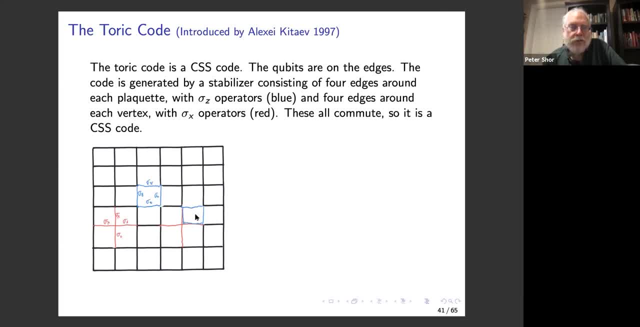 two of the: the Placket operator fixed into a nice corner of the Vertex operator, And now there are two edges that overlap and you know, Sigma X, Sigma Y equal Sigma X, Sigma Z equals minus Sigma Z, Sigma X. So these commute as well. 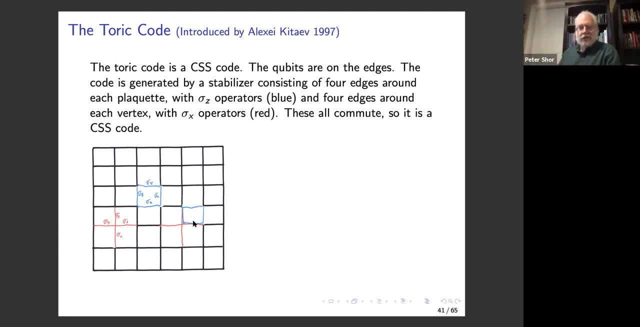 because they overlap in two edges. So these all commute, which means it generates the CSS code And you can ask: how many keys do you want? So you can ask how many keys that's gonna Allison. that's gonna be the last question. 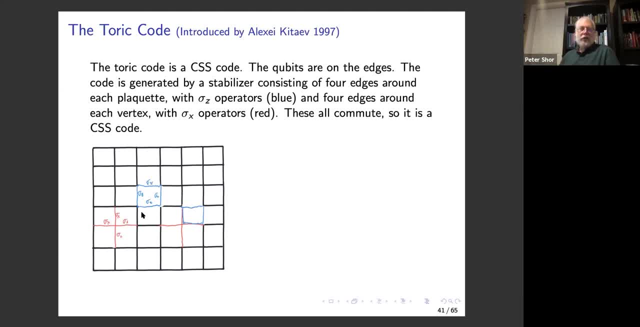 Qubits doesn't encode, And one way of getting that is figuring out the number of operators, which is n? squared minus two or two. n squared minus two, because there's only n? squared minus one independent plaquette operators, because if you put one on every square, then you've covered every edge twice, so their product is one. 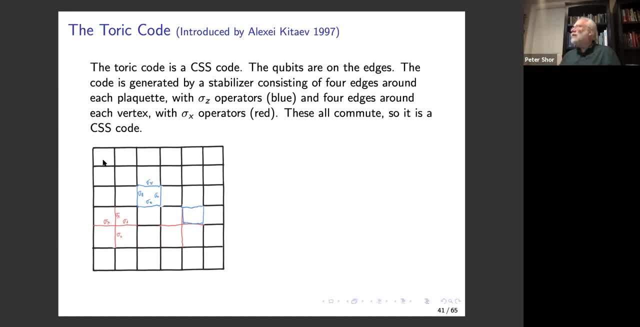 So there's one degeneracy in the square ones and also one degeneracy in the vertex ones, And so that means that and there are two n squared edges, so that means there are two qubits that are encoded. Okay. 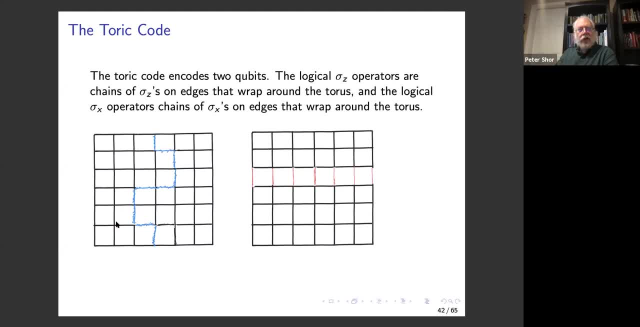 So what are the logical z operators and what are the logical x operators? Well, the logical x operators are just a chain of edges going around the torus. So you can see that if you have a chain like this, there are two blue squares. I mean it overlaps with zero or two edges with every square and they commute with the vertex operators because they're all sigma x's and here you have a chain that goes down. 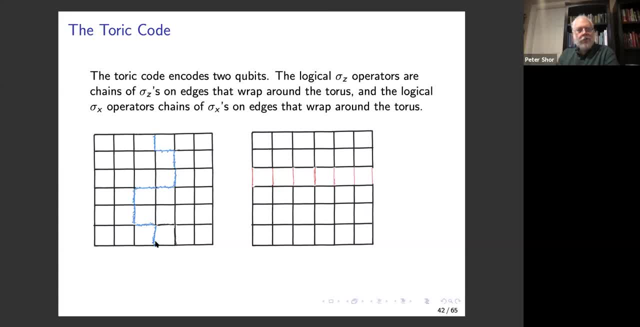 or that wraps around the square vertically, and this is a sigma z operator applied to the qubits, and you can see that any vertex operator overlaps this chain wrapping around in two edges and that means it commutes with it. So these two things commute. 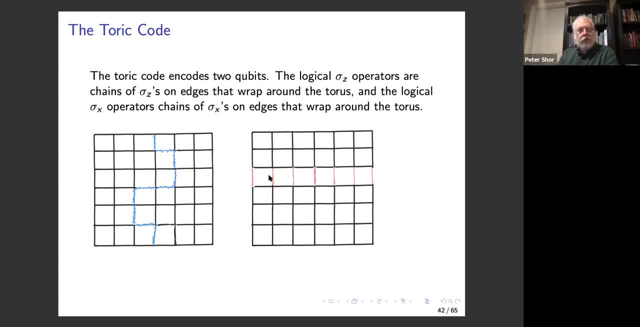 They commute with every stabilizer operator, but they don't commute with each other because you know, if you have a vertical chain and a horizontal chain, they overlap at one edge, so they anti-commute. So this is a sigma z applied to one of the qubits and this is a sigma x applied to the same qubit. 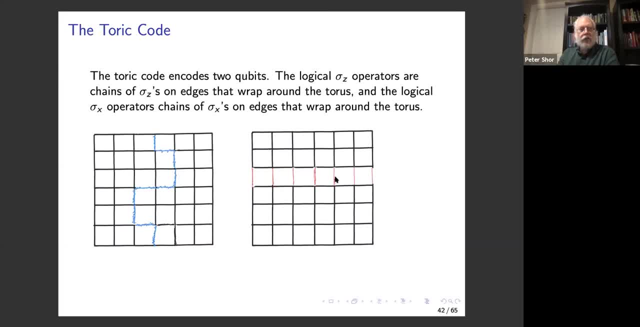 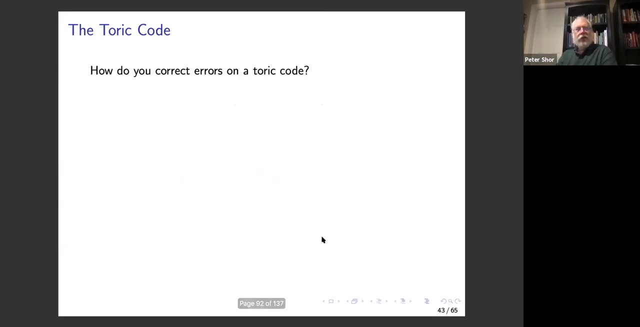 And let's see. And of course, the other two logical operators are sigma x going across and a sigma z going down. I'm sorry, a sigma z going across and a sigma x going down. So you can ask: how do you correct errors on a Toric code? 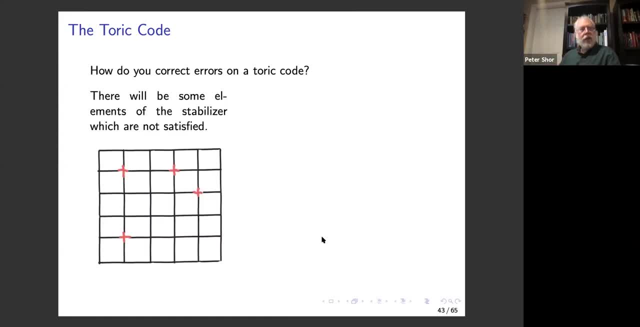 Well, there will be some elements of the stabilizer which are not satisfied. So, to correct errors on a CSS code, you measure all these stabilizer elements and figure out which ones give you. you know, find the eigenvalue of each of these operators, and some of them are going to be one, in which case this, the state, satisfies that one, and some of them are going to be minus one. and 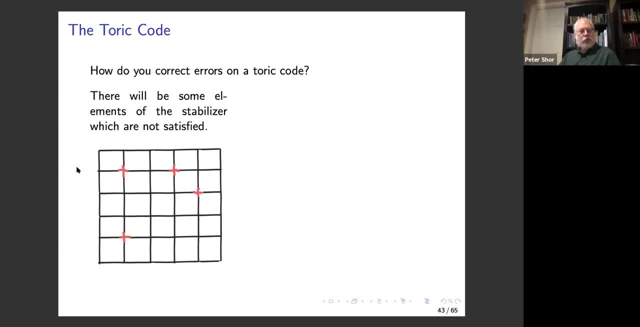 the minus ones are the ones that aren't satisfied. So you find all the ones that aren't satisfied And I'm just assuming that these are all vertex operators here to make things easier. You know, plaquette operators are exactly the same, except you take the dual graph. 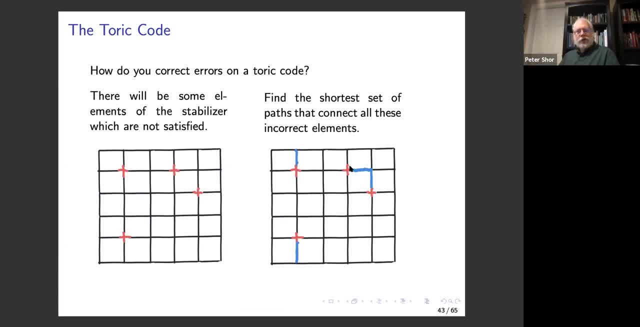 And now you find the shortest set of paths that correct all these incorrect elements. So if you applied sigma z to all of these two, you know, to these two edges well, an anti-commute attributes with this thing. So now, after you've applied this, this operator will be stabilized, And it similarly for this operator. so if you apply sigma z path connecting these incorrect vertices, you will have figured out the, you will have corrected the state to a state that's now in your CSS code. 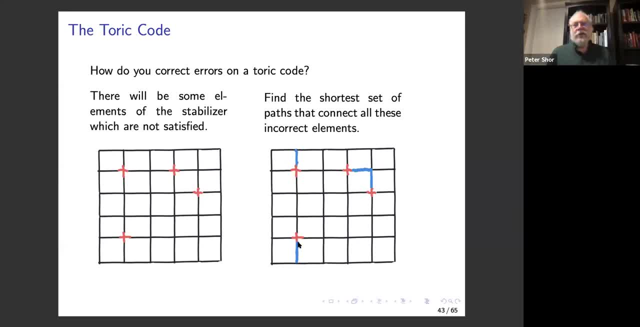 And the only way you can correct it to the wrong code word is if you do something topologically different. So, instead of wrapping around here, which would have corrected two errors because there's an error on this edge, an error on this edge, if you corrected the, if you applied it along this edge. 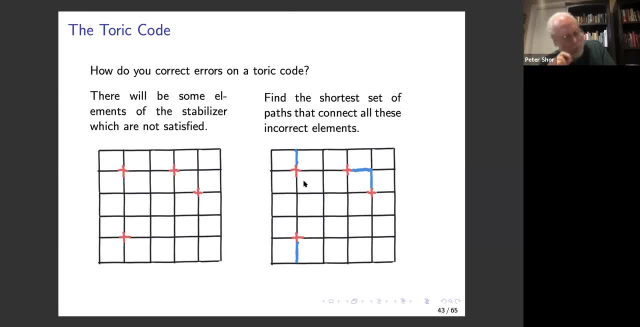 on this path which is correct, three errors. then you would have corrected it to a code word which has a sigma z. well, you get one code word if you correct it going up, and a different code word if you correct it not crossing the thing. 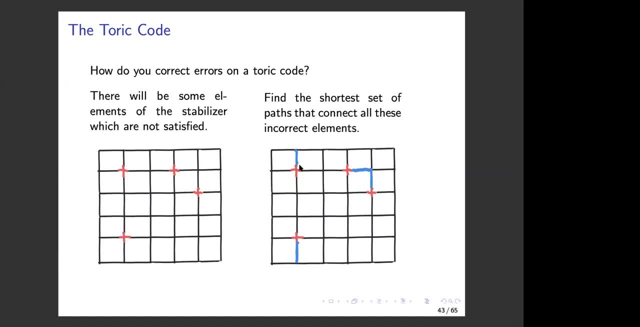 So that means that you get. so that means that If you correct it, you can correct this two different ways, depending on whether you wrap around or not, And those give you two different code words. So the only way you can correct it incorrectly is if you accidentally wrap. apply a wrapping around on your different edges. 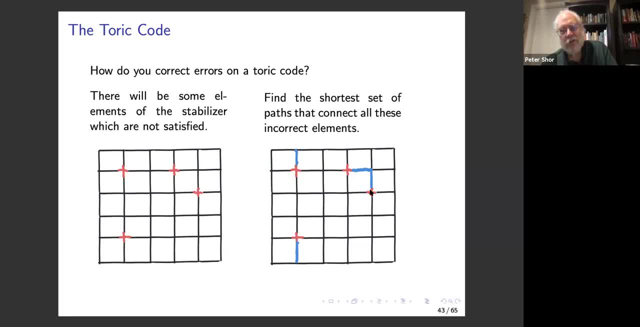 So if you corrected this error by using these two edges- you know down and across rather than across and down- you would have Corrected it to the same code word. So what you do is you find the shortest set of paths that connect all of these incorrect vertex operators and then you apply that, And if you have a large square and not too many errors, that is almost certainly going to be the right correction. 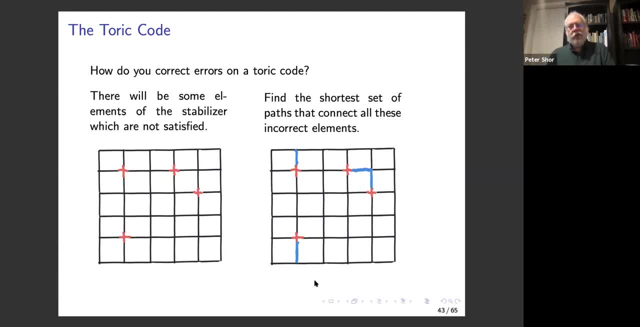 So now we can ask: how many errors does the Torrek code correct? Well, I mean it has two N qubits You need to apply, have an error that hits N edges to actually change it from one code word to a different code word, because you need to wrap around, which means it corrects this number on its own, and then you crack down an N. 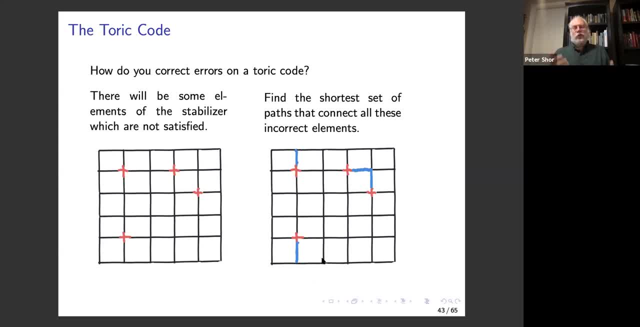 Because you need to wrap around, And so you ended up, Which means that it corrected this error. Okay, If you have error which has less than one half n edges incorrect, then it will always correct it to the right code word, which means that the distance of this code is order of square root of the number of cubits in the code. 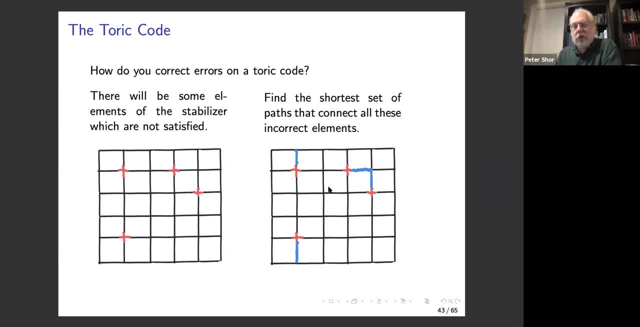 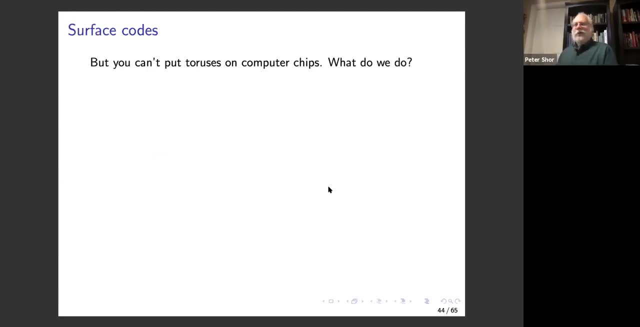 So the Toric code is pretty good because square root of n is a fairly large number. if you have a large Toric code, Okay. Well, yeah, you have a question. We have a question from the audience, which is that the Toric code seems robust, but is it also efficient or fast enough? 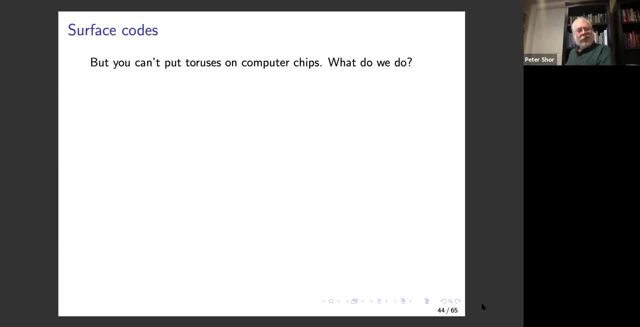 Well, That's a good question. So right now, well, there's a problem with the Toric code, but we can fix that with surface codes, which I will get to. But right now the best way we know of to correct errors on a quantum computer is use Toric codes. 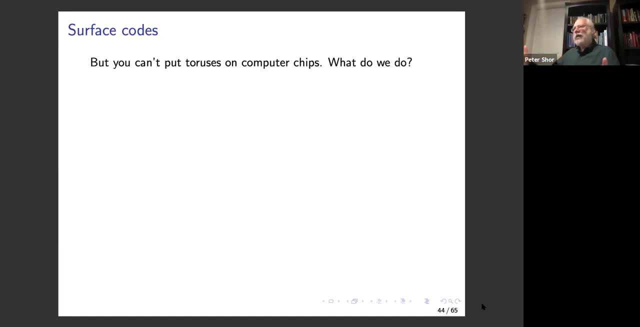 But you know this is inefficient because suppose you have a seven by seven squares To encode one qubit. you need two times forty-nine physical qubits to encode one logical qubit, which means you need- you're blowing up the number of qubits you use by a factor of a hundred. 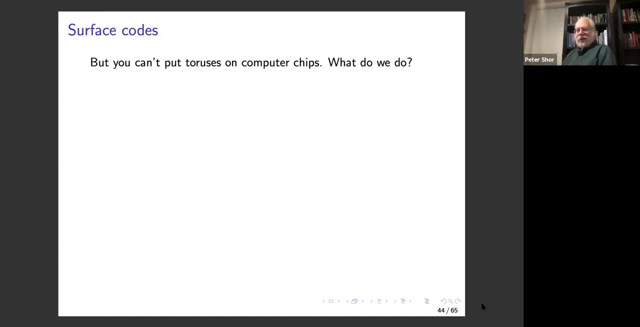 And we would really rather not do that. So yeah, Toric codes are good in that they have large distances, but they're bad in that they waste space. But the worst waste, the worst waste of space, is in terms of magic space, which we will get to later. 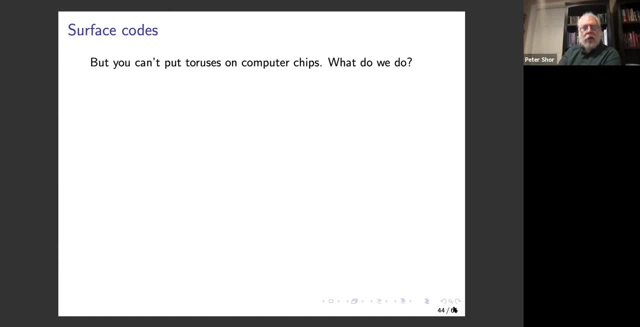 But you can't put toruses on computer chips. So what do you do? Well, okay, come on. What's wrong? Here we go. Well, instead of a Toric code, you can use a rectangle where the edges don't wrap around, and you have one smooth edge. 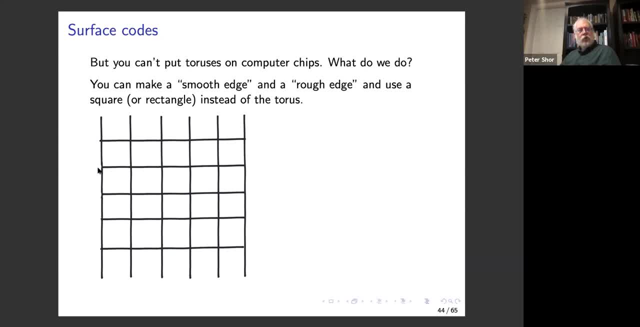 That's this one And one rough edge, And that means that your logical operators are sigma x's or vertex operators, a chain of vertex operators going horizontally across this thing And a chain of platet operators going vertically, And I won't go into the details of that. but this will encode one qubit in roughly exactly the same way that qubits were encoded in Toric codes. 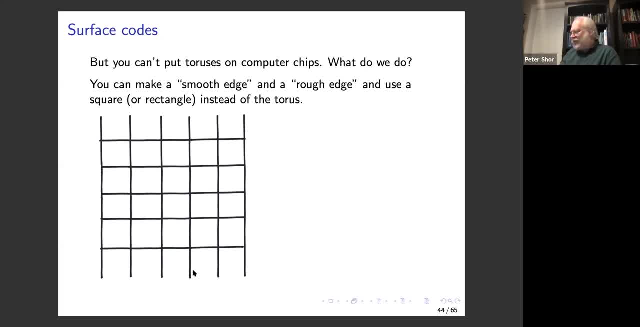 And this surface code is, are small variations of the surface code, are the- you know- current code that people use when they're- I mean so right now we're in quantum computers are too small to actually have quantum error correcting codes work on them. 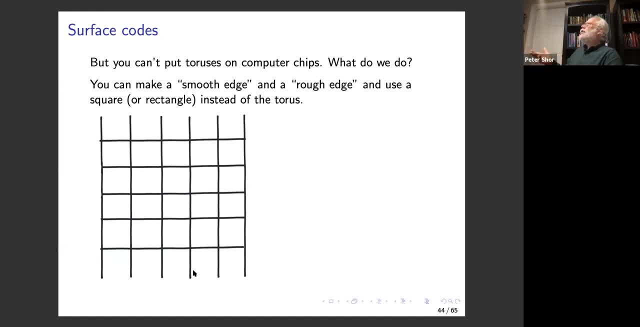 Because the biggest biggest quantum error correcting code in the world, The biggest quantum computer we built, is 60 something qubits And if you're using a surface code You basically get to encode one or two qubits that way, But when they're- you know, designing hypothetical large scale quantum computers, they use the surface code. 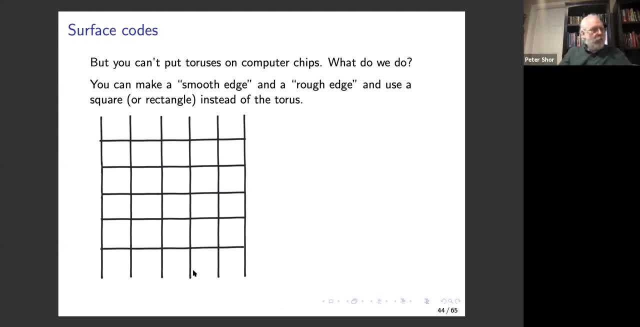 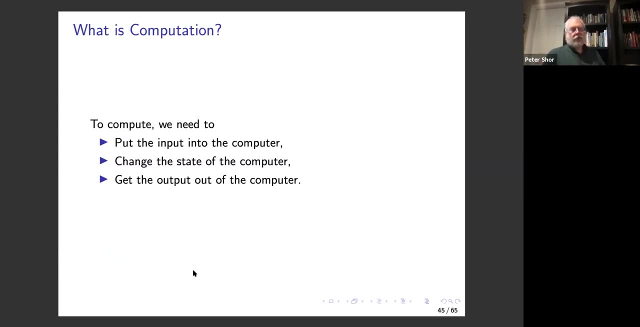 So Now I want to switch topics and talk about actually How do you do computation on a computer, and I see I'm going to run out of time So I will try to go through the next part A little bit quickly. So to compute, what we need to do is first you need to put the input into the computer, change the state of the computer and get the output out of the computer. 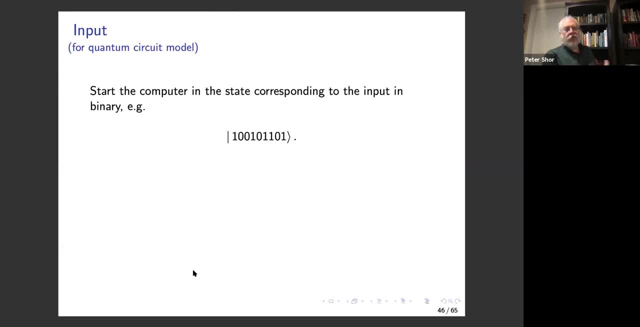 So input? well, the model- quantum circuit model- is you just start the computer in the state corresponding to the input in binary. And you actually might, in fact are very likely to need extra workspace in the algorithm, which means you start the workspace in the state of all zeros. 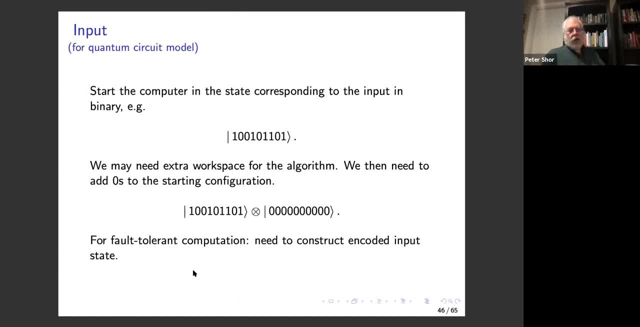 So that's straightforward. And for quantum computation you need to instruct, construct encoded input states. So instead of this 10010, you will need to construct the Logical zeros and logical zeros, And then you need to construct the Logical ones in a surface code. 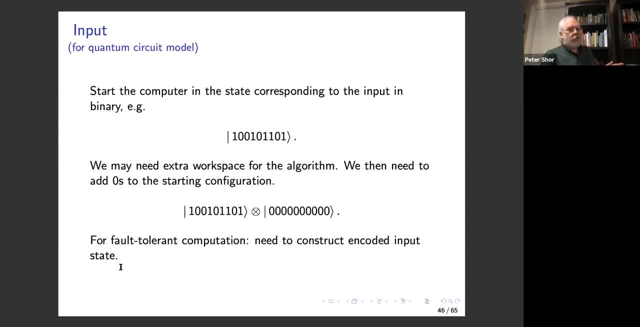 And That's not. it's not completely obvious how to do that, but I'm not going to talk about this in my talk because I'd run out of time. And the more interesting part is in the actual computation For output. Well, at the end of the computation the computer is in some quantum state. 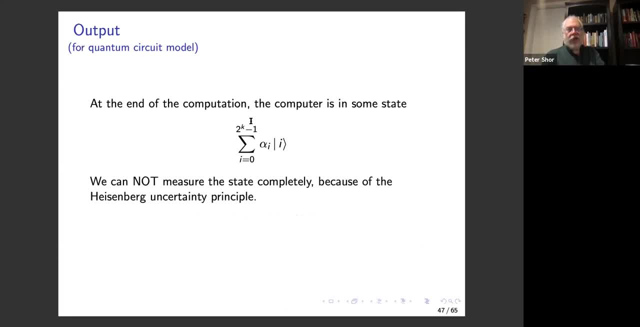 And We have a Heisenberg uncertainty principle. We cannot Assume that we measure Output i's, which are the Amplitudes in that quantum state. But what we're going to do is we're going to assume that we measure in the canonical basis. 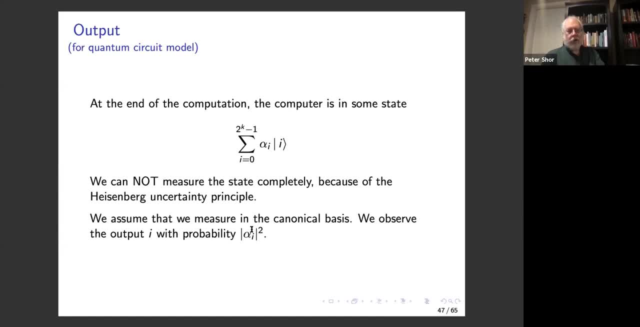 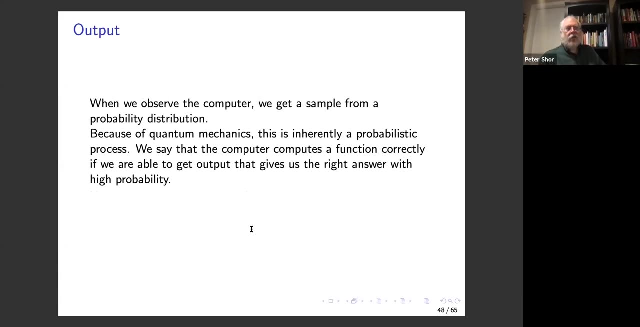 So what that means is: we'll observe output. I with probability absolute value. Alpha is the by squared. This is the Quantum mechanical, No Way that measurement works. And so when you observe the computer, You just get a sample from a probability distribution. 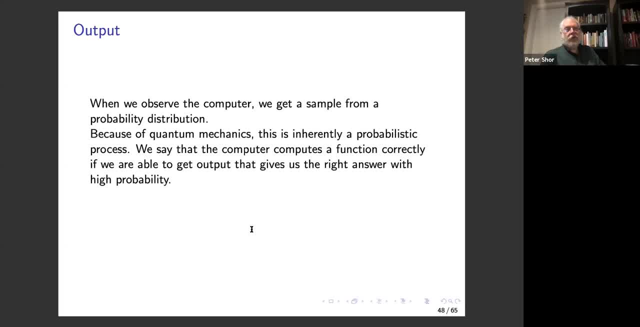 And what we want to do is: we want to make sure that the computer Computes a quantum state, Which will give us The answer to the question we're Asking with high probability When we measure it, And for Quantum computation You need to measure the encoded output space. 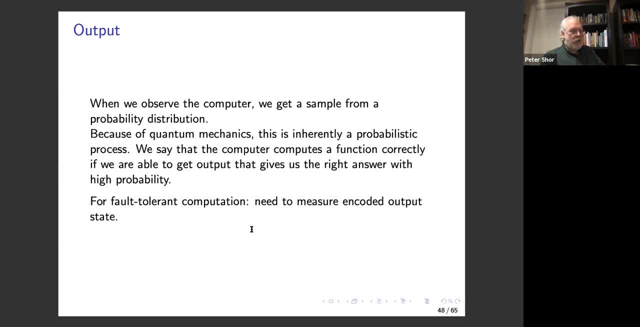 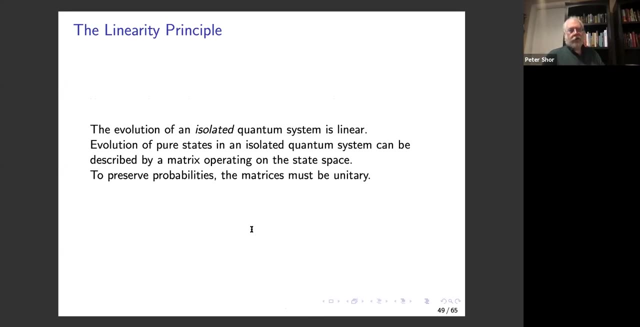 But that's really is Immaterial, Because if you made The encoded output State You can easily deduce the actual output state from that. So The linearity principle says the evolution of isolated quantum system is linear And that the 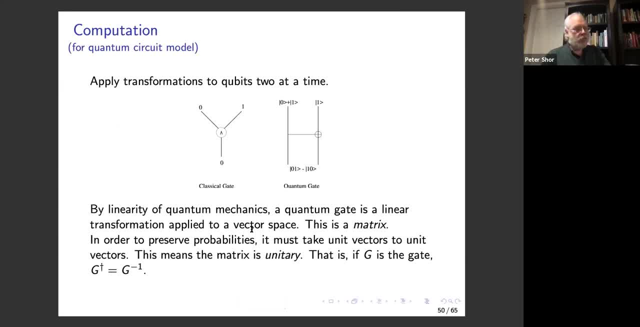 Quantum gates are matrices. So in our quantum circuit model What we're going to do is we're going to apply transformations to qubits, two at a time. So classically You can get any Function By decomposing it to ends and knots. 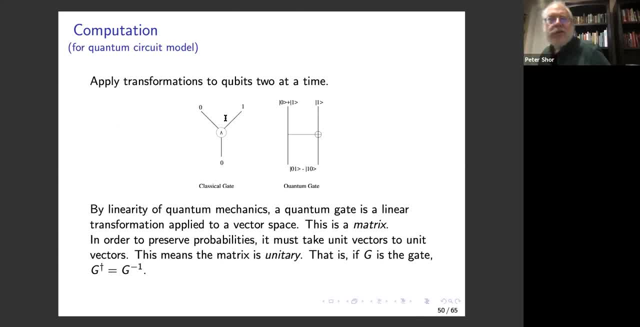 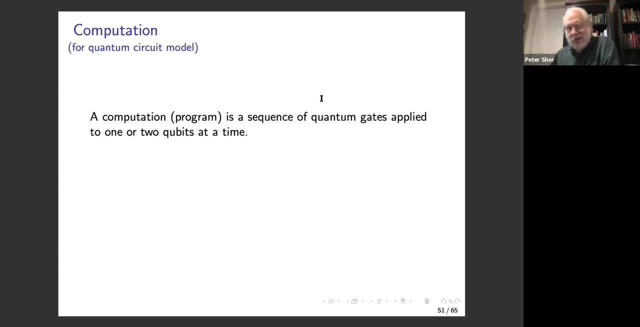 So you just need and gates and not paints. So the same is true for Quantum gates. So this is a quantum gate called a CNOT. And Okay, I am Getting ahead of myself here. Computation Is a single function. 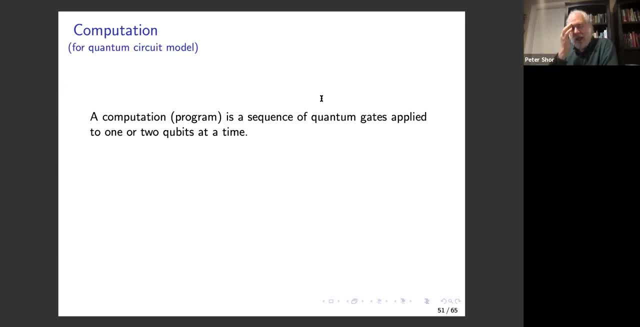 Right computation is a sequence of quantum gates applied to one or two qubits at a time. And why do we choose two? Well, three doesn't give you any more power and it's more complicated due to experimentally and arbitrarily many qubit gates are hopeless experimentally Now. 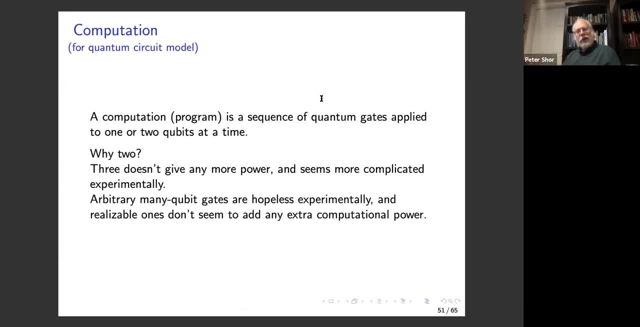 it's quite possible that you can realize some many qubits gates experimentally. but the ones you can realize can be broken up into a sequence of a reasonable number of two qubit gates, so they don't seem to add any extra computational power. So our quantum computing. 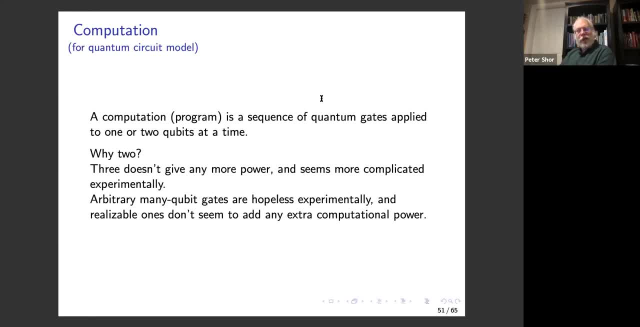 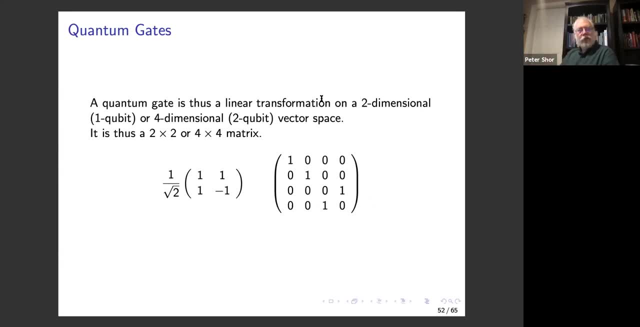 circuit model. we assume you do two qubits gates. apply gates to one or two qubits at a time. Now a quantum gate is a linear transformation on a one-dimensional space or a two-dimensional space, so it's a two by two or four by four matrix. 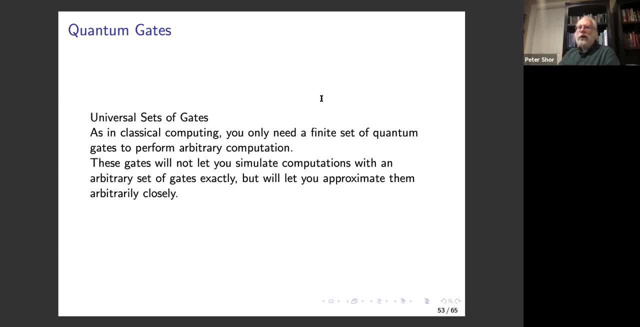 And, as in classical computing, you only need a finite set of quantum gates to perform an arbitrary computation. And well, these gates will not let you simulate computations with an arbitrary set of gates exactly. and that's easy to see because there's a countable. 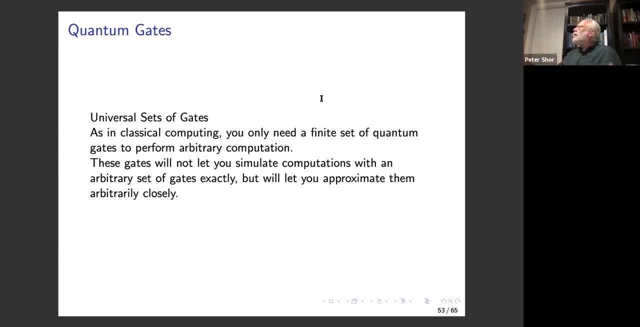 number of sets of gates. If you have a finite set of gates, you can apply, and there is an uncountable number of unitary matrices. But in fact this set of gates will let you simulate computations with an arbitrary set of gates arbitrarily closely. So that's good enough. 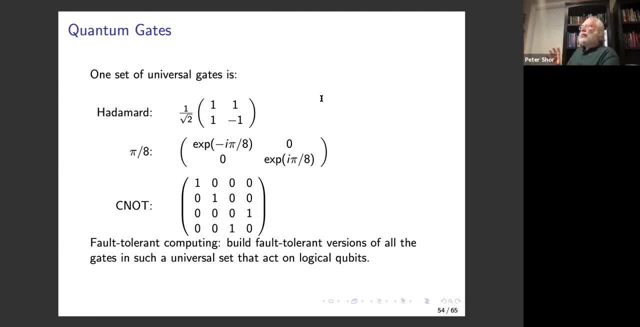 And in fact you can show that this doesn't take that much extra overhead. to simulate arbitrary gates with a finite set, And one set of universal gates is this set. So if, for fault-tolerant quantum computing, what you do is you build fault-tolerant versions, 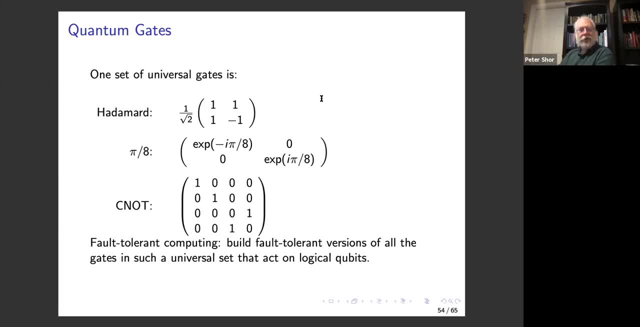 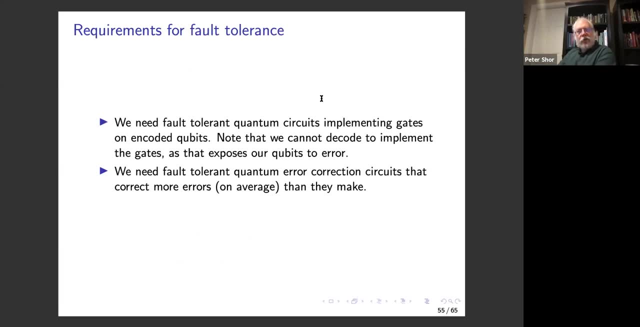 of all the gates in a universal set that act on magical qubits. So what we need is we need fault-tolerant quantum circuits to implicate gates on the encoded qubits, And the problem is that we cannot decode the encoded qubits implement. 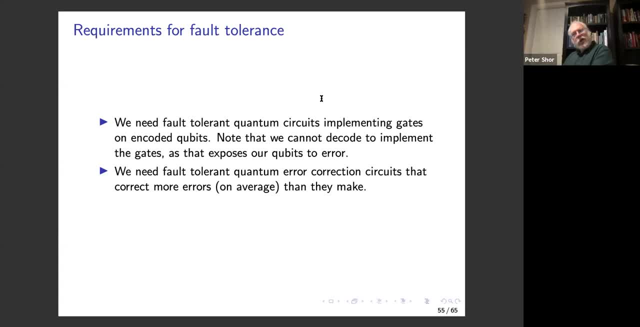 the gates and then re-encode them, because once you've decoded the qubits you're exposing them to error, And a single error- which is not all that unlikely on an unencoded quantum state- will throw your entire computation off. So you need to keep your quantum bits. 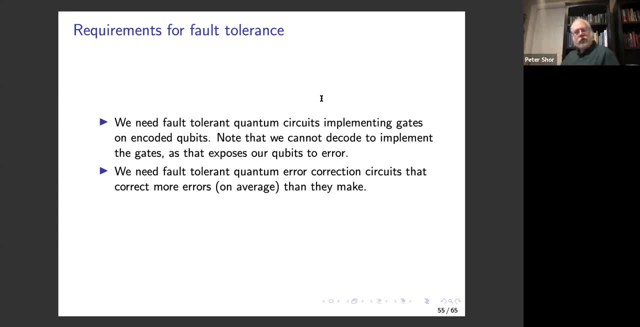 or your logical qubits encoded while you do the quantum circuits on them. And the other thing is that we need the fault-tolerant quantum error correction circuits that correct more errors on the average than they make, Because when you're trying to correct errors, you're obviously going to make a few errors. 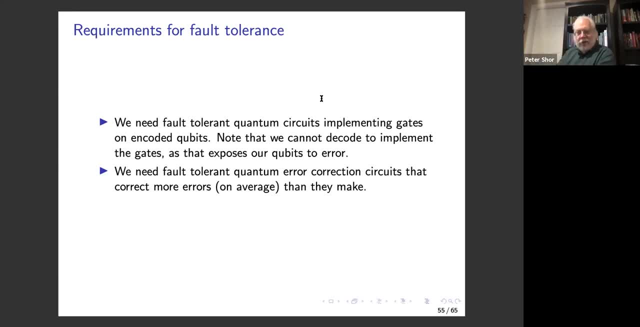 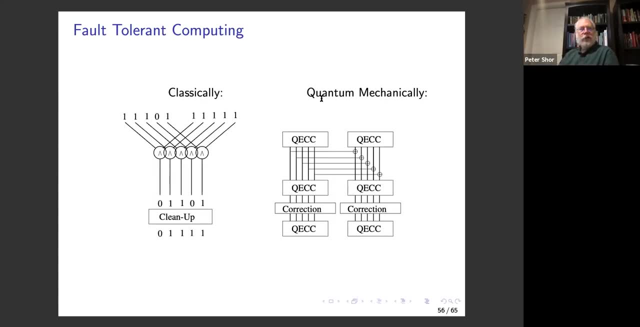 in your correction error thing if you have faulty gates And so you want them to correct errors faster than they make more errors. So what do you do classically? Well, classically, what you do is you take your repetition code. So this is von Neumann's algorithm. 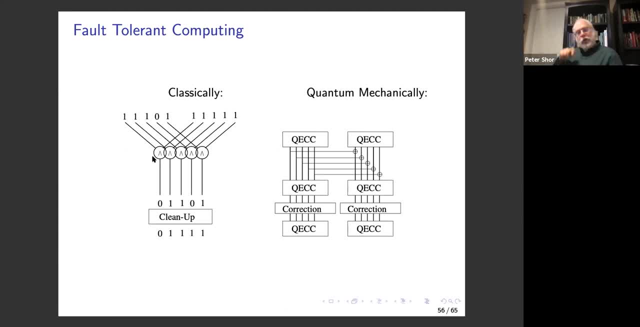 For quantum, fault-tolerant quantum computation And if you're doing an AND, you just do an AND gate on these things in pairs And you'll get a few errors because you had errors in your original input. So this 0 goes down and gives you a 0 in the AND And you might make 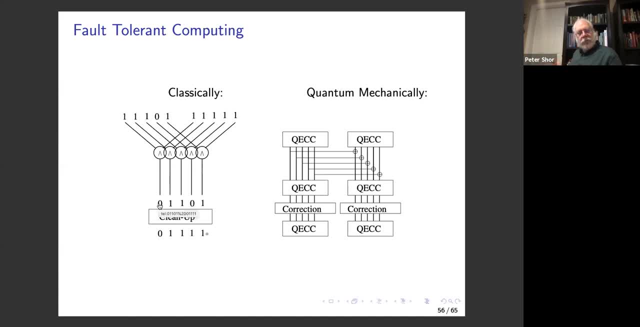 an error in this gate, in which case you will get another 0. And now, after this, you go through a process Where you clean it up. So you basically take the bits in threes and do majority, And that will catch most of the errors, Although it might miss a few and it might introduce more. 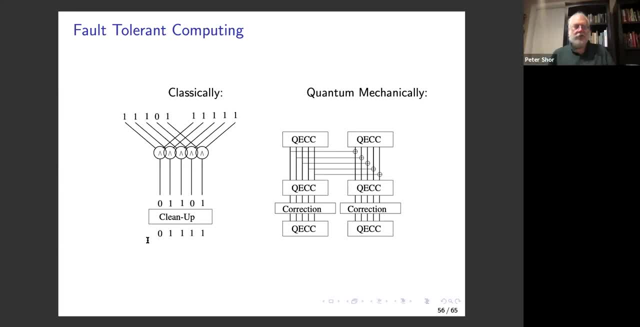 But on average it will correct a lot more errors than you originally had. So if you make a computation fault-tolerant this way, it will correct a lot more errors than you originally had And it will probably give you the right answer with high probability. 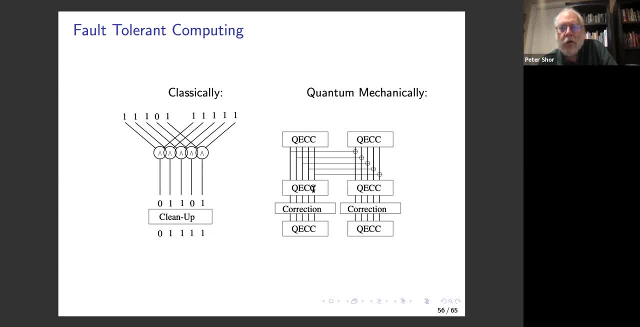 So quantum mechanically you have quantum error-correcting code And here is an example of a traversal fault-tolerant gate. So this is a control knot And you can do a control knot to each qubit of your encoded state and get a control knot on the qubits. 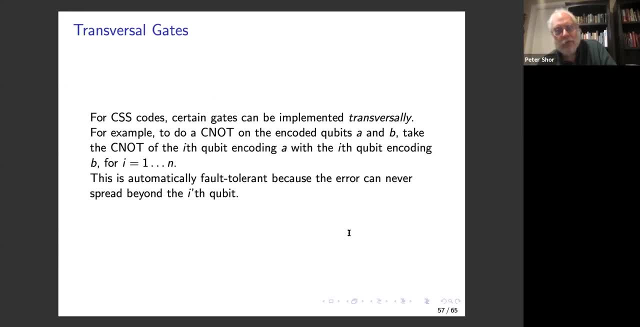 And the nice thing about transversal computation is that they're automatically fault-tolerant, because if you have an error in the ith qubit of some code, if you do transversal computations, it will never spread beyond the ith qubit in any of your encoded states, Which means 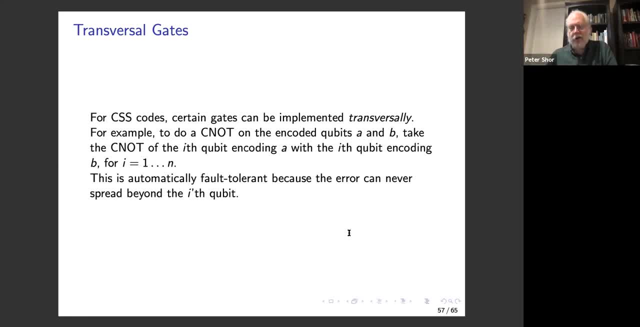 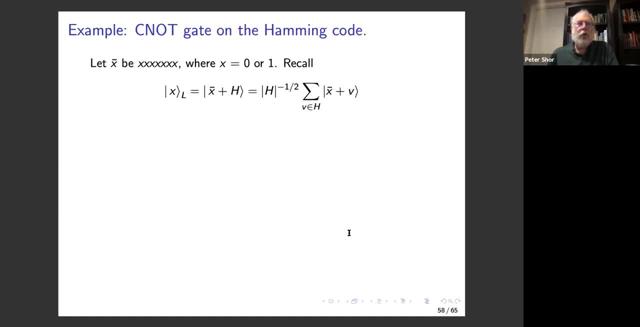 that you will never have more than a one qubit error, an encoded k state, and you can assume that we can fix one qubit errors. so, um, here is how a truck. here is how a c not works in the hamming code. here's: let's let x bar be all x's. so the hamming code was: um, you know, you took the. 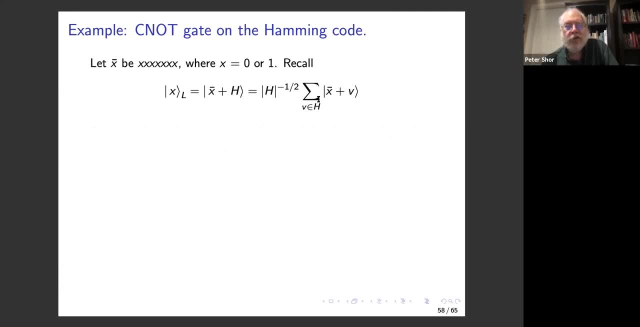 cos you took the superposition of everything in the coset, which is this. and now, if we do a transversal c not gate, what you're doing is a c not gate. you're applying a c not to every um bit, to the, to the i-th bit of this quantum code and the i-th bit of this quantum code, and that means 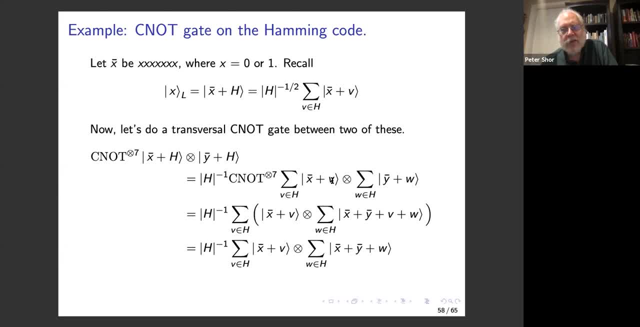 that if this is x plus d, it's going to be the same as the i-th bit of this quantum code, and this is y bar plus w. we get here when you apply a control knot: x bar plus y power plus v plus w, and now x bar plus y bar is the thing we're trying to do, because that's the c, not of. 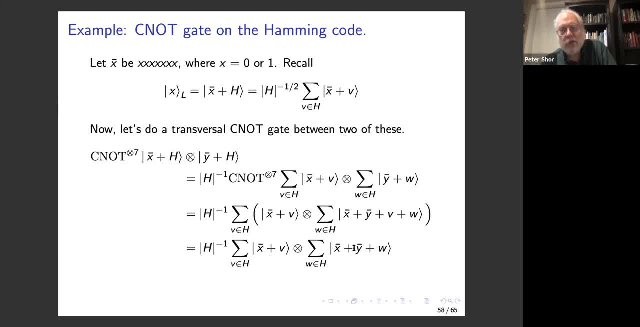 x bar and y bar is x bar and x bar plus y bar, and we have a v plus w here, summed over all w in the in our um sub. well, in our um subgroup, and because it's a subgroup, if you take v plus w and sum over all w, 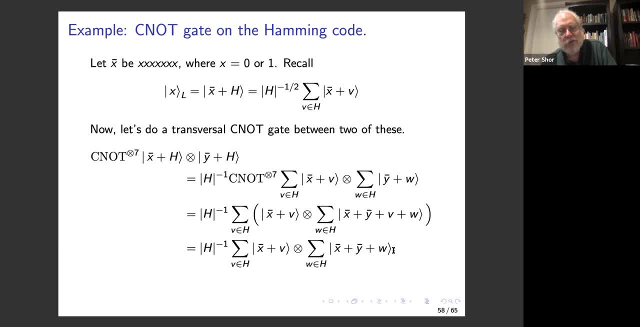 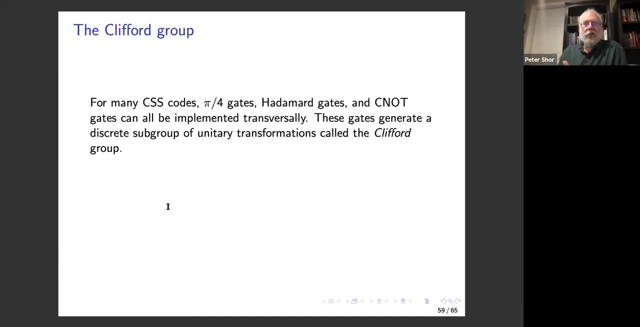 it's the same thing as just taking w and summing over all w, so this does a transversal scene. this applies a c knot to the logical qubit here and the logical qubit here and for many css codes. they can all be implemented transversally and these code generate. 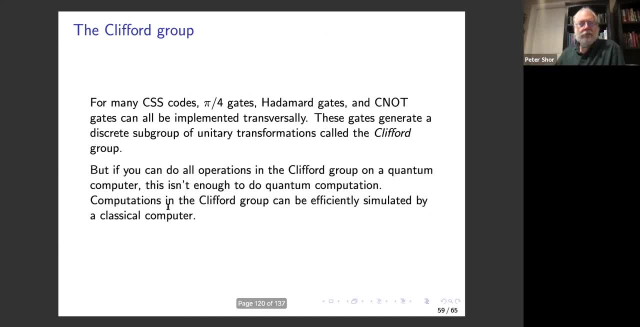 discrete subgroup for the unitary transformations called the clifford group. but doing everything in the clifford group on a quantum computer isn't enough for doing quantum computation. you need to do um some quantum gate that isn't in the clifford group and um let's skip. 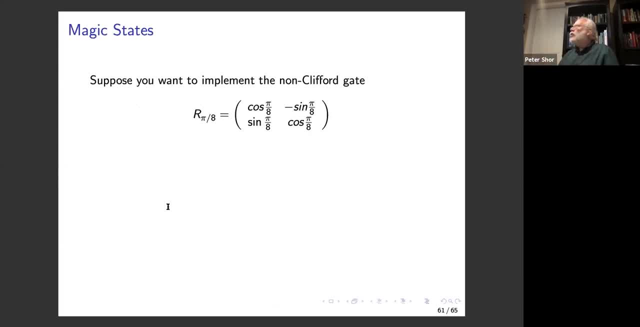 означating the Austinenzams. end the code, like we are empty because of the vocalization module. and and um are good quantum state one that's not in the clifford group, and you want to create the state which is called a magic state, cosine pi over eight zero plus sine pi over eight哪裡 poner? 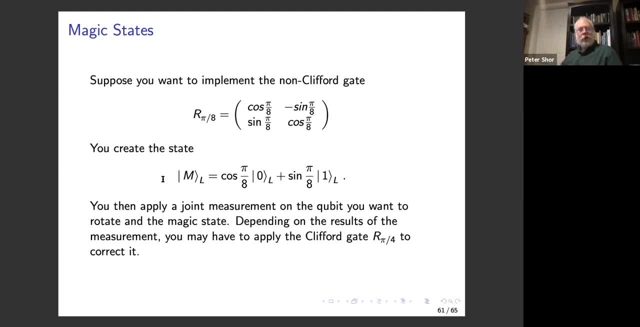 democrats. you can apply it transversely to both the qubit you want to apply the gate on and this magic state And then, depending on the results of this measurement, you may have to apply rotation pi over four rotation to correct it. because what happens when you do this? 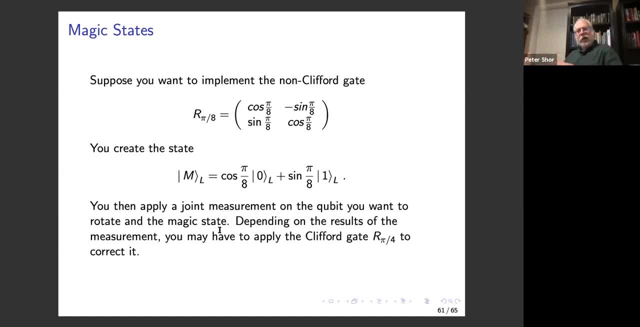 is it either rotates it by pi over eight to the left or pi over eight to the right. And if you rotate it by pi over eight to the left, then you have to rotate it by pi over four to the right to get your desired thing. 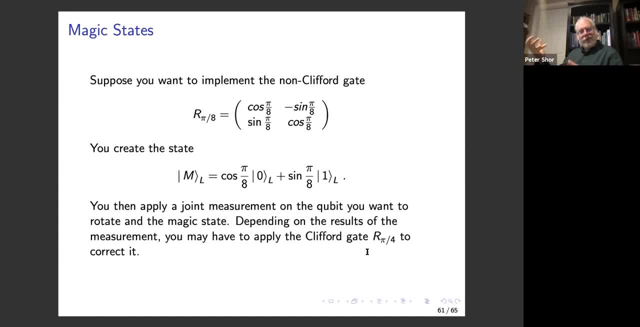 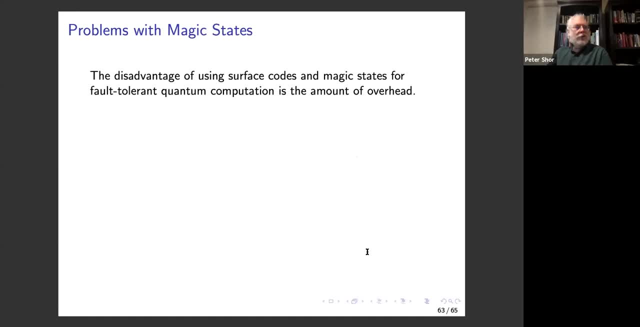 But the pi over four rotation is in the Clifford group so you can do it. So that's how magic state works and how you create the magic state. I do not have time for that. And what's the disadvantage of using surface codes and magic states for fault-cognitive computation? 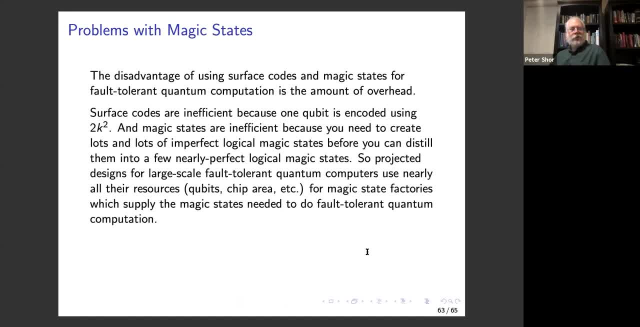 is the amount of overhead, And the problem with using magic state computation is the way you create these magic states is you take seven states that are close to a magic state and then you do a joint measurement on all of them and you get one state that's even much closer. 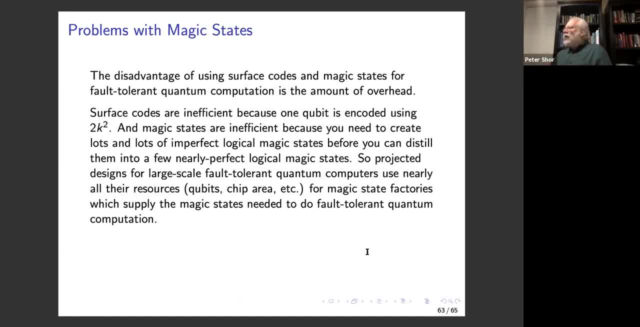 to the magic state you want. So you have to create lots and lots and lots of approximate magic states and then distill them into a few very good magic states, And then you can use the magic states you've distilled to do real computation. And that means that on your 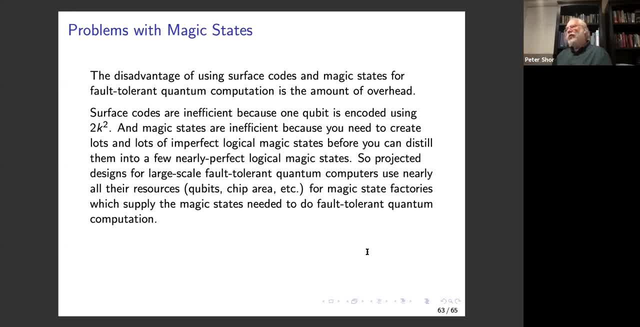 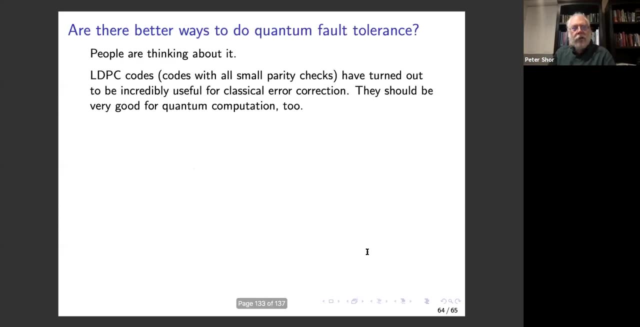 on your quantum computer, most of your resources are doing used for preparing these magic states, which is really seems like an incredible waste of resources, And if there was some way to do better than that, it would be great. Okay, So well, I have two slides on possible ways. 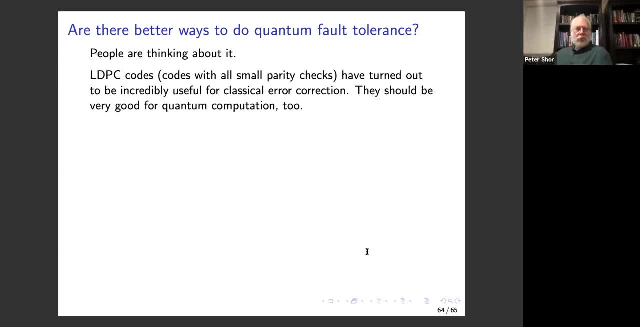 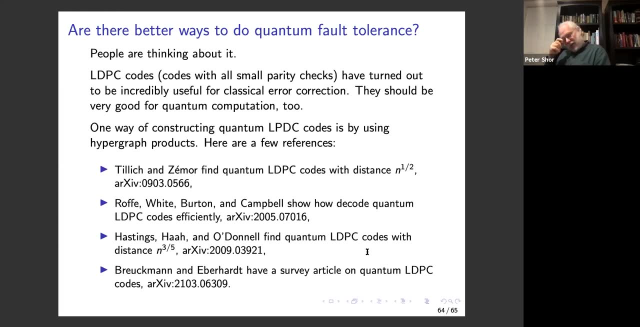 to you know, proceed without magic states. One of them is LDPC codes, LPDC codes, And these are codes with small parity checks. So the surface code is one of them, But there are other ones And one way of constructing these. 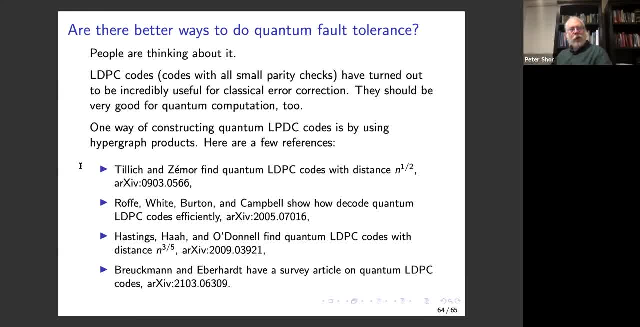 is using hypergraph products, And hypergraph products are a completely different way of constructing LDPC codes, And we haven't figured out how to use hypergraphic products to do quantum computation well yet, But we can. But maybe we can. And the other construction is related. 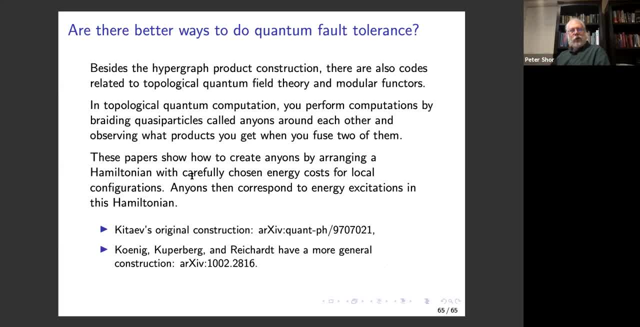 to topological quantum computation. So in topological quantum computation you have computations where you braid quasi-particles, called anions, around each other and observe what products you get when you fuse two of them, And you can create a Hamiltonian which you can simulate by qubits on a grid which has 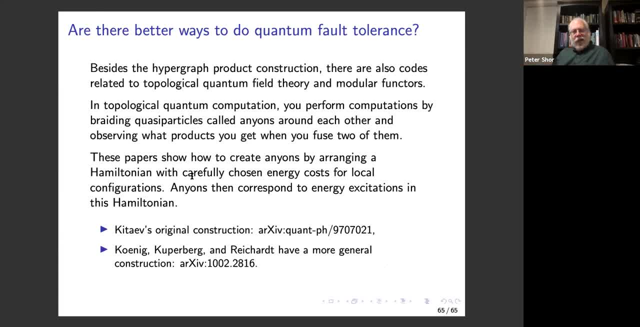 as anions, as its energy excitations. So that means you can actually do topological quantum computation using quantum codes And this might be another way to get around surface codes. And I think that's all I, and this is my last slide. 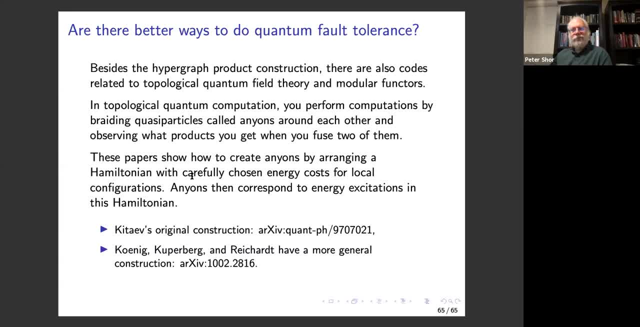 so I should open it up for questions. Thank you very much for the beautiful talk, And here are some questions. One is from Jin Chengu, And you mentioned that the current best size we have is about 60 qubits. What's the crux to build a large quantum computer? 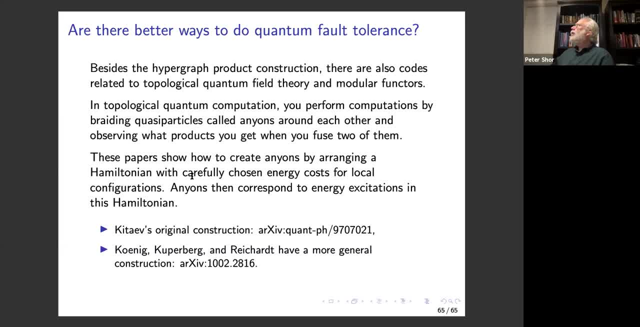 What's the problem for building a large quantum computer? Well, well, first people are going to: I mean so, I guess Google tried to build. I mean so, Google did this supremacy computation with a 53 qubit machine and actually they built a 54 qubit chip. 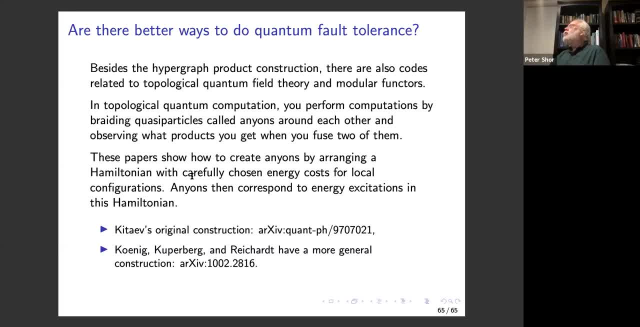 but one of the qubits didn't work right, So you really need a lot more experimental precision when you're constructing quantum bits to build a chip with thousands of qubits. The other thing is that right now, the qubits we have on large chips are really not very reliable. 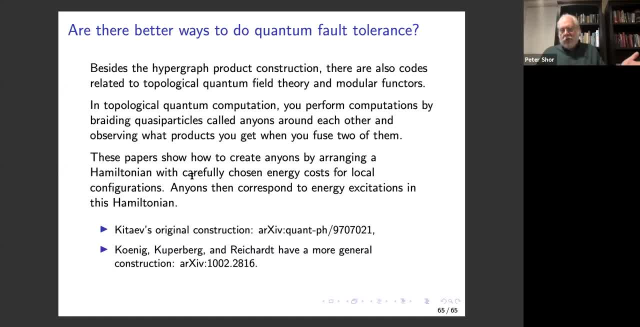 So maybe you know the gates are 99% accurate or 99.5% accurate. Well, that means if you do length 200 computation, there's a 50% probability that one of your qubits has done something wrong. 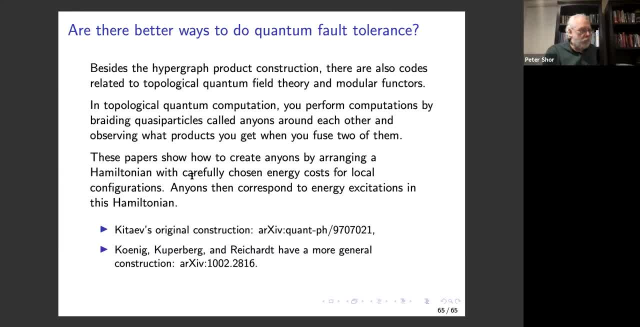 which means that the results aren't going to work. So if you have qubits that are only 99% accurate, there's no point in trying to build a chip with a thousand of them, because by the time you've applied the gate to every single qubit. 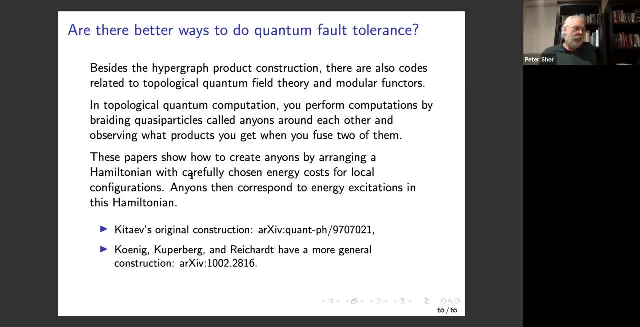 you've made an error and the results of your computation are unreliable. So you really need much better quantum gates and much better manufacturing techniques before you can build large computer chips. On the other hand, there are academic, experimental physicists who have built quantum gates or built chips with two qubits on them. 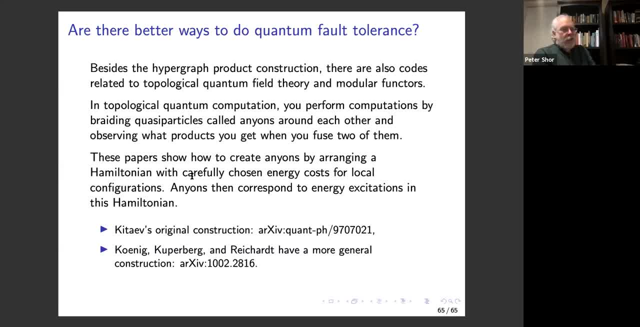 which have much higher accuracies than 99 percent. So it's possible. It's just combining the scaling and the accuracy, and everything is really something which we haven't figured out how to do yet. But if you believe there is a Moore's law for qubits, then we shouldn't be more than 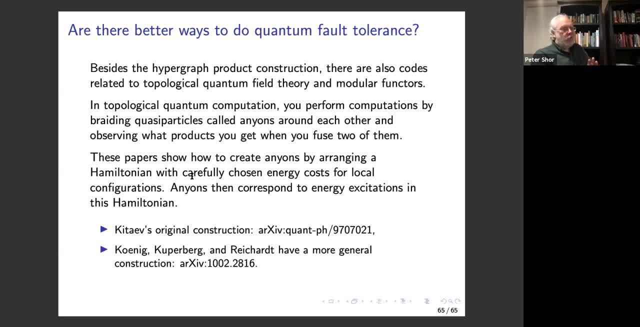 20 or 30 years before we have very large-scale quantum computers that work? And here's a question from Yixuan Wang: Why do we work with the stabilizers being a tensor product of non-trivial operators supported on a single site instead of more general form? Is this because 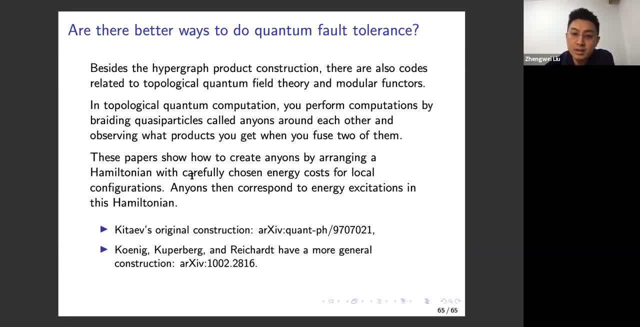 all general stabilizer codes are equivalent to the stabilizers of this type, up to a global unitary transformation, or just because such stabilizers are both within reach of theory and experimental realizations. Well, so the, I guess these anions and topological quantum computation, they're actually not the. 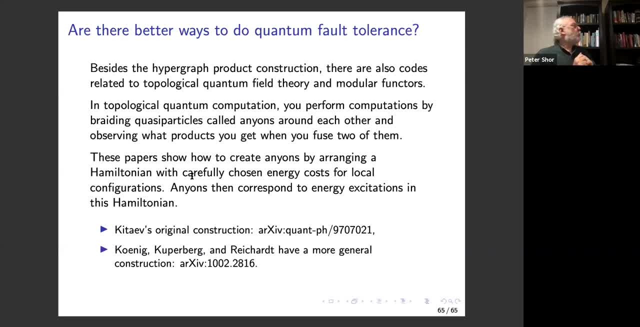 Pauli matrices. that are the basic building blocks, but more complicated things. But these codes are much more complicated to think about And really I think all the ones that have been designed so far are actually more complicated than the stabilizer codes. So stabilizer codes are both easy to think about and are probably better than the non-stabilizer, than. 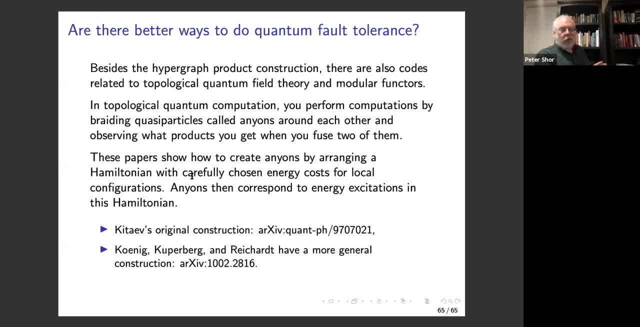 the more complicated ones we know about, So that's why we're using them. A question from Jintai Ding: How do those quantum-variable correcting codes are used practically? Yeah, Um, how are they used practically? Well, they're not yet. 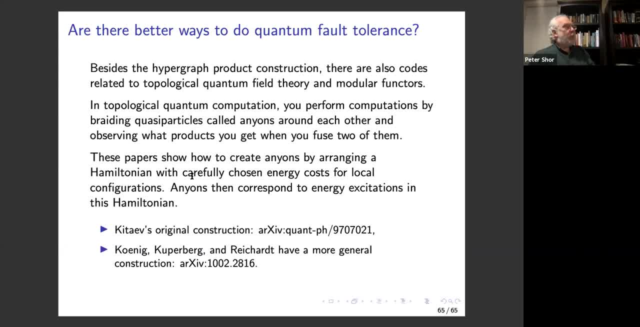 Um, but they would. I mean if we ever get large okay. So there's two things. If we ever get large scale quantum computers, we're going to have to use fault tolerance, And the only way we do know how to do fault tolerance is 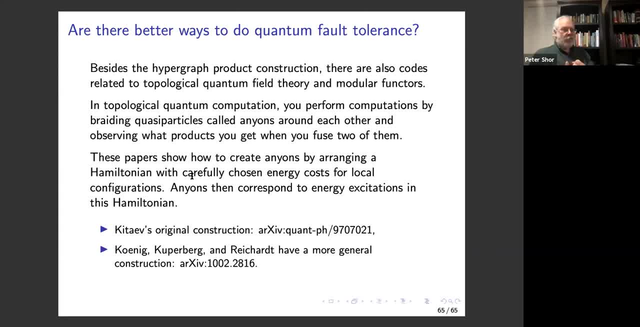 quantum error correcting code. And there's another thing. There's something called quantum key distribution, where two people with a quantum channel between them can agree on a key which an eavesdropper is guaranteed cannot be um Discover. it cannot be discovered by an eavesdropper. 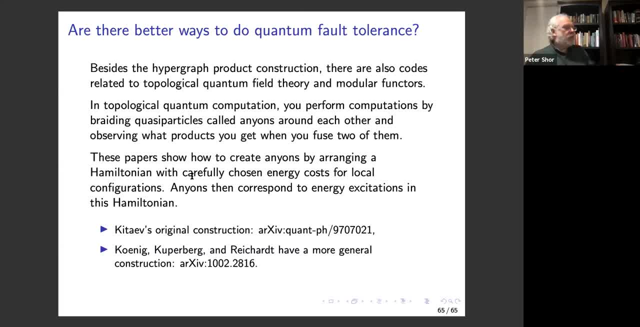 by the laws of physics and not just by the assumption that some computation is hard and the way the proofs that the security of quantum key distribution work, many of them go through quantum error correcting codes. and the third thing Is it's entirely possible that you could view build X physics experiments for 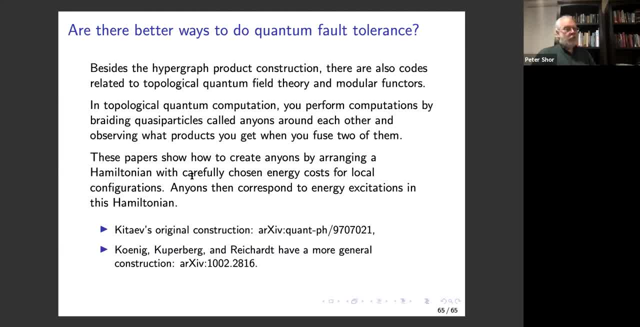 measuring things better than you could Um otherwise, by using quantum error correcting codes. for example, the best um The best quantum clocks are best clocks We know about. use something that's equivalent to the um Repetition code in them. 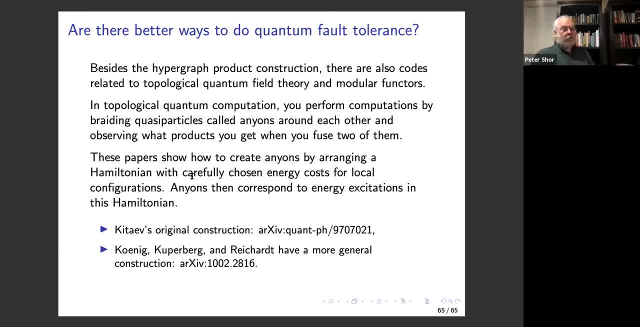 And it's entirely possible that we could build better clocks using quantum error correcting codes, um, in their design, Although I don't know if anybody has actually proposed a protocol for it, but it's seems conceivable. Uh, we have several questions. 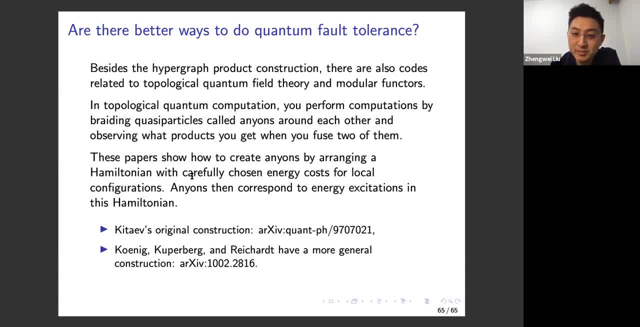 Still, uh, which experimental system is most promising? Well, the ones that are the most promising so far are using ion traps and using trans mons with superconducting chips. And these are, you know, these are two quantum systems which both have fairly. 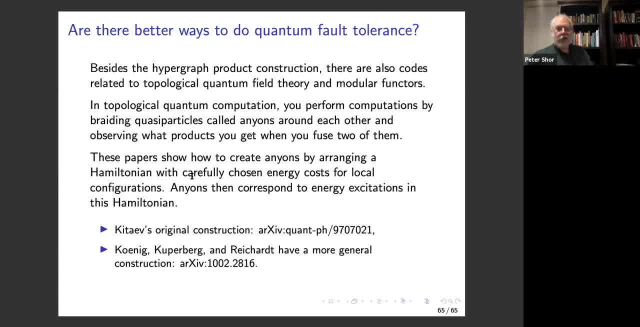 large numbers of qubits And reasonably good accuracy. I mean, the disadvantage of ion traps is that they're much slower than trans mons, So if you wanted to do a long computation on them, so breaking codes, it might take days instead of um hours. and the disadvantage of the advantage of ion traps is it looks. 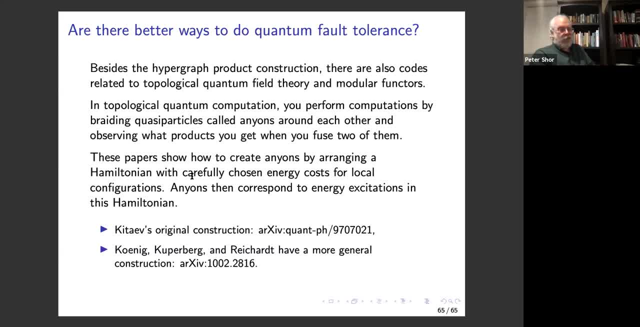 like they're going to be much more accurate gates. Then We can do on superconducting code qubits in the near future, So they have an advantage that way. So I'm not going to be able to decide between these two things. 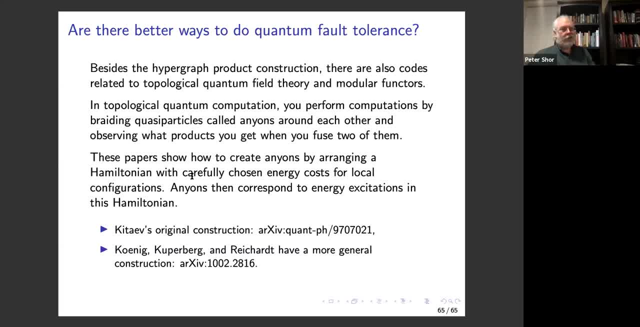 And then there are also other people investigating completely different techniques, like one of dots and other stuff, And I don't know, I mean I don't know that they're not going to be able to come up with some very clever way and surpass ion traps and trans mons. 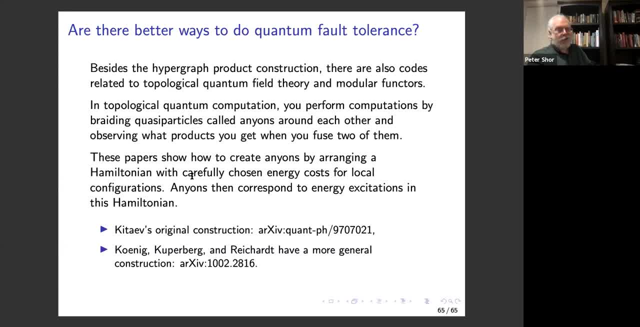 right now, but right now they're far behind these two technologies. do we know the minimal cost of quantum iron cracking codes? no, we, i mean. so it looks very much like if you want to do computation with accuracy with gates that are accurate in one part in n. no, it looks very much like if you want to do. 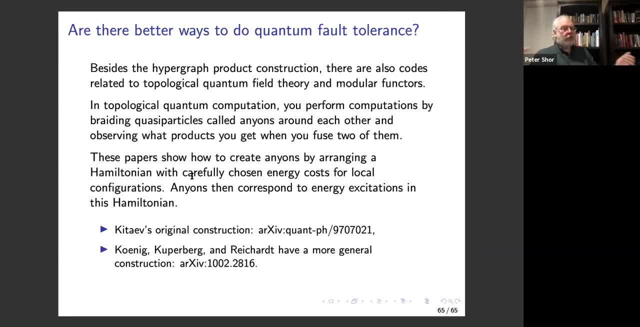 n steps of computation, you need at least log n overhead. but the best techniques we have for proving that right now are log squared n overhead and we have very, very bad, lower bounds on the how much overhead you really need for fault-tolerant quantum computation. so we don't have any idea about. 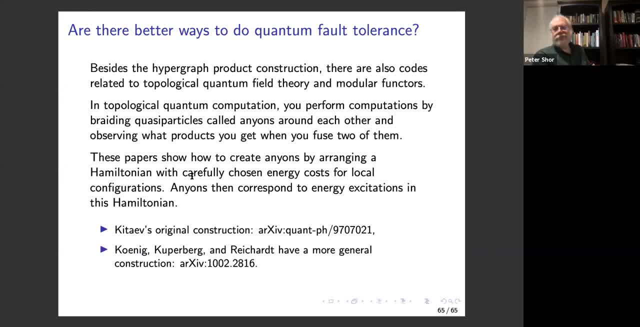 lower bounds? with all these quantum iron cracking codes adding up to the complexity, is it still realistic for quantum computers to exceed the classic ones? um well, i mean, if you get, if you get a computer with billion quantum bits which has um one part in 10 to the fourth accuracy for each quantum gate. 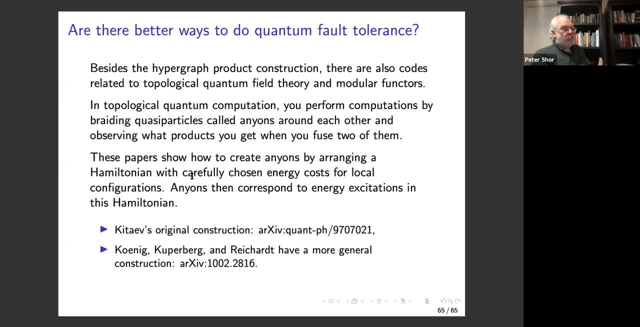 then you can definitely use quantum, these quantum error tracking codes, to do computations you could never do on a classical computer. and you know a billion qubits and um. one part intended, the one part in 10 to the fourth, are really completely trivial um, you know numbers for classical computers. 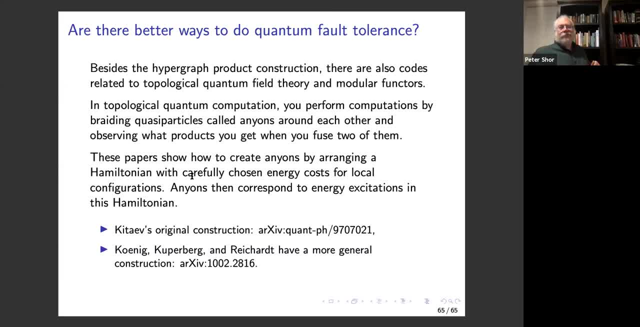 so there's definitely hope. and what do you think is the relationship between quantum b algebra and quantum christography? can connection be constructed between quantum error correcting codes and other algebra, a logical algebra, um? well, quantum error correcting codes using quantum, using anions, and quantum topological field theory are very much connected with um. 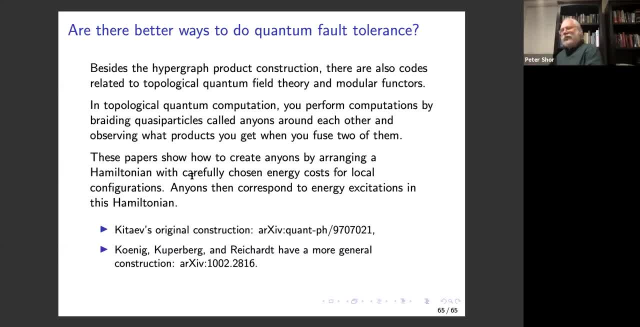 modular functors, which are an algebraic construction. so there is some kind of close connection between um quantum error correction and algebra. and the other thing is that algebraic geometry codes are, you know, very good classical codes and no, we can use algebraic classical codes generated. 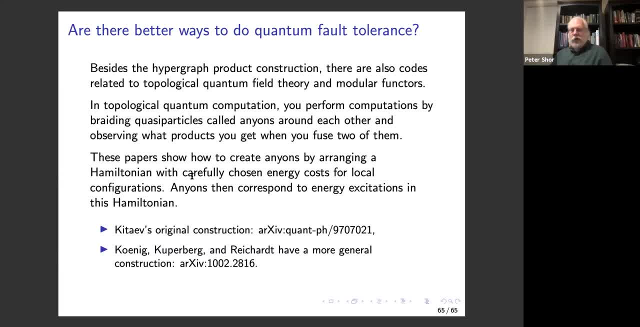 by algebraic geometry to get quantum codes with a css code construction or a stabilizer code construction. so these are also um connection between algebra and quantum error correction. now then, i believe in topological. any small fault tolerance than a billion ones, um so well, the the real advantage of non-abelian anions rather than billion anions. 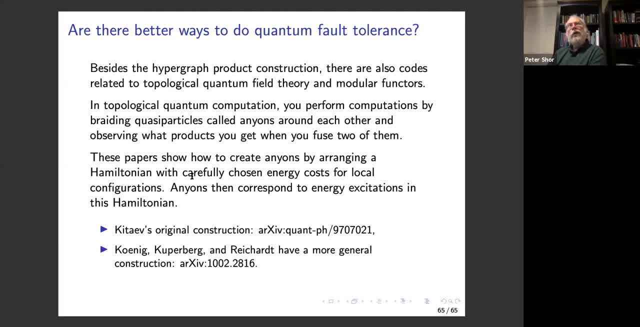 is that non-abelian anions. you can do computations with them directly on the anion. so if you braid one anion around another, this does a quantum gate on the underlying hilbert space. and if you have a billion anions and you braid one around each other, this 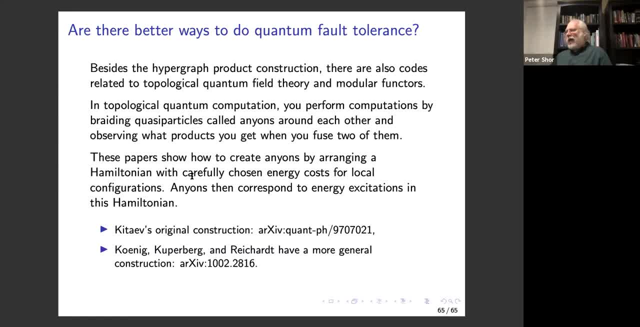 quantum gate is just multiplies by. it's just basically multiplication by a complex phase. so you're never going to get anywhere into any interesting computations just by doing those um quantum gates. but if you have, say, the eisen set of anions and you braid one around, 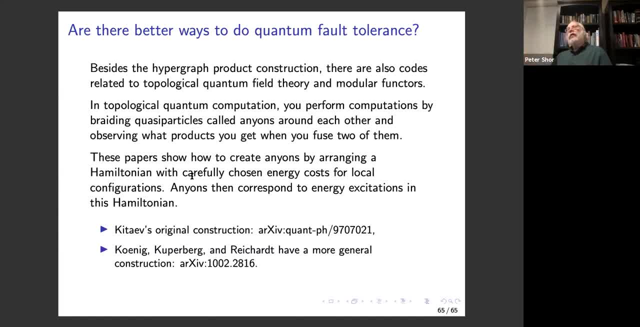 the other um, it does a non-trivial thing to your um underlying quantum state. so if you have a complicated enough set of anions, then you can definitely do quantum computation just by braiding the anions around each other, and that means you don't have to come up with a set of anions. 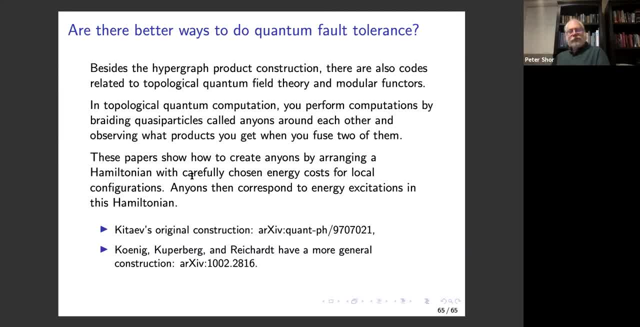 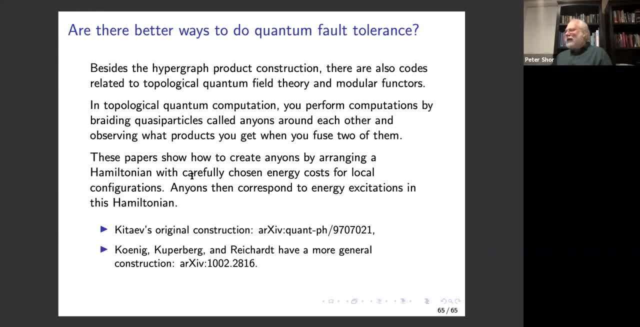 you know, there are studies saying if you have a quantum gate that can factor rsa 1024, you know a quantum computer that can do. you know a quantum computer that can do. you know a quantum computer that can do x million operations, and it has x million operations and it has. 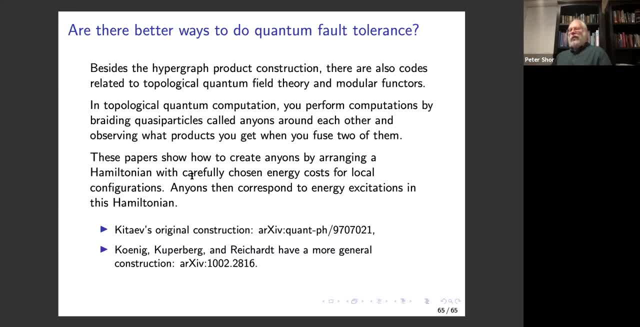 x million operations and it has y million quantum bits, y million quantum bits, y million quantum bits, and it and it, and it has each operation accurate. to has each operation accurate to has each operation accurate to one part in x, then you can factor rsa, one part in x, then you can factor rsa. 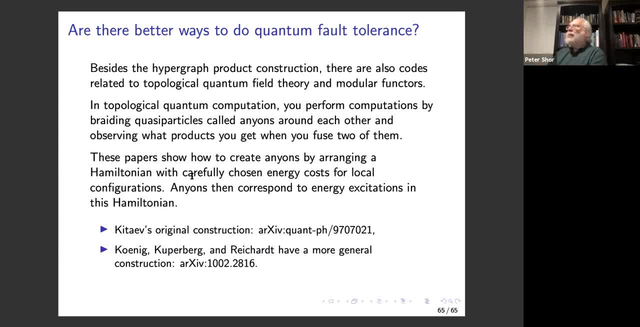 one part in x, then you can factor rsa and you can look up these, and you can look up these, and you can look up these um papers on the archive, um papers on the archive, um papers on the archive. but i don't have the numbers memorized. 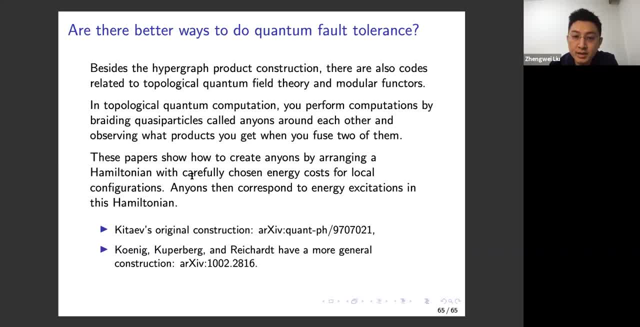 but i don't have the numbers memorized. but i don't have the numbers memorized. the theory of fault tolerant quantum. the theory of fault tolerant quantum. the theory of fault tolerant quantum. computation: computation: computation is based on the idealization of the is based on the idealization of the. 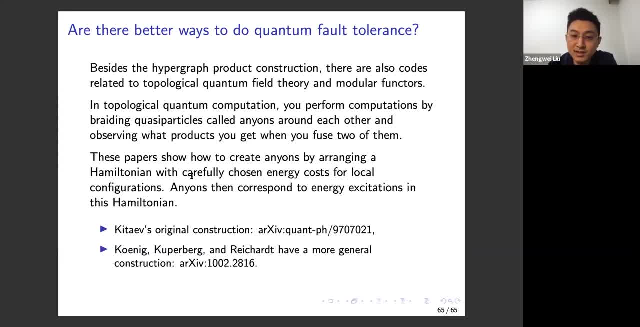 is based on the idealization of the physical world. physical world, physical world that looks unrealistic to a condensed. that looks unrealistic to a condensed. that looks unrealistic to a condensed. matter matter, matter. theorists like superior, such that theorists like superior, such that theorists like superior, such that and kept qv system. 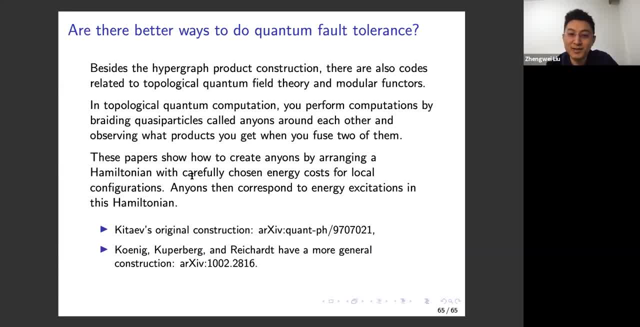 and kept qv system. and kept qv system coupled to random heat bias with coupled to random heat bias with coupled to random heat bias with uncorrelated random errors in practice. uncorrelated random errors in practice. uncorrelated random errors in practice. qvs are coupled to numerous 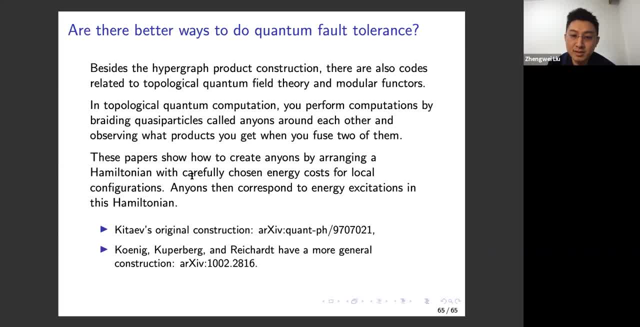 qvs are coupled to numerous qvs are coupled to numerous gapless elements with an experimental gapless elements, with an experimental gapless elements, with an experimental large, large, large hyperspace of interacting degrees of hyperspace, of interacting degrees of hyperspace, of interacting degrees of freedom. 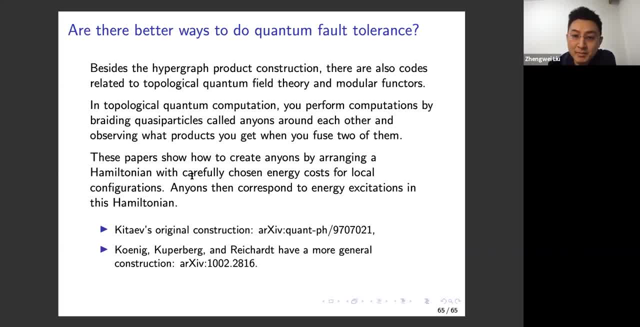 freedom. freedom: the small arrows get very quickly. the small arrows get very quickly. the small arrows get very quickly, magnified by many body quantum kills. magnified by many body quantum kills. magnified by many body quantum kills, and are not uncorrelated between qvs, and are not uncorrelated between qvs. 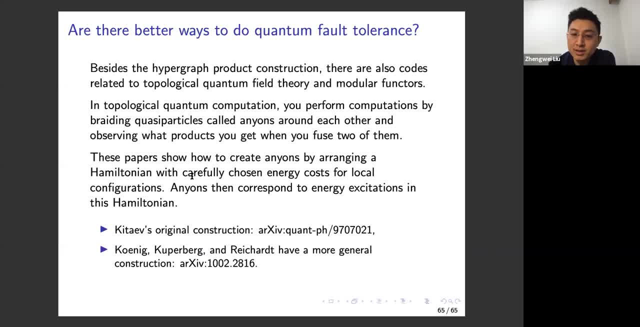 and are not uncorrelated between qvs. so what are your thoughts on making the? so what are your thoughts on making the? so what are your thoughts on making the series more realistic series more realistic series more realistic? well, i mean so if you look at classical. 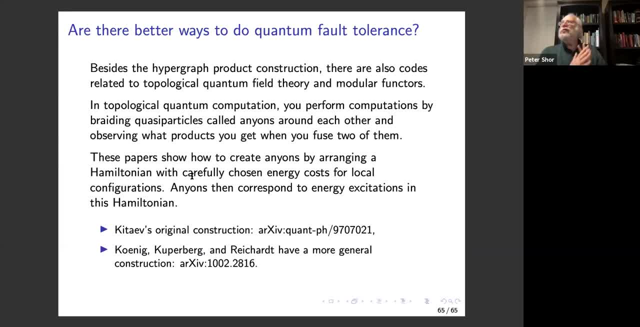 well, i mean so if you look at classical- well, i mean so if you look at classical. error correction on error correction on error correction on classical computers, we assume that classical computers, we assume that classical computers, we assume that everything is, everything, is everything is independent or nearly independent, and 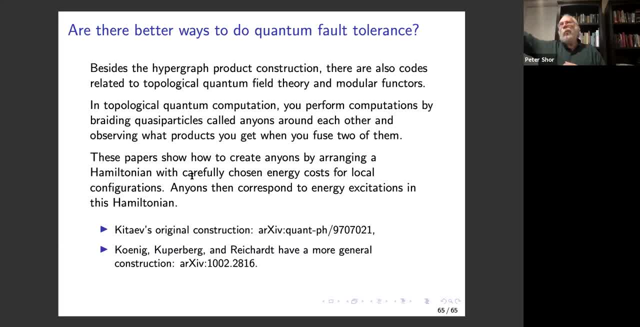 independent or nearly independent and independent or nearly independent. and you know in the real world if you have. you know in the real world if you have. you know in the real world, if you have um uh cell phone tower and um uh cell phone tower and um uh cell phone tower and uh cell phone receiver and the cell 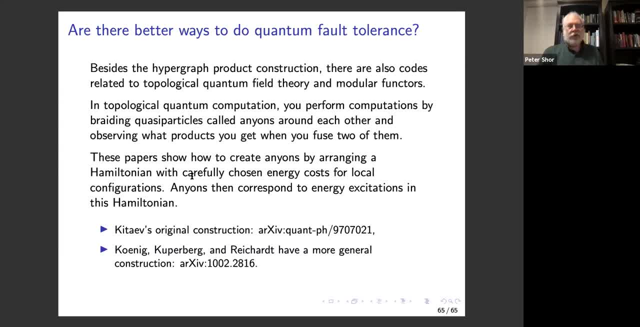 uh cell phone receiver and the cell? uh cell phone receiver and the cell phone tower goes. phone tower goes. phone tower goes, you know, sends a signal to the cell phone, you know, sends a signal to the cell phone receiver, receiver, receiver. nothing is independent but the fact that 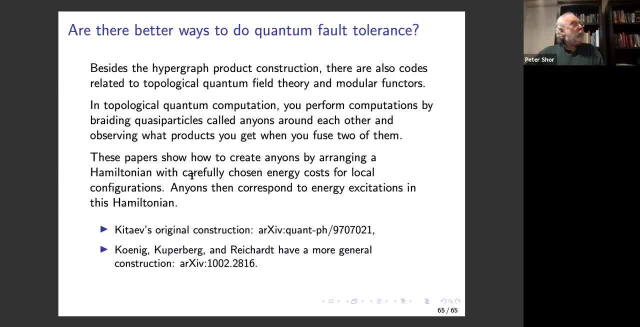 nothing is independent. but the fact that nothing is independent, but the fact that there is correlations doesn't matter. there is correlations doesn't matter, there is correlations doesn't matter because these correlations are not, because these correlations are not, because these correlations are not designed adversarily in order to defeat. 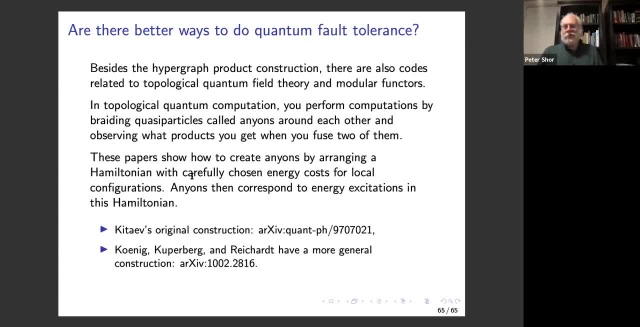 designed adversarily in order to defeat, designed adversarily in order to defeat your classical codes, your classical codes, your classical codes. now there's lots of correlations in now. there's lots of correlations in. now. there's lots of correlations in. you know a real condensed matter. you know a real condensed matter. 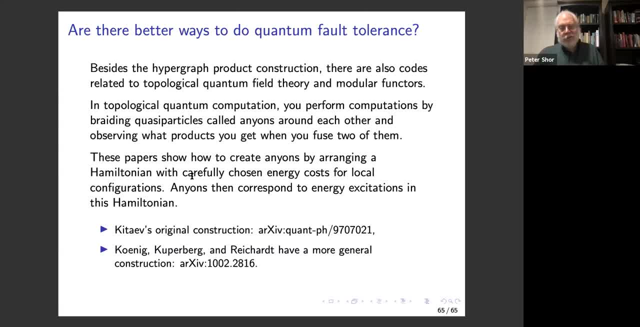 you know, a real condensed matter, system, system, system, but, but. but they're all fairly small, they're all fairly small, they're all fairly small. and the adversary and the adversary and the adversary: no adversary has defined, designed them. no adversary has defined. designed them no adversary has defined, designed them maliciously so as to defeat your. 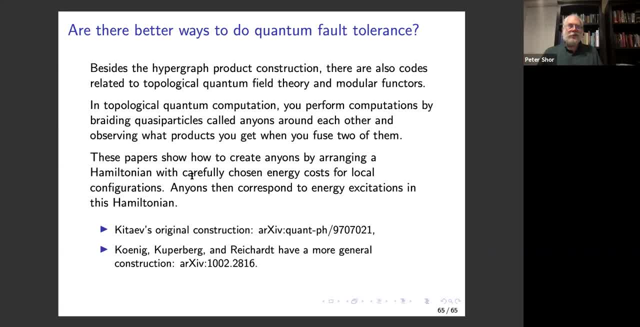 maliciously so as to defeat your, maliciously so as to defeat your- quantum error correcting codes. so my quantum error correcting codes, so my quantum error correcting codes. so my hope is that hope is that hope is that it doesn't matter that they're correlated. it doesn't matter that they're correlated. 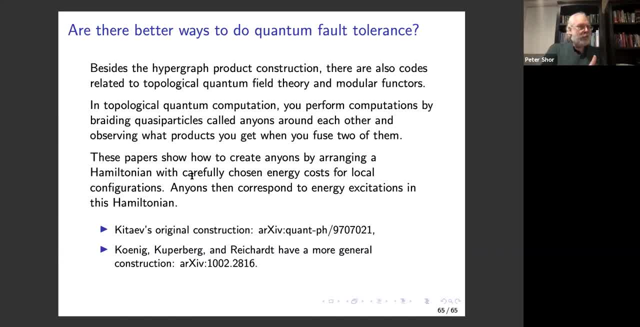 it doesn't matter that they're correlated and they're not correlated in any way, and they're not correlated in any way and they're not correlated in any way. that is going to affect that is going to affect that is going to affect the error correction. the error correction. 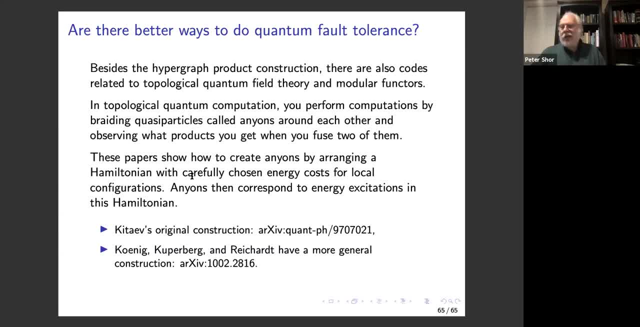 the error correction, but i mean we can't prove this. but i mean we can't prove this, but i mean we can't prove this without actually um, without actually um, without actually um either having an extremely, either having an extremely, either having an extremely complicated model of errors. 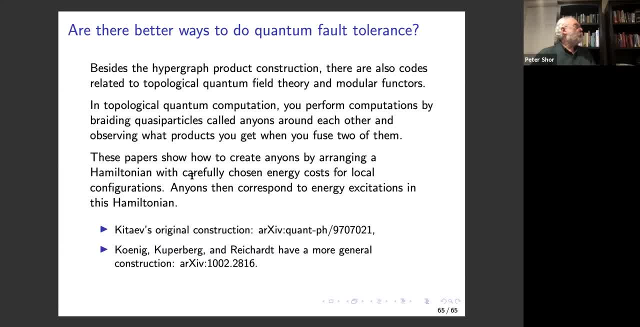 complicated model of errors, complicated model of errors which it's very difficult to actually, which it's very difficult to actually, which it's very difficult to actually prove anything about. prove anything about, prove anything about, or by designing a system and seeing that, or by designing a system and seeing that. 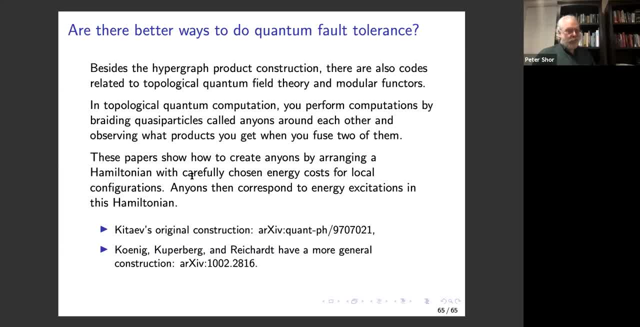 or by designing a system and seeing that it works, it works, it works. so i think that you know this fact that. so i think that you know this fact that. so i think that you know this fact that errors are really correlated, errors are really correlated, errors are really correlated, is not going to matter at all in terms. 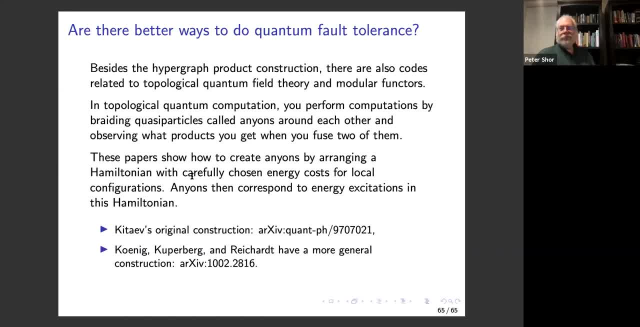 is not going to matter at all in terms. is not going to matter at all in terms of of of actually building them. how good is bisonic code compared with? how good is bisonic code compared with? how good is bisonic code compared with stabilizer code? 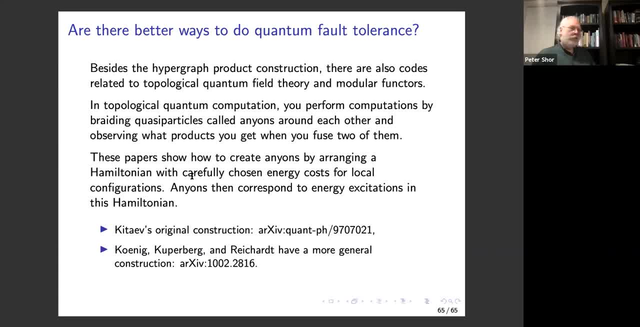 um, um, um, well, i mean, there's lots of different. well, i mean there's lots of different. well, i mean, there's lots of different. um metrics for good, um, um metrics for good, um, um metrics for good, um. the ldpc codes are good. the ldpc codes are good. 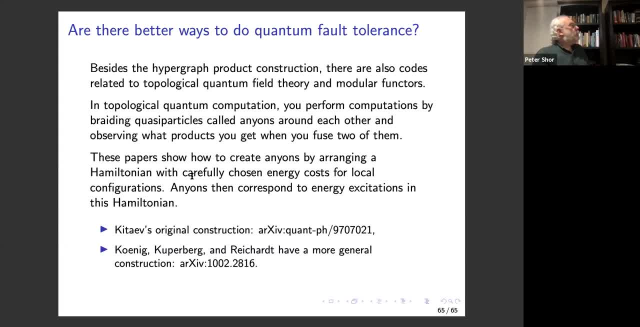 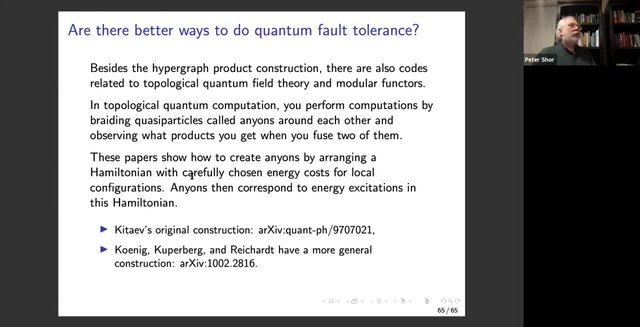 are much broader than surface codes, are much broader than surface codes, which is what we're thinking of using, which is what we're thinking of using, which is what we're thinking of using, and it's quite possible, we will find. and it's quite possible, we will find. 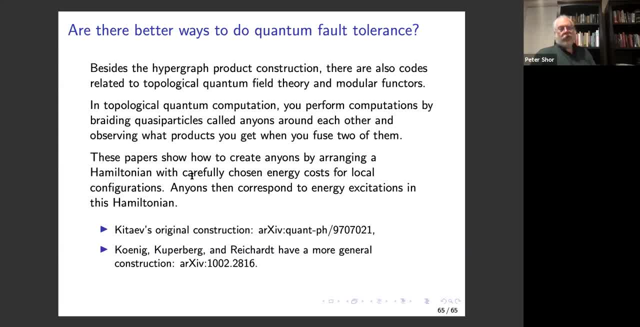 and it's quite possible, we will find much better stabilizer codes for much better stabilizer codes for much better stabilizer codes for correcting errors, correcting errors, correcting errors, than the surface codes we know about now, than the surface codes we know about now, than the surface codes we know about now. we. 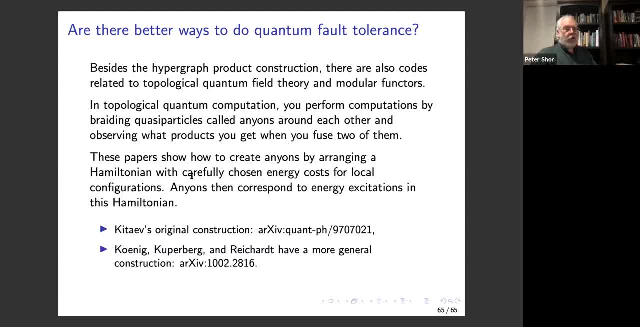 we, we know, know, know barely anything about exotic codes. so barely anything about exotic codes. so barely anything about exotic codes. so, um, um, um. it's not clear at all that there are. it's not clear at all that there are. it's not clear at all that there are going to be. 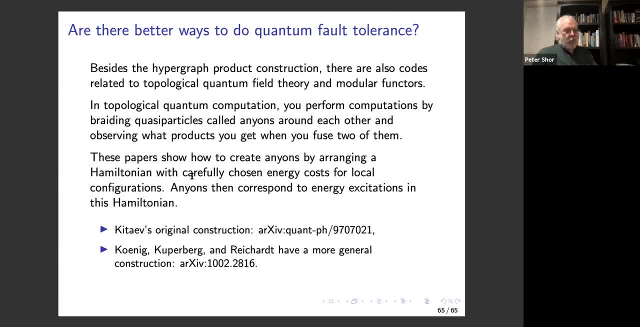 going to be going to be useful exotic codes to use, for useful exotic codes to use, for useful exotic codes to use for fault tolerance, but fault tolerance but fault tolerance. but there are certainly stabilizer codes, there are certainly stabilizer codes, there are certainly stabilizer codes that are not surface codes and that 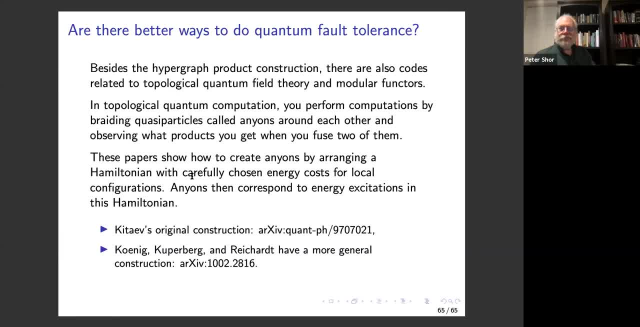 that are not surface codes and that that are not surface codes and that might be, might be, might be very useful for both. tolerance: what will be earlier in your opinion? what will be earlier in your opinion? what will be earlier in your opinion? quantum computer doing fast. quantum computer doing fast. 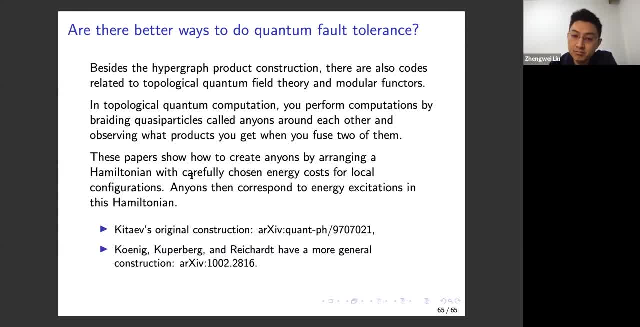 quantum computer doing fast. shaw algorithm factorization. shaw algorithm factorization. shaw algorithm factorization. say, say, say, 250 dgs numbers, 250 dgs numbers, 250 dgs numbers. all a new discovery in number theory. all a new discovery in number theory. 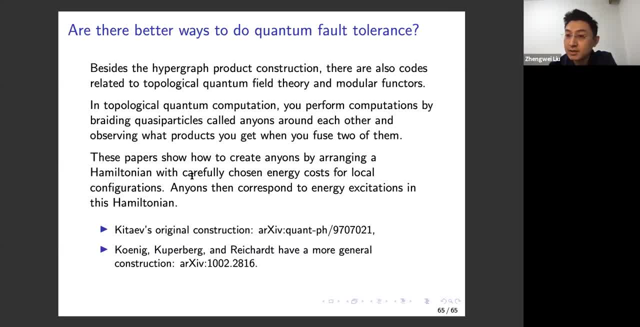 all a new discovery in number theory of fast classical factorization, of fast classical factorization, of fast classical factorization algorithm, algorithm, algorithm. um well, i mean we've, i mean we've, i mean, we've, i mean, it's been a long time since. i mean, it's been a long time since. 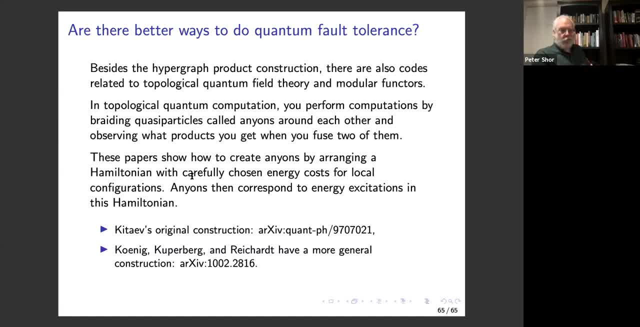 i mean, it's been a long time since there's a, there's a, there's a new, but that, since there's been a new, new, but that, since there's been a new, new, but that, since there's been a new fast factorization algorithm, the number 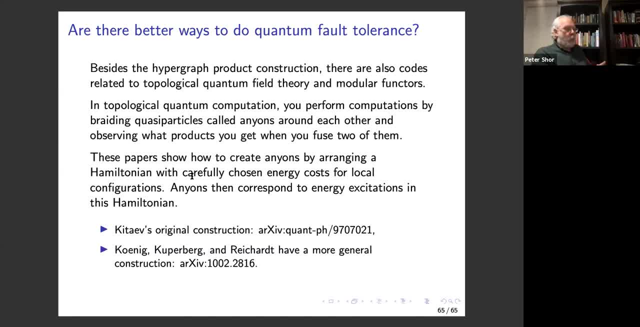 fast factorization algorithm, the number fast factorization algorithm, the number theory theory theory, and um i mean, and um i mean, and um i mean. it's been a long time since there's a new. it's been a long time since there's a new. it's been a long time since there's a new. it's quite possible someone could come. 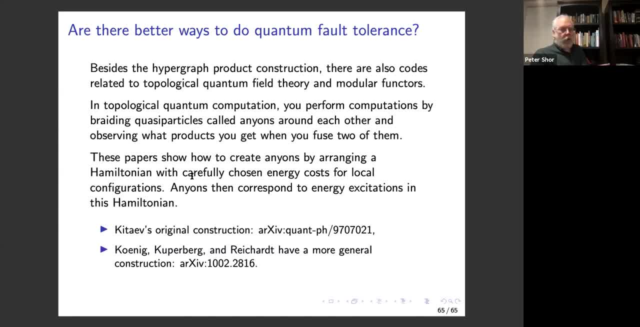 it's quite possible, someone could come. it's quite possible someone could come up with a polynomial time algorithm, up with a polynomial time algorithm, up with a polynomial time algorithm for factorization tomorrow. but it's also for factorization tomorrow, but it's also for factorization tomorrow. but it's also quite possible that such a thing doesn't. 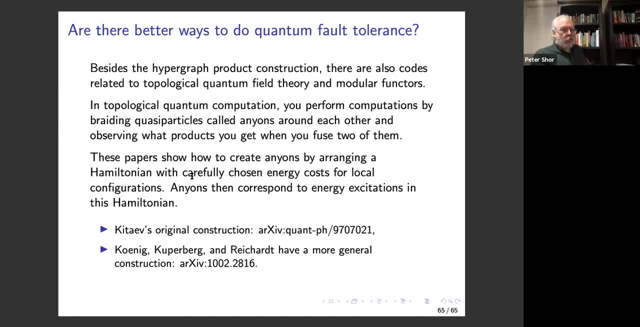 quite possible that such a thing doesn't quite possible, that such a thing doesn't exist, and we already know exist, and we already know exist, and we already know all the good algorithms for factoring, all the good algorithms for factoring, all the good algorithms for factoring 250 digit numbers. 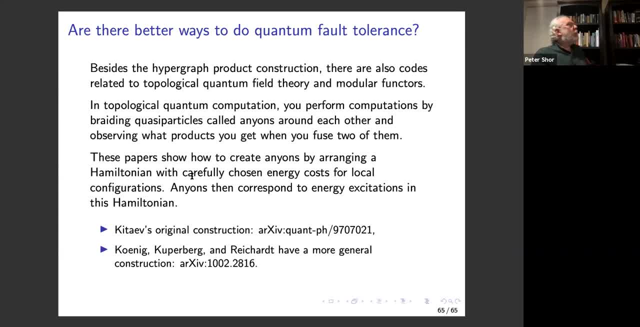 250 digit numbers, 250 digit numbers. so which is more likely? i don't know. do we need uh millions of qubits to do? we need uh millions of qubits to do. we need uh millions of qubits to realize quantum error corrections. realize quantum error corrections. 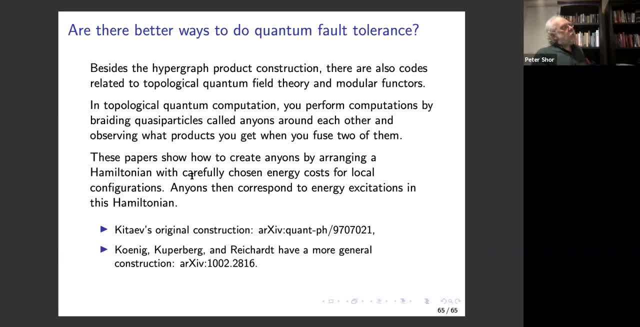 realize quantum error corrections: um, um, um. well. if you want to do quantum error, well. if you want to do quantum error, well. if you want to do quantum error correction, correction, correction on uh. if you want to do a computation on uh, if you want to do a computation. 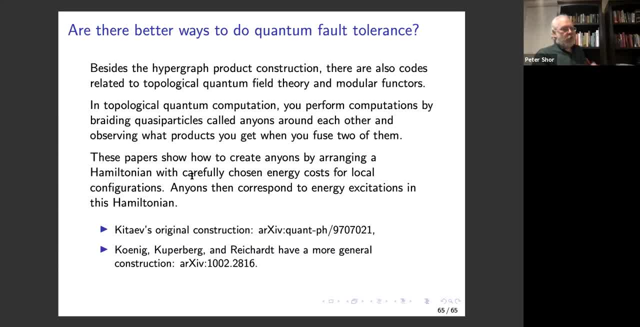 on. uh, if you want to do a computation with several thousand qubits, with several thousand qubits, with several thousand qubits, and do quantum error correction and do quantum error correction and do quantum error correction on it, then you probably on it, then you probably on it, then you probably then using the techniques we do, we know. 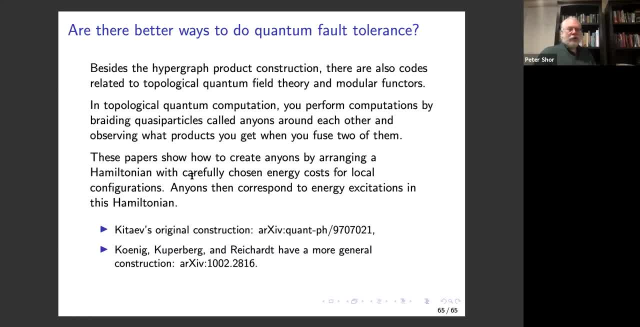 then using the techniques we do we know, then using the techniques we do we know about you probably do need a million, about you probably do need a million, about you probably do need a million qubits, qubits, qubits. but first, but first, but first, um, quantum error correction, where the 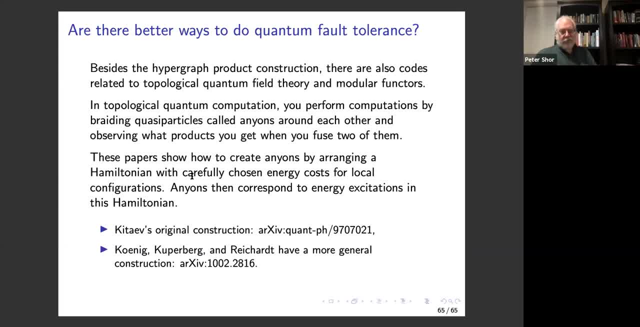 um quantum error correction, where the um quantum error correction, where the overhead is overhead is overhead is 10 then rather than 100, 10 then rather than 100, 10 then rather than 100 um in the next 10 years. it's much more um in the next 10 years. it's much more. 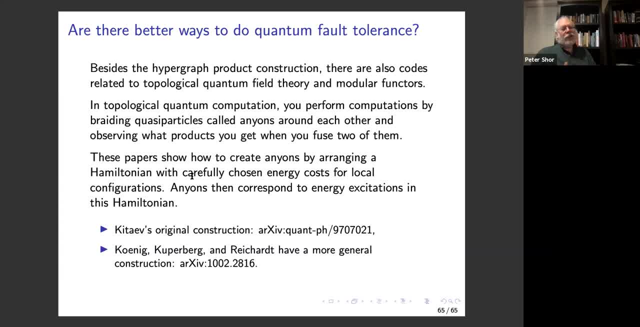 um, in the next 10 years, it's much more likely than likely than likely than that that will happen. rather than that that will happen. rather than that that will happen. rather than someone finding someone finding someone finding uh better classical factoring algorithm- uh better classical factoring algorithm. 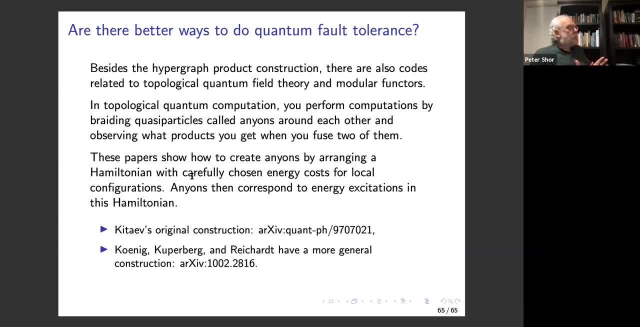 uh, better classical factoring algorithm. so i in fact, so, i think, so, i in fact, so, i think, so, i in fact, so, i think, and the other thing is, if you want to, and the other thing is, if you want to, and the other thing is, if you want to just demonstrate quantum error correction. 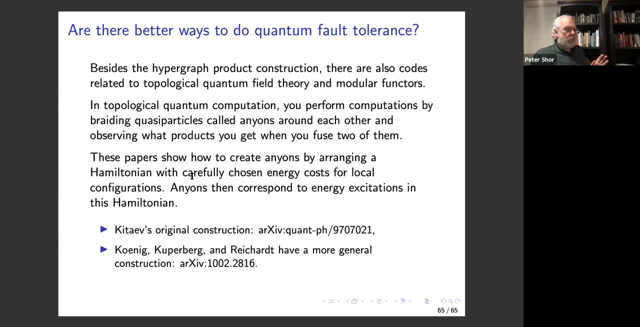 just demonstrate quantum error correction on three or four qubits. i think you on three or four qubits, i think you on three or four qubits. i think you could do it with, could do it with. could do it with a hundred um physical qubits. a hundred um physical qubits. 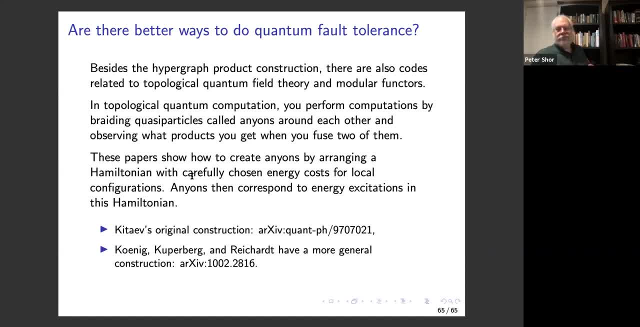 a hundred um physical qubits and um we're going to have that in the and um we're going to have that in the and um we're going to have that in the next few years, and whether there's still exponential. and whether there's still exponential. 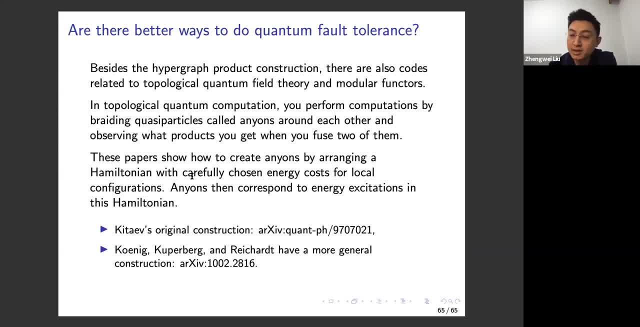 and whether there's still exponential speed up for quantum computer, speed up for quantum computer, speed up for quantum computer after we consider noise, after we consider noise, after we consider noise. um, well, if, well, if well, if, if we assume, if we assume, if we assume that that 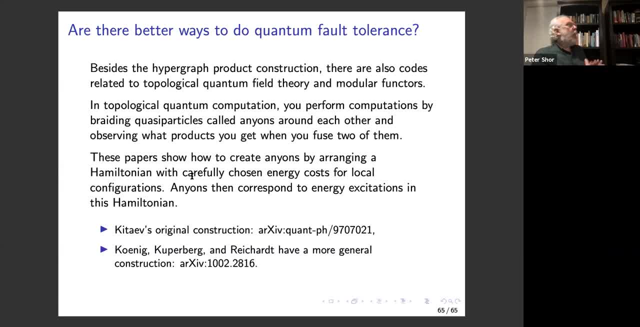 that the noise is independent. the noise is independent, the noise is independent. yes, there is, yes, there is, yes, there is. if we assume the noise, if we assume the noise, if we assume the noise is, is is not independent, not independent, not independent and is not maliciously controlled by. 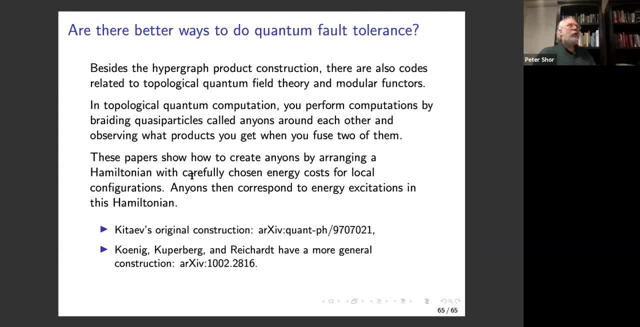 and is not maliciously controlled by, and is not maliciously controlled by some kind of adversary who's trying to some kind of adversary who's trying to some kind of adversary who's trying to defeat our computation, defeat our computation, defeat our computation. we don't have any proof that there is but. 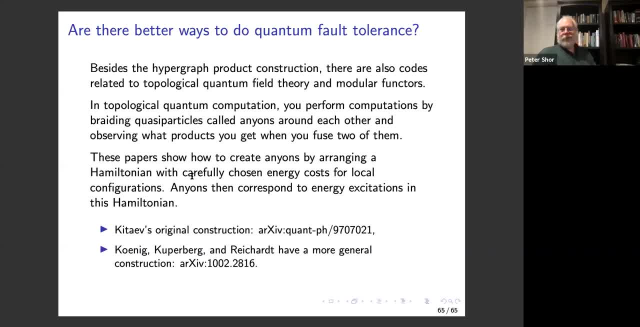 we don't have any proof that there is. but we don't have any proof that there is, but i think it's very, very likely. and classical codes have some other and classical codes have some other and classical codes have some other parameters of interest, like locality. parameters of interest like locality. 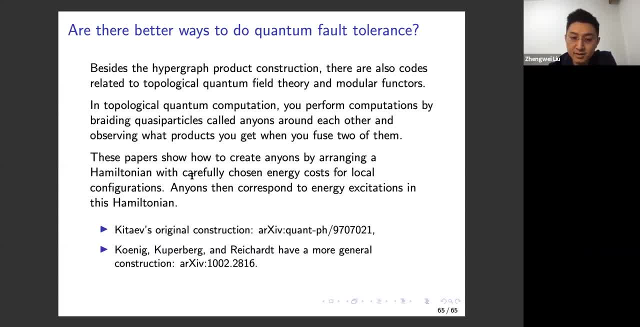 parameters of interest like locality, and are concepts like locality, even of, and are concepts like locality, even of and are concepts like locality even of interest or relevance in quantum error interest or relevance in quantum error, interest or relevance in quantum error corrections? yeah, so, locality is probably one of the 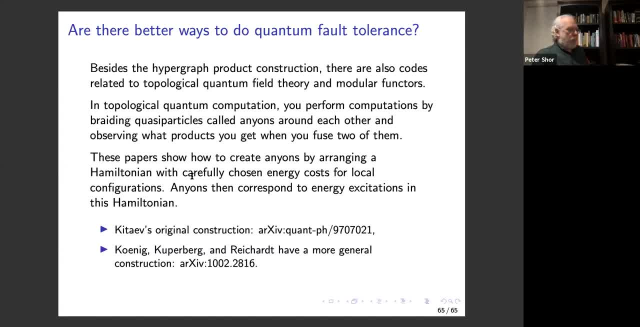 yeah, so locality is probably one of the yeah, so locality is probably one of the main reasons that people main reasons that people main reasons that people. you know planning to build um. you know planning to build um. you know planning to build um, you know, you know, you know quantum computers in the distant future. 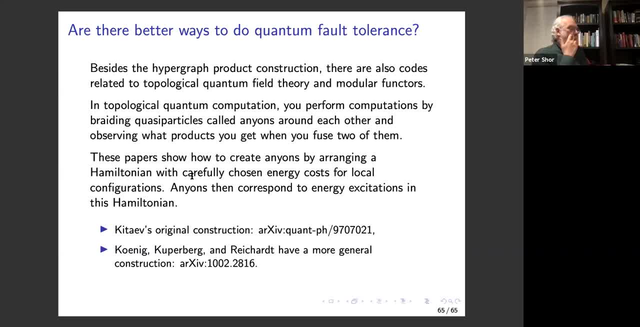 quantum computers in the distant future. quantum computers in the distant future are using surface codes rather than are using surface codes, rather than are using surface codes rather than um these, these, these hypergraph product codes, is locality. hypergraph product codes is locality. hypergraph product codes is locality, so locality is. 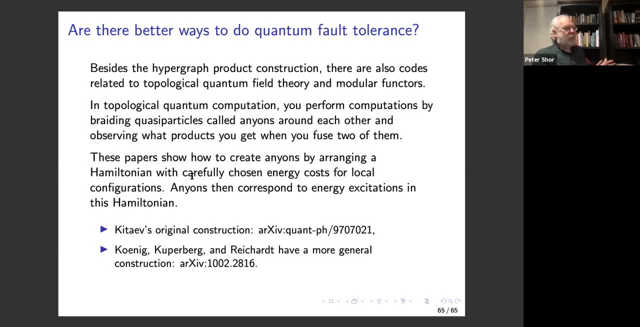 so locality is. so locality is very important for quantum codes and i very important for quantum codes and i very important for quantum codes, and i have basically swept that under the rug, have basically swept that under the rug, have basically swept that under the rug in my talk, but it's a 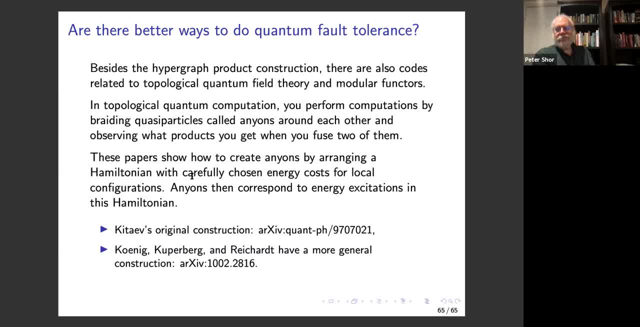 in my talk, but it's a in my talk, but it's a a very important consideration. yeah, a very important consideration. yeah, a very important consideration. yeah, have people thought about using machine? have people thought about using machine? have people thought about using machine learning, learning, learning to design better quantum error. 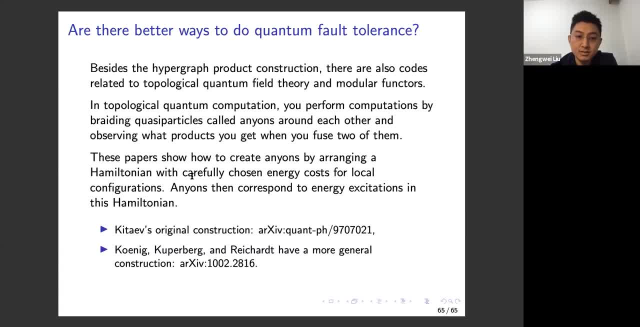 to design better quantum error, to design better quantum error. cracking codes. cracking codes. cracking codes, um, um, um. have any? have any? have any? have has machine learning designed? have has machine learning designed? have has machine learning designed any better? classical error: correcting any better classical error. correcting any better classical error. correcting codes. 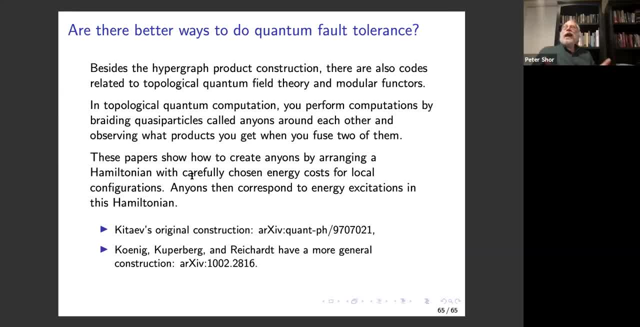 uh, quantum error correcting codes. uh, quantum error correcting codes. uh, quantum error correcting codes. no i, i'm asking: has machine learning? no, i, i'm asking: has machine learning? no, i, i'm asking: has machine learning designed any better? classical error designed any better? classical error designed any better? classical error correcting codes and. 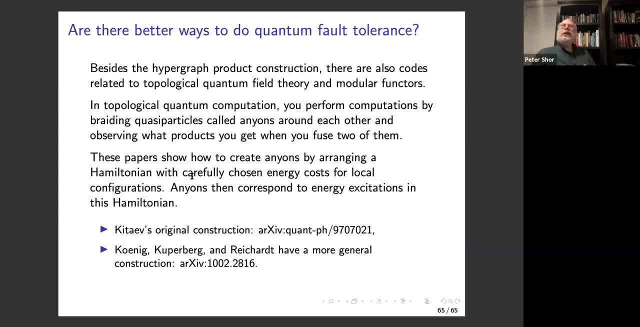 correcting codes and correcting codes, and the answer, i'm pretty sure, is no, so i the answer, i'm pretty sure, is no, so i the answer, i'm pretty sure, is no, so i don't see why we should expect it to. don't see why we should expect it to. 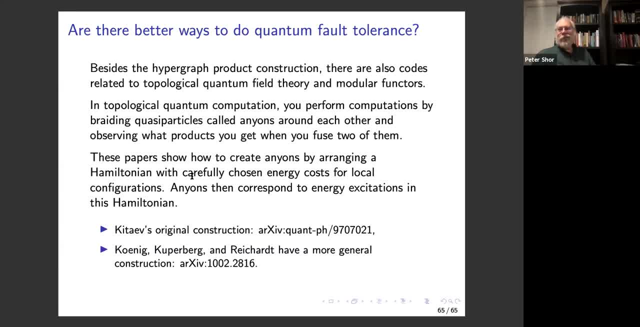 don't see why we should expect it to design better quantum error correcting design. better quantum error correcting design. better quantum error correcting codes, codes, codes. i mean machine learning actually. could i mean machine learning actually, could i mean machine learning actually could easily tweak parameters on classical, easily tweak parameters on classical. 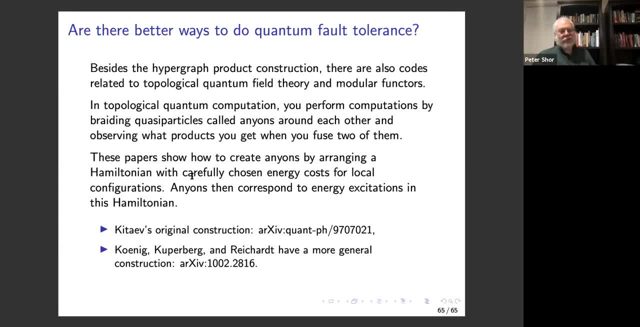 easily tweak parameters on classical error correcting codes, but actually error correcting codes, but actually error correcting codes, but actually designing a new class of them, i think is designing a new class of them. i think is designing a new class of them, i think is hopelessly out of. 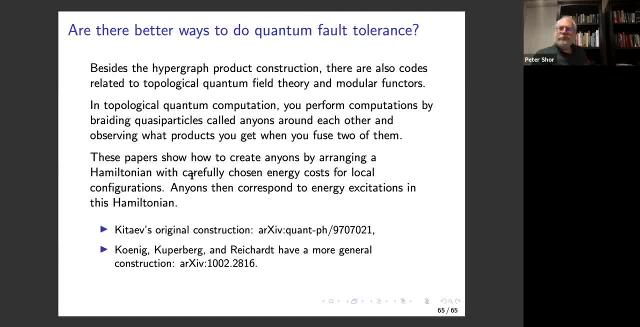 hopelessly out of, hopelessly out of its abilities. how could it attack the? how could it attack the? how could it attack the control noise, um, um, um. i need. I mean there are no real attackers, for I mean the attacker that we're imagining is controlling the noise is nature, and nature is not malicious, just random. so I don't think an attacker is going. 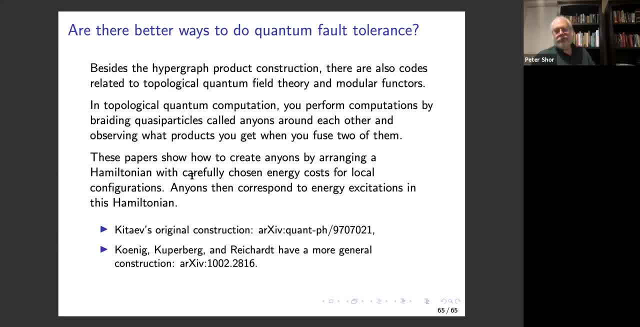 to control noise, to defeat quantum computers? how did you find the factoring algorithm? how did I find the factoring algorithm? well, I would say, watch my May 6th talk, at the 40th anniversary of the quantum. you know the the physics and computation conference at Endicott. 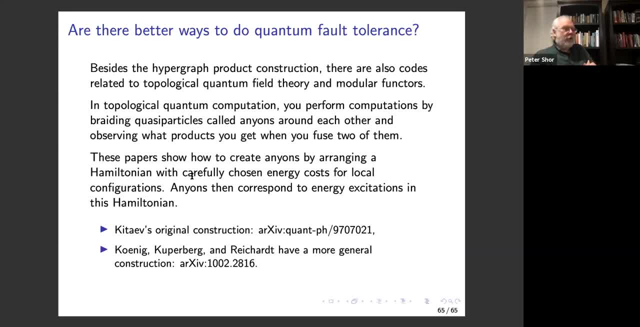 house on May 6th. but how did I find it? well, essentially I saw Dan Simon's algorithm- for you know, I'm solving this contrived problem on binary strings and a function on binary strings, and I generalized it to an algorithm that solved discrete logs and factoring and the basic.